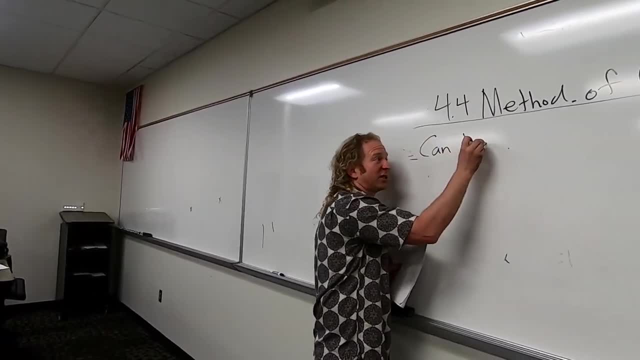 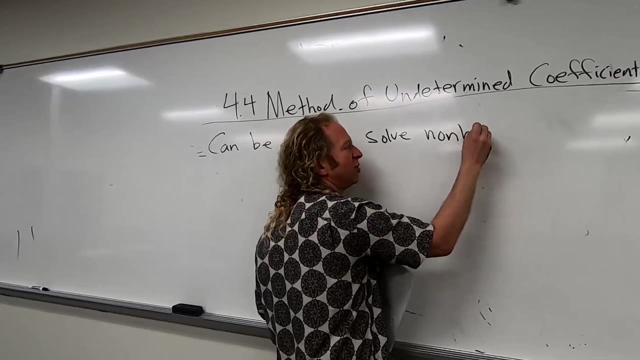 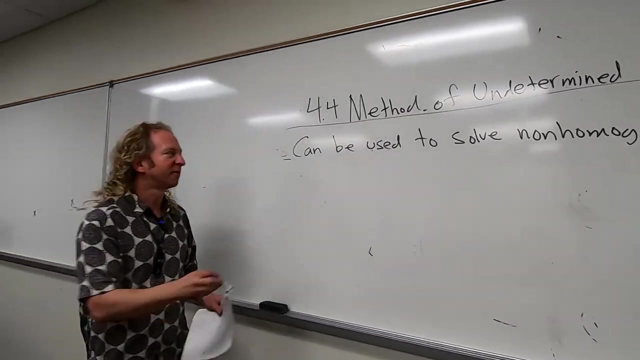 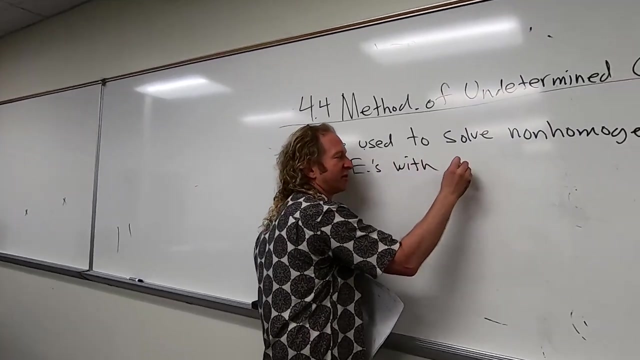 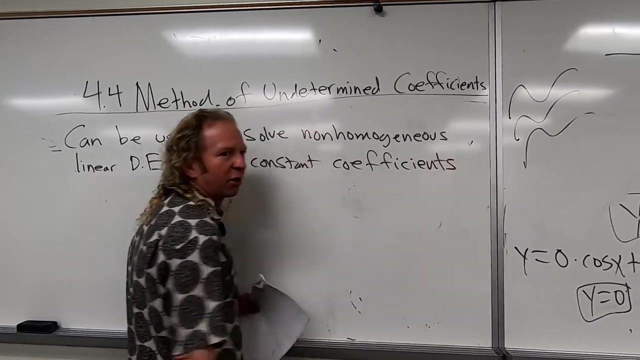 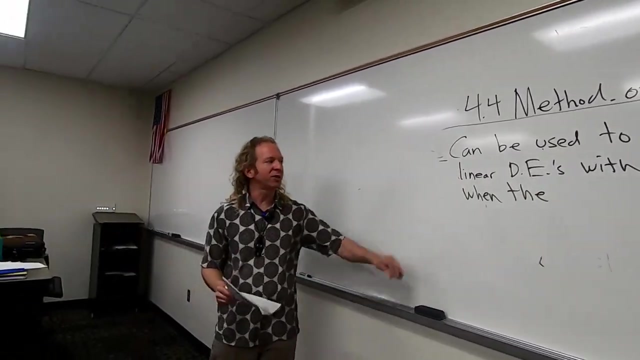 So this can be used. doesn't have to be used, just can be used to solve non-homogeneous- I'm writing a little bit fast- non-homogeneous linear DEs with constant coefficients. that's a lot when I'll pause here the so this can be used to solve non-homogeneous linear DEs with constant coefficients. 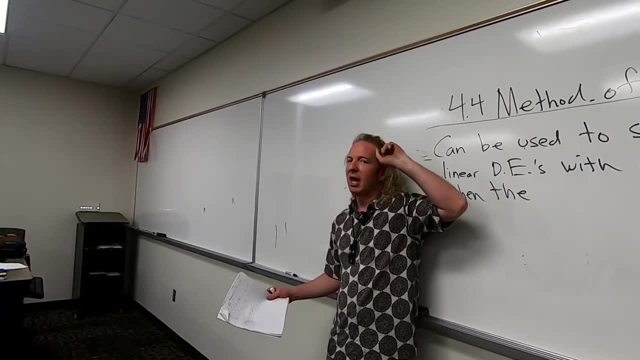 So, in other words, instead of zero, we're going to have something else on the right-hand side and we can only have numbers in front of the y's and y primes. What happens when you have variables there? It's different, okay. 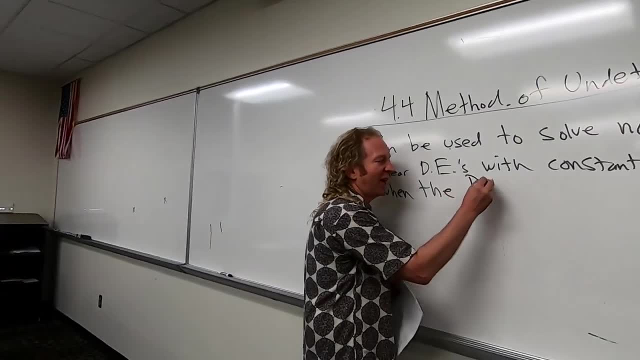 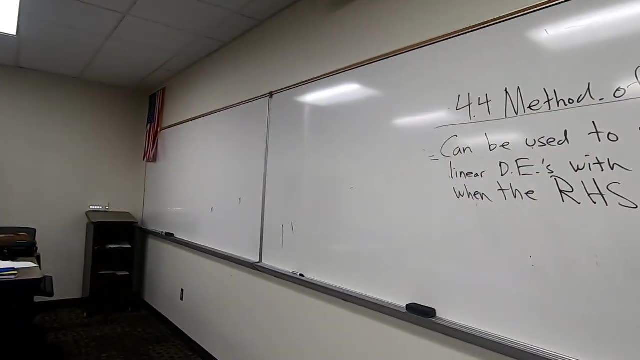 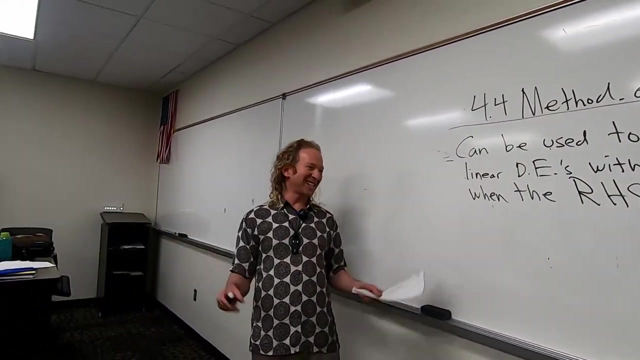 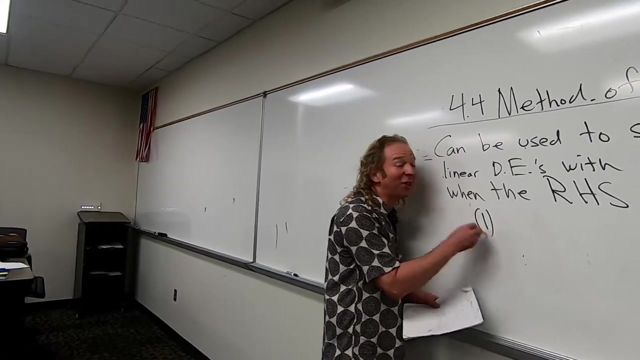 When the RHS is. What do you think? RHS stands for? Right, Right-hand side? Good, good, good. yeah, So when the right-hand side, when the right-hand side is one. This is a really specific method, by the way. 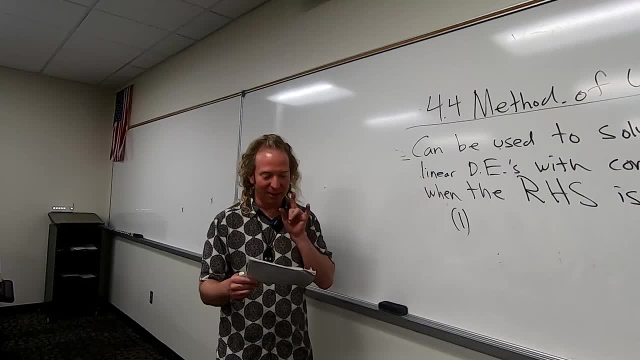 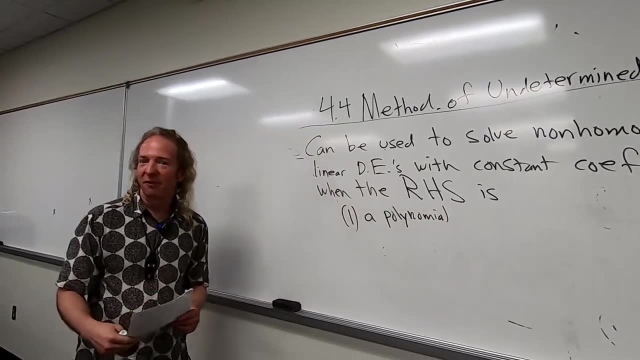 It's like so it's only when the right-hand side is a polynomial, So like x, x squared, x cubed, x to the fourth. We do some really beautiful problems. This section like, it's really really nice. 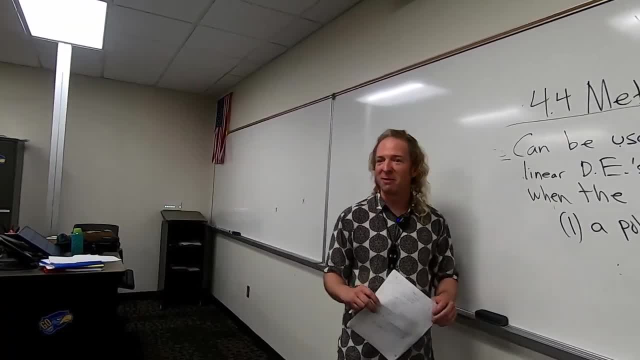 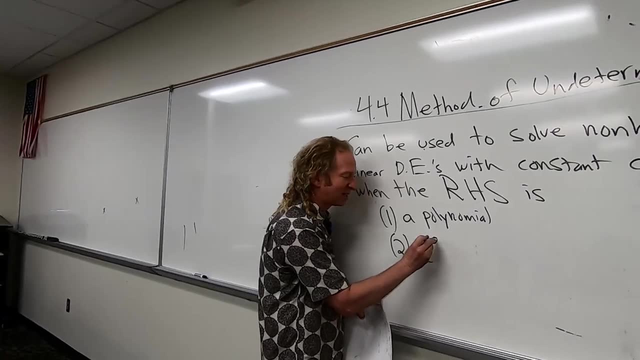 Like I mean I assigned almost all the homework that's available, so that means we have some hard ones. An exponential function with an e, so like e to the ax or like e to the 2x, You're allowed to have numbers in front of it too. like 5e to the 2x. 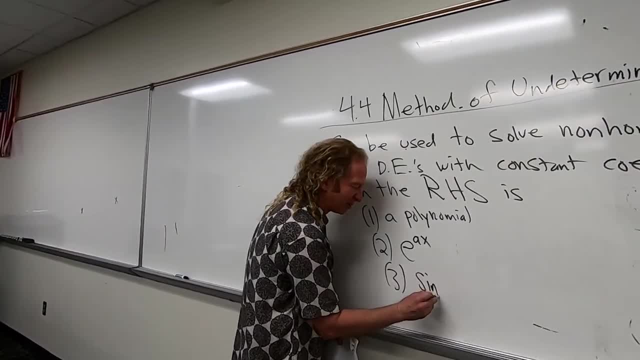 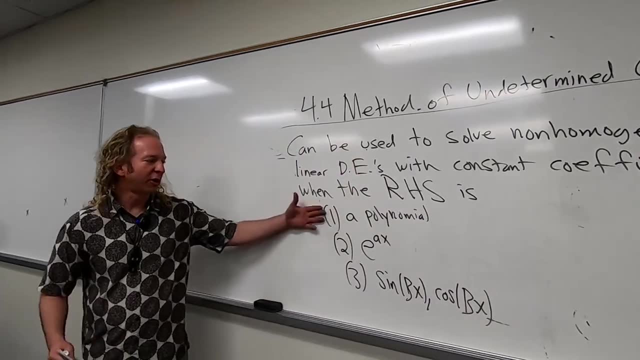 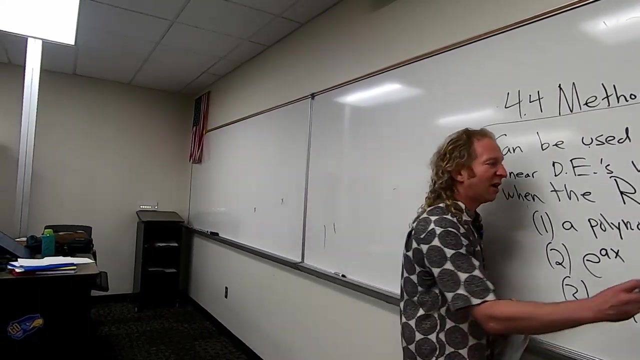 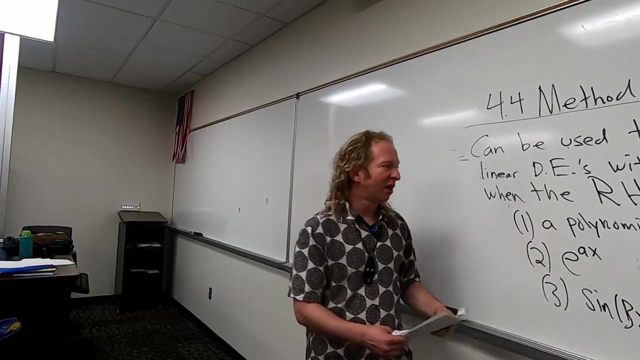 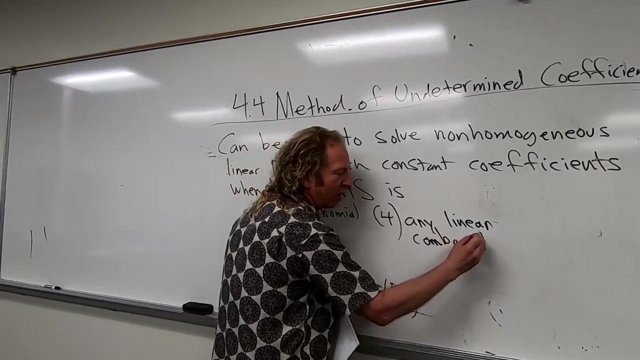 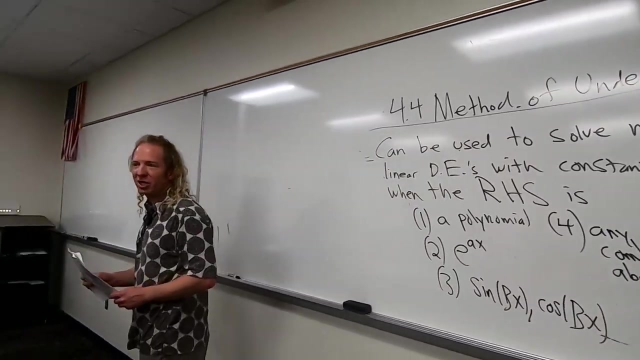 Three: sines and cosines, so like sine, beta x, cosine beta x. So polynomials, exponentials, Sines and cosines. so polynomials, exponentials, sines and cosines. and then four, any linear combination of these, so like x plus e to the x is okay. so any linear combo- this is the word- combo of the above, any linear combo of the above, any linear combination of 1,, 2, and 3.. 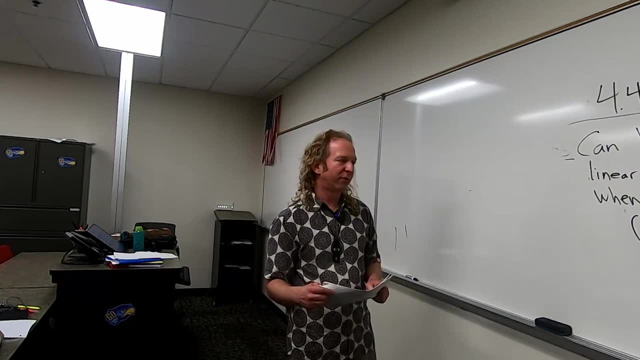 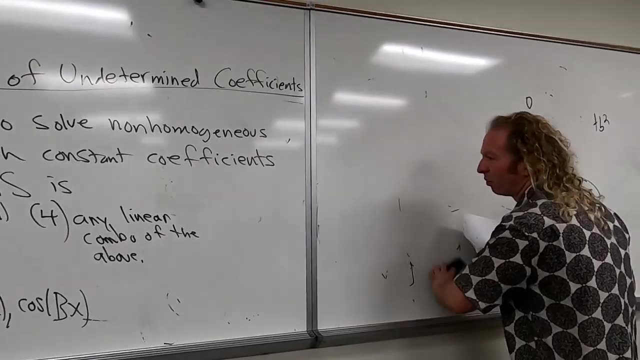 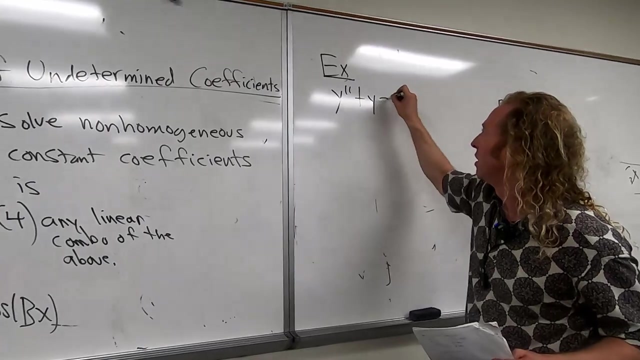 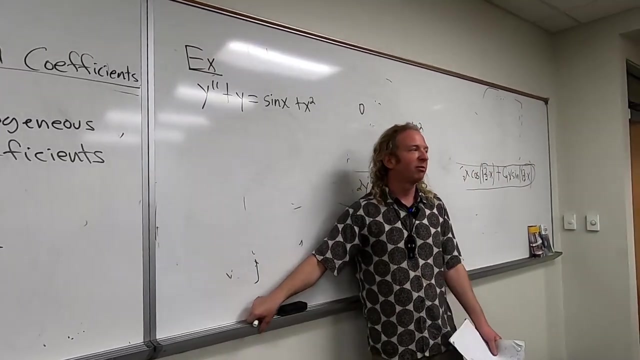 So let me just briefly give you some examples so you see when it can or can't be used. So just some examples. Say we have y double prime plus y equals sine x plus x squared. So we just did this problem, except we had a zero here. 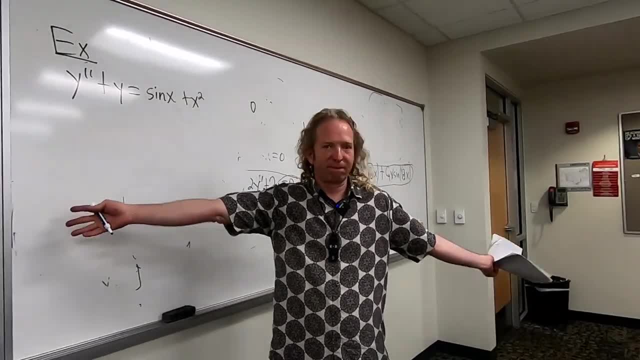 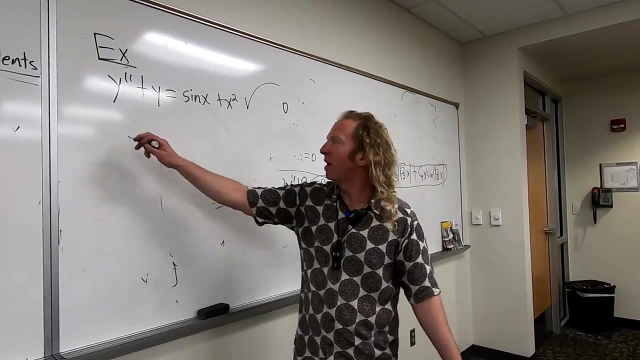 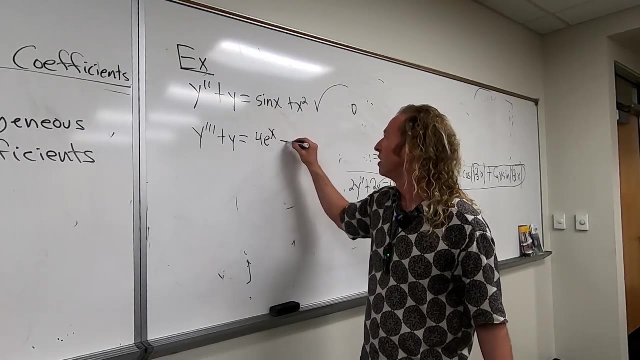 Could we solve it using this method? What do you think? Yeah, it's just a linear combo of the above. It's this one plus this. this is good, Yeah, Yeah. or how about y? triple prime plus y equals 4e to the x minus cosine 2x. 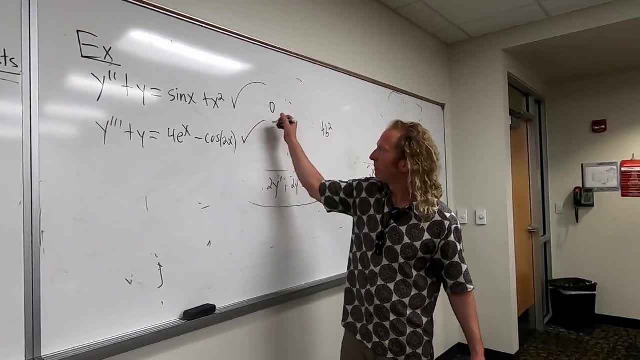 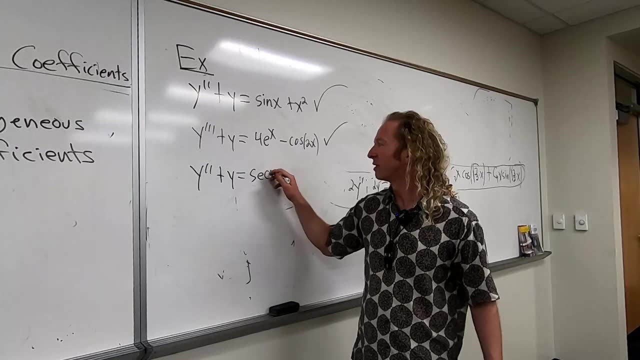 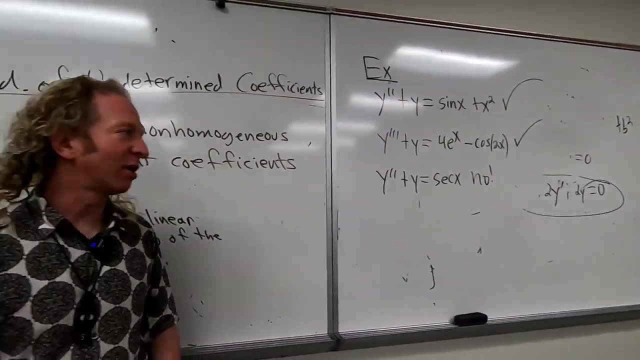 What do you think? Can we use it? Yep, Yep, Mm-hmm. What about y double prime plus y equals secant x. What do you think? No, No, No, No way, right, And it's 1 over cosine. that doesn't count, right. 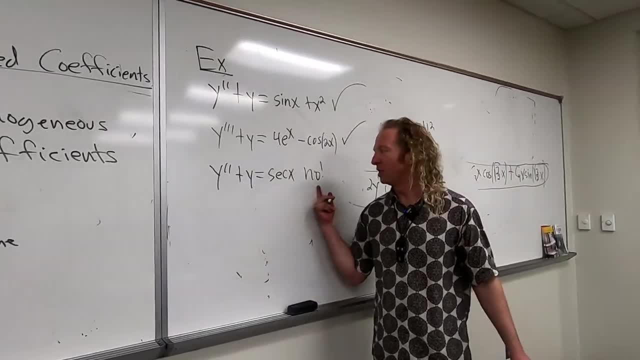 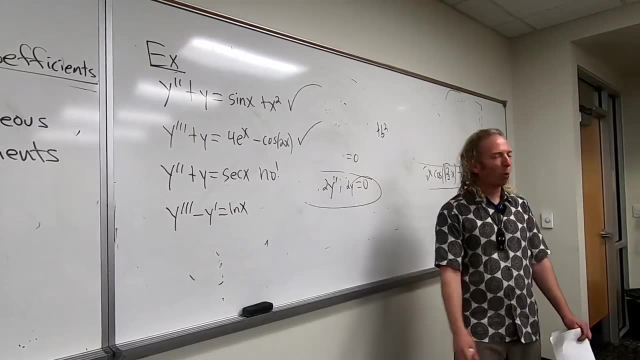 It's got to be just cosine or sine Fails the evil secant function. What about this one y triple prime minus y prime equals ln x. What do you think? No, No, Not possible. So we're really restricted. 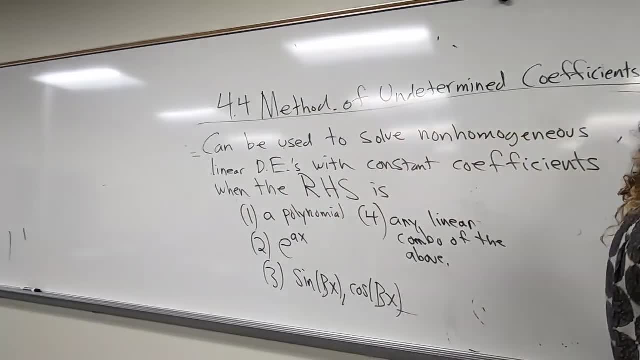 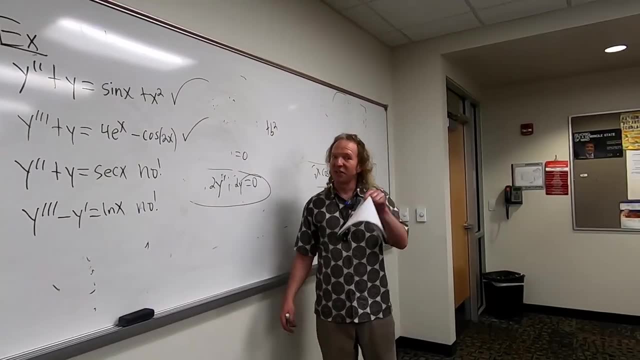 In 4.6, there's no restriction here. So I tell you, why would we even do this? What's the point? right, I mean, I would skip it if we didn't need it, Because in 4.6, you have to integrate. 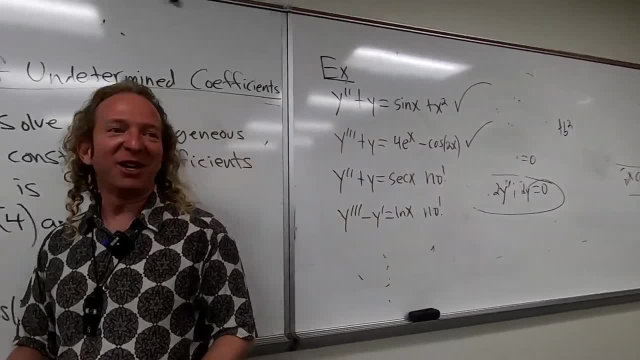 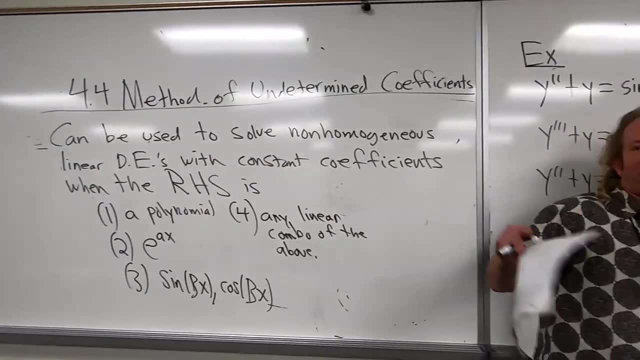 You know what that means, right, Harder problems, right So. and it also means integrals you can't do. You might get an impossible integral. So the next in 4.6, there's only seven homework questions. 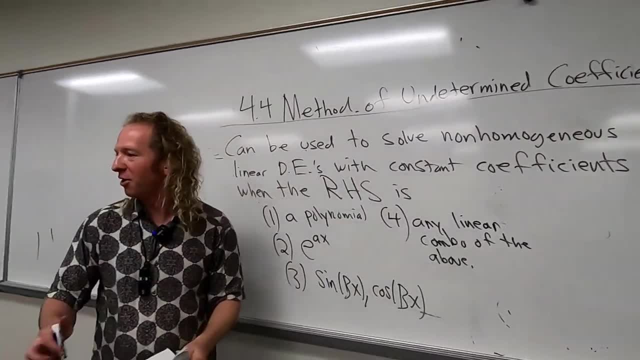 It's like these are the steps. here's the problem: We can do 4.6 in like 45 minutes. I'll just show you. That's how long it'll take to do a problem carefully. There is 4.5.. 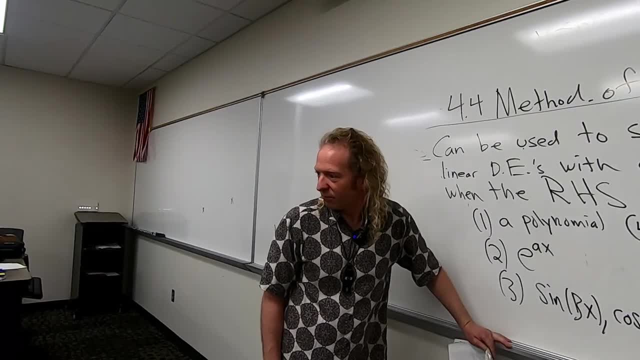 No, we're going to skip it, though. So the next class is just going to be 4.6?, 4.4 and 4.6.. We're going to do more 4.4.. Yeah, I want to do more. 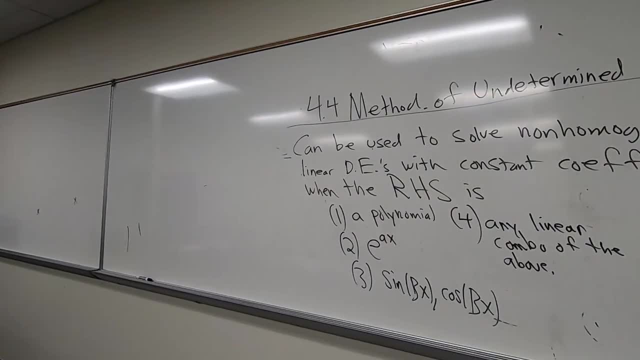 I want to make sure you got this. 4.6, I can do one or two examples and you'll be good, But 4.4, we have to build up to the process. Yeah, so let me give you the steps now. 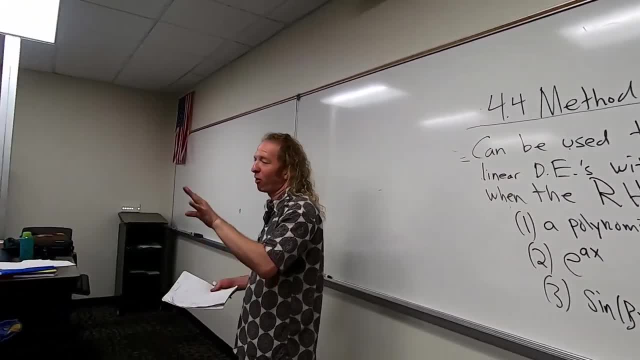 Like step one, step two. I'm going to write down the steps very carefully And then we're going to practice some of the steps. The homework will not give you steps. This is where I was saying on the test. I'll give you the steps. 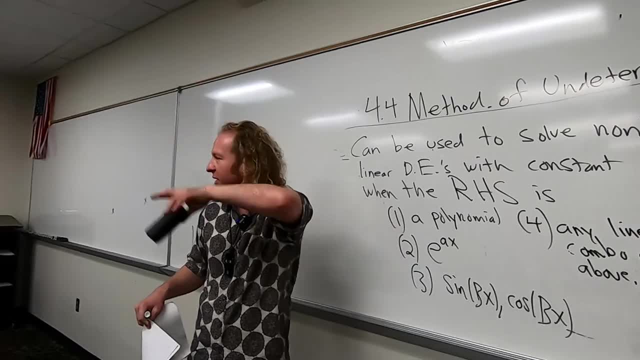 Okay, so on the test, I will give you the steps. It's the same steps as the old exam, So the old exam is actually really good practice this time, So it's worth it. I know last time the old exam it was all right. 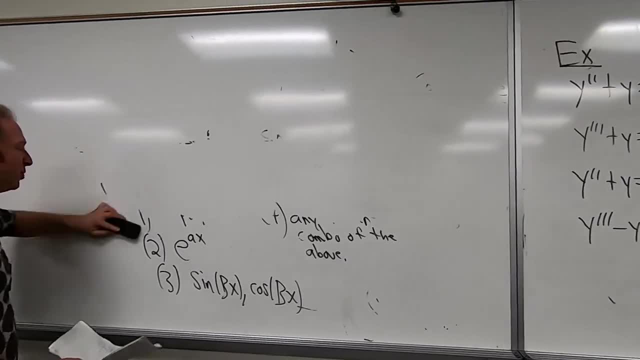 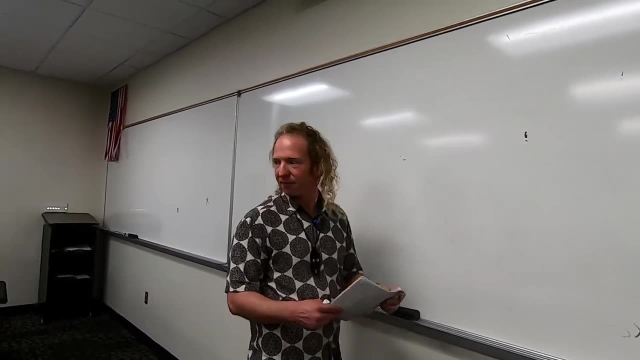 I mean, the DEs might have been different Here, they might be different too, but at least the steps are the same And there's more similarity, I think this time, no matter what I put on the test, No, that's not correct. 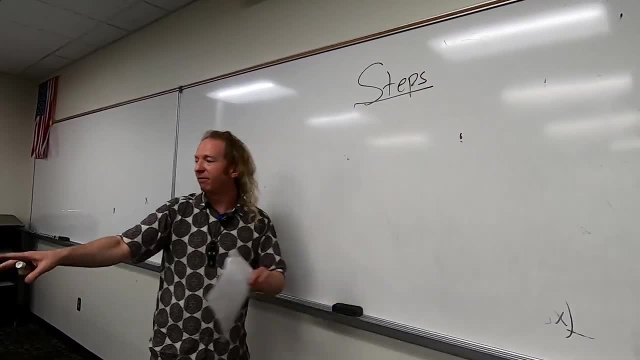 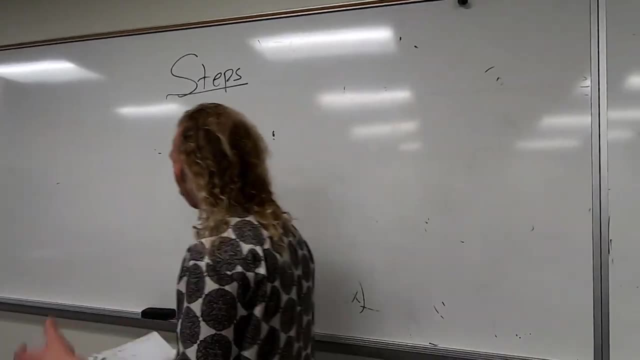 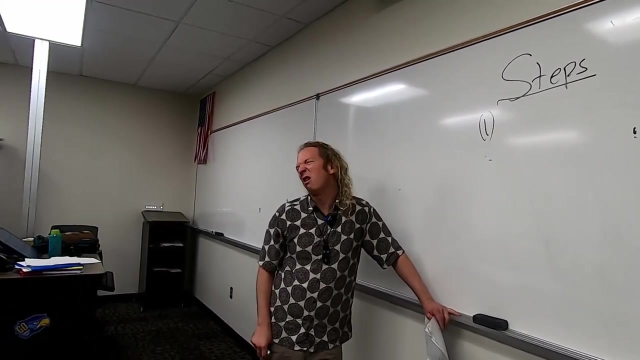 Steps: The old exam. The old exam two. Yeah, you have an old version of the test. Yeah, no, the old exam two. No, I was just. You didn't upload a test for COG-3.. No, no, you don't. 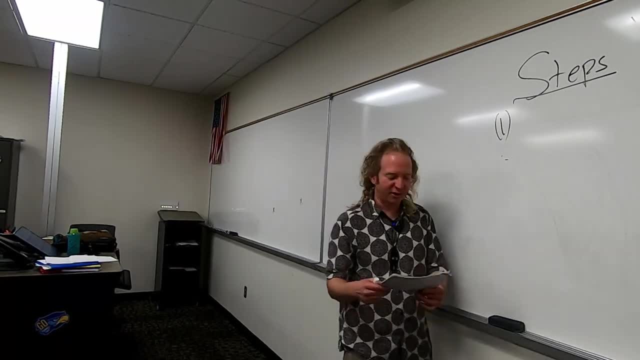 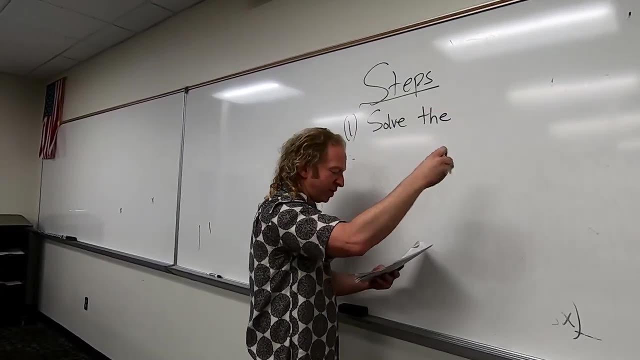 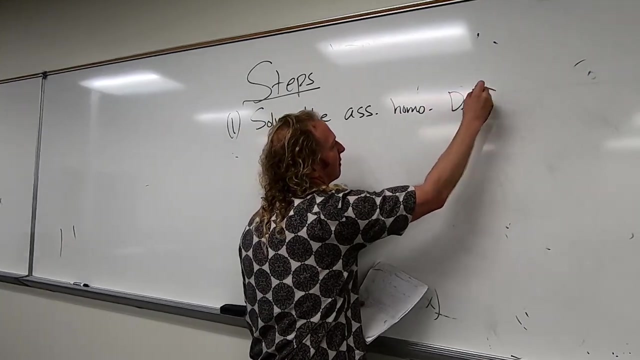 Okay, You have review questions? Okay, yeah, yeah, For this it's harder to give. review: Solve the associated homogeneous differential equation. I can abbreviate that: Solve the associated homogeneous DE. Solve the associated homogeneous DE. It's solution. 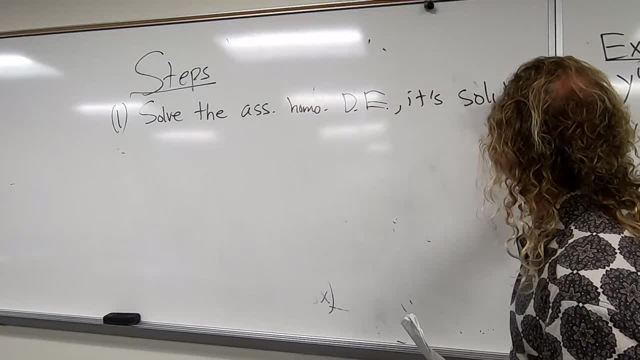 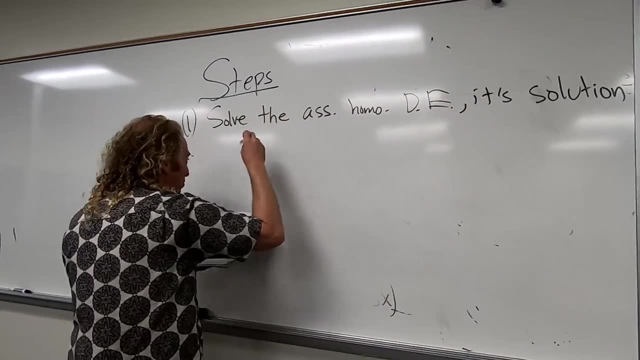 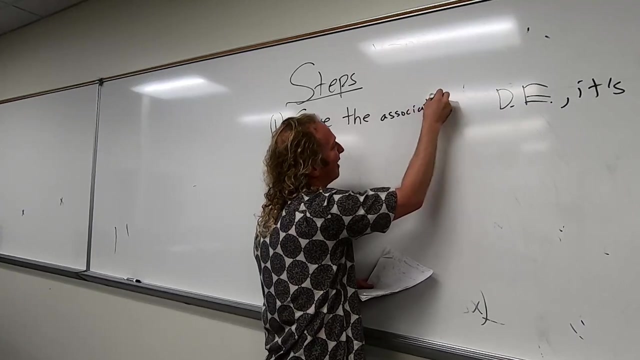 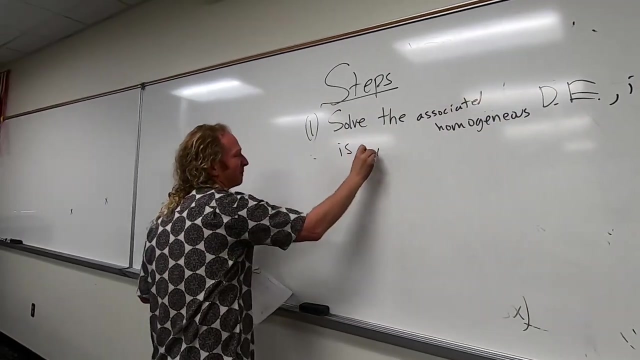 It's solution. ASS means associated Solve. the associated It's solution is, Let me just spell it- Solve. the associated homogeneous DE solution is YC. It's solution is YC. Yeah, it's just whatever. It's ridiculous. 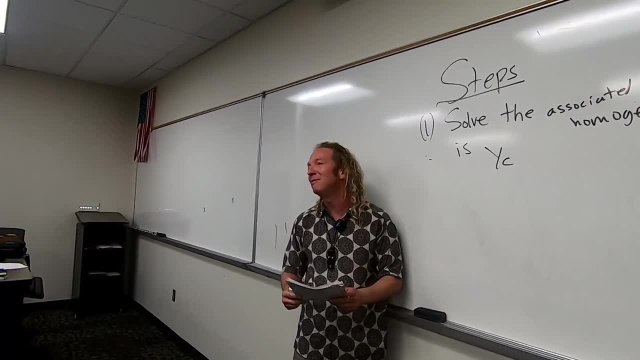 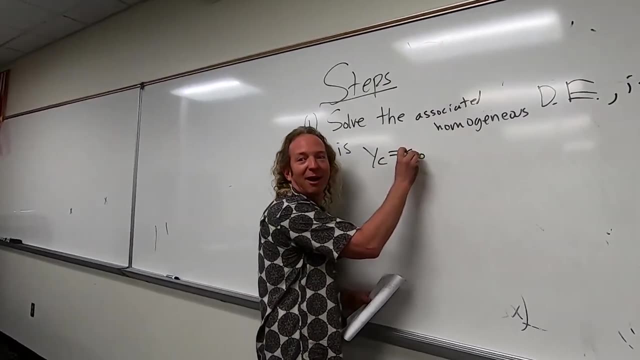 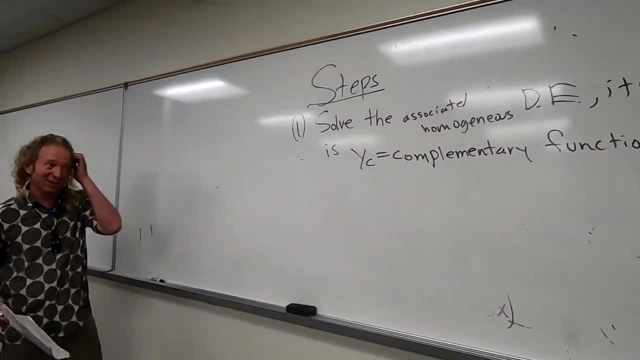 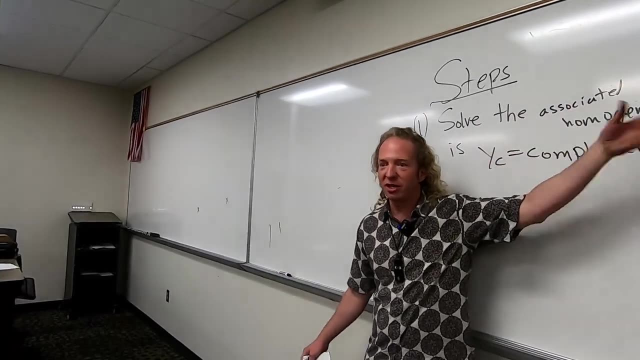 So solve the associated homogeneous DE. Its solution is the complementary function. Yes, Oh, we find the auxiliary equation. So this is 4-3.. We just did, We just did this. Yeah, So step one is going to be what we just did. 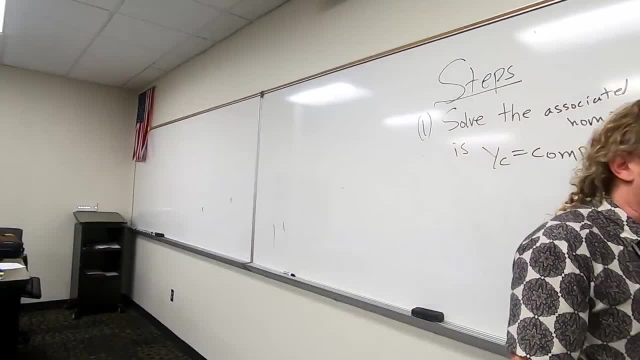 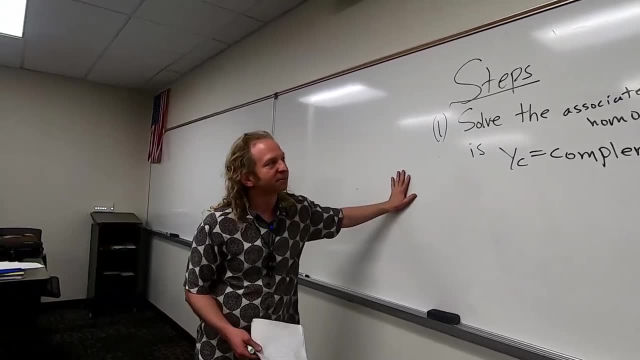 except it's easier in this section. There's no rational roots theorem. in this section, I mean whenever it's this problem on your test, it will always be easy. You made a grammatical mistake. You can't put an apostrophe after that S. 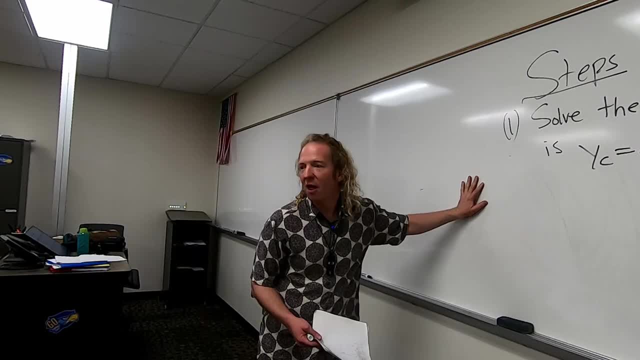 because it's. I mean it is. I thought it was possessive. No, it's. You don't do it with its. You don't do it with its. Yeah, no, Someone like You don't only do it. 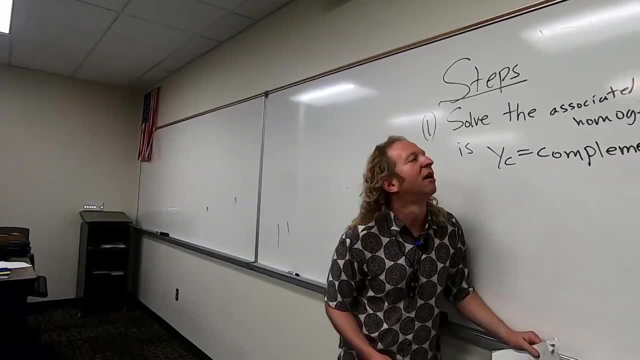 You don't do it with its. No, It's like, Because it's its You got to take the apostrophe off, and then that one points. No, it's grammatical, So I mean It's half a point. 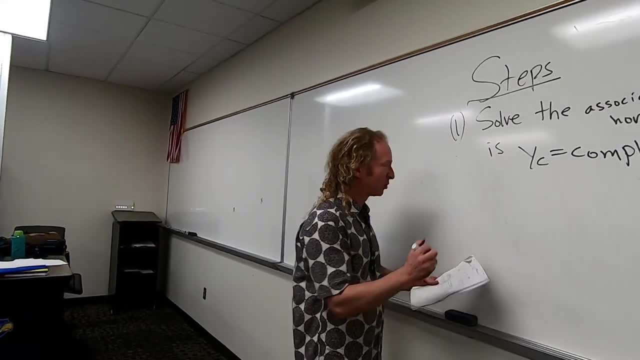 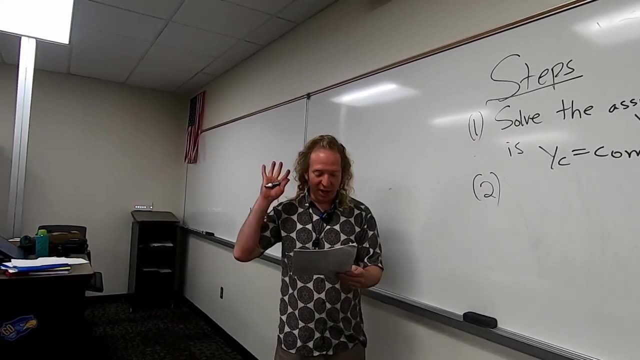 It's half a point. No, no, no, it doesn't matter. Two: this is the tricky part, Remember. the homework just says: solve So on a test. this will be part A, okay, Two: make a guess for the particular solution. YP. 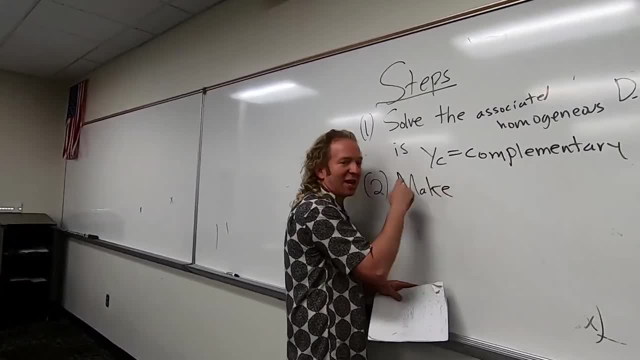 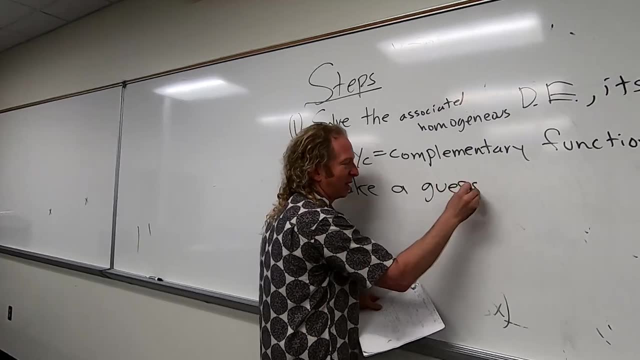 We're going to practice this a lot today. It's like on your test. you'll have to do this too. I'll have a question for this, and I'll show you what I mean. Make a guess. I'm going to show you how to guess. 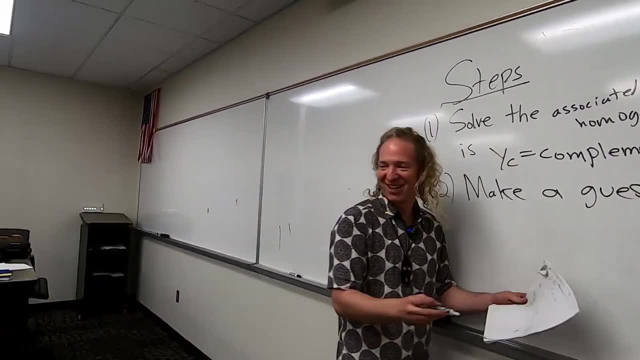 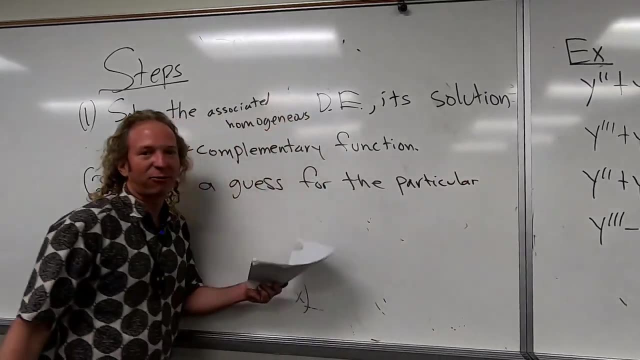 so that you always guess. right, Make a guess, for It's in the book, but the book doesn't really like. Yeah, I don't know, You can't really write down a formula. It's kind of hard For the particular solution. YP. 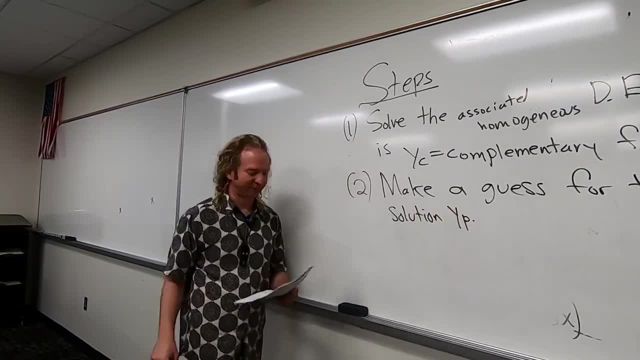 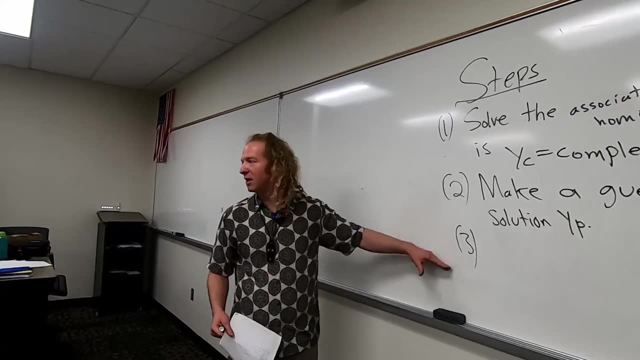 So we're just going to do a ton of examples. YP Three: I made these steps up by the way. So like I break these steps up into two steps, like This could really be one step, but I'll do it in two steps. 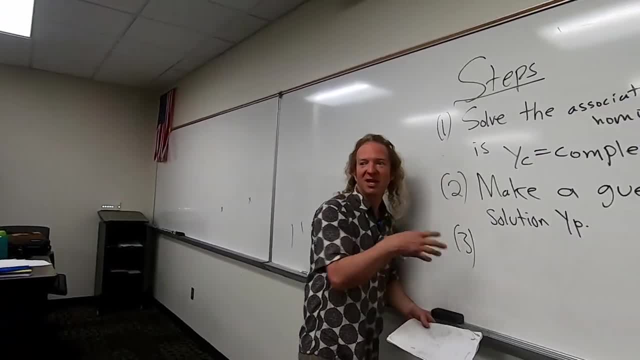 and I'll show the work for the steps. Isn't there a chart? Yeah, there's a chart, but Yeah, there's kind of like a chart and it gives you like an idea, which is important. 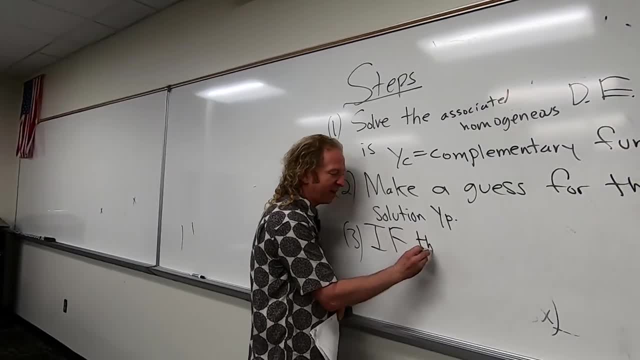 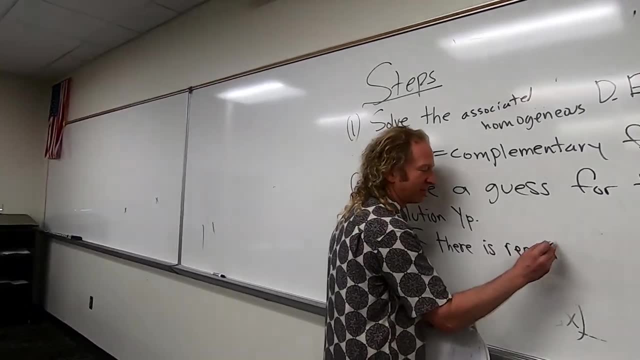 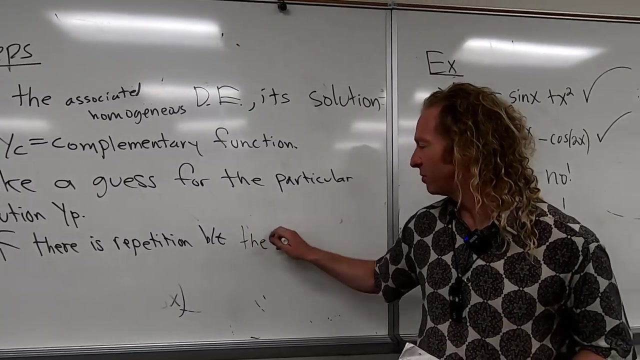 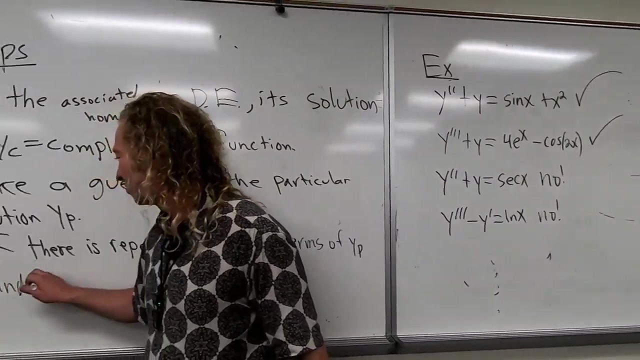 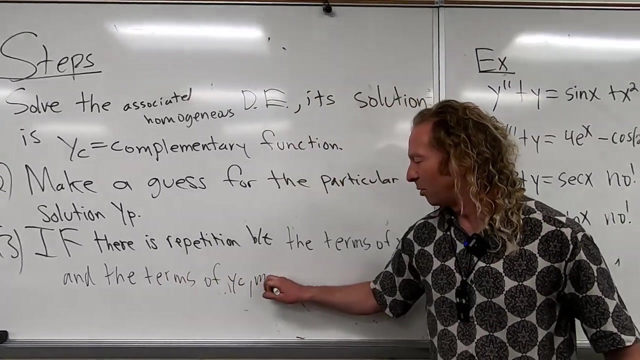 Two: if, If there is repetition, re-re-re-re-repeh, repeh, repetition between the terms of YP and the terms of YC. So the terms of YP and the terms of YC and the terms of YC multiply the terms. 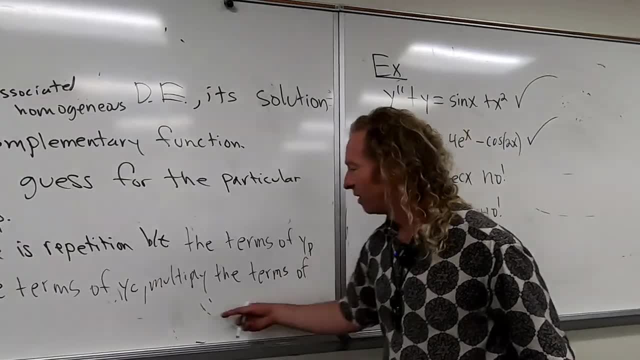 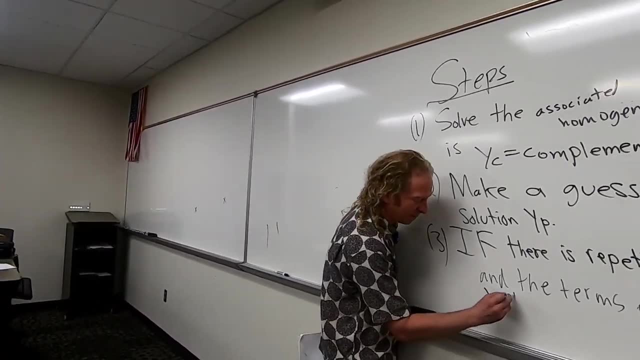 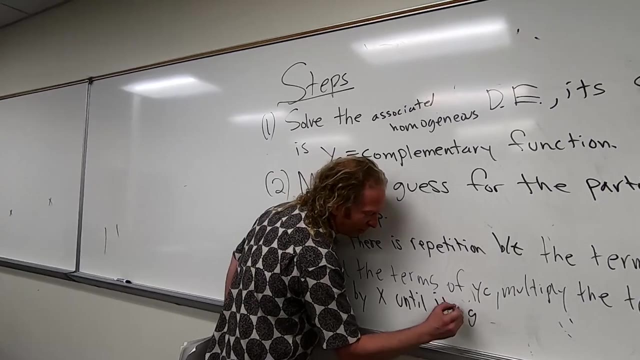 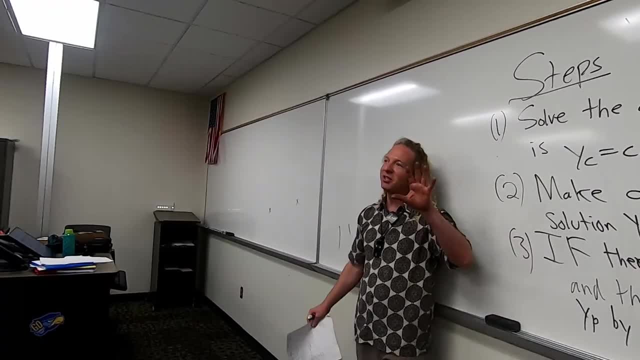 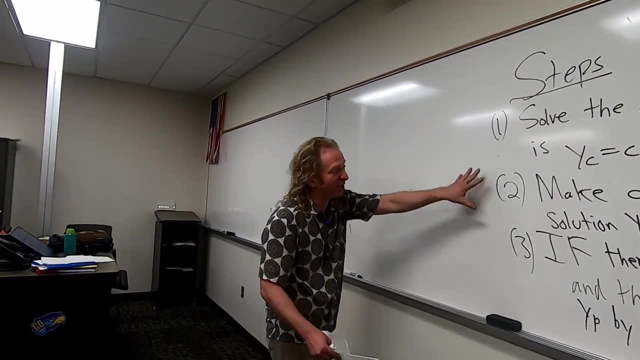 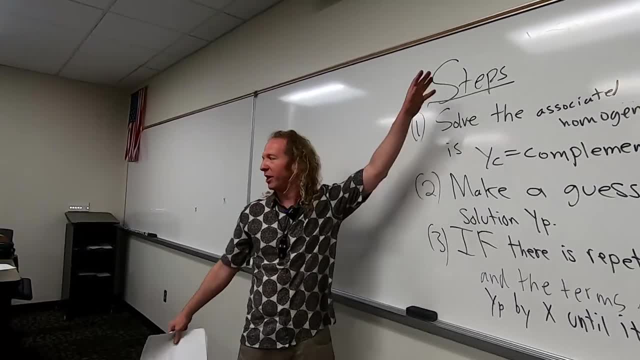 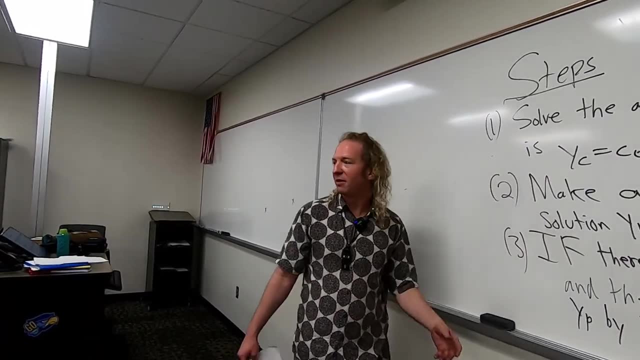 So this is easy, This is tricky, So I There's a worksheet I uploaded to WebAssign and it has like ten problems. We're going to do it in class today. Okay, That worksheet will be on your test. 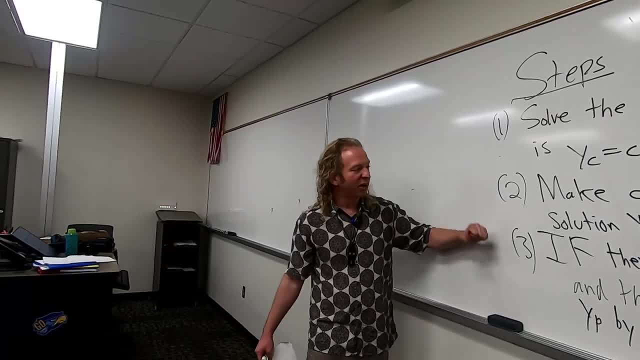 Like you'll have a question like that, So it's really This will help you. So you're supposed to do all of this in the homework, even though it just says solve. So this can be really sneaky. 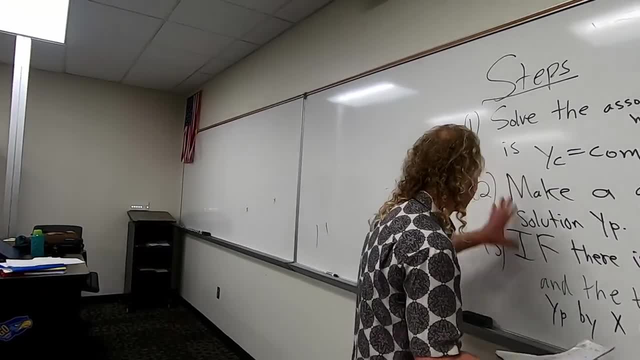 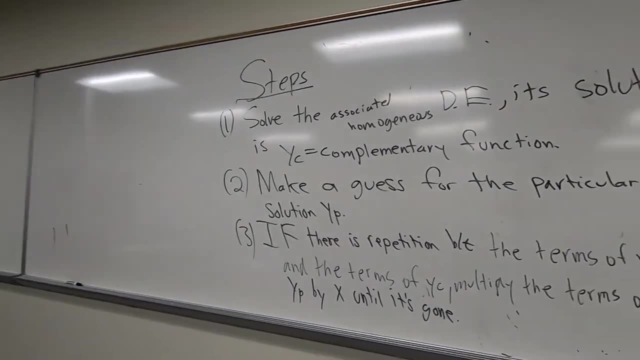 So we'll spend some time on this Four. So this is just, It's not messy, It's just tricky. Four is what makes the problems long. So four: you have to find YP. This is like: 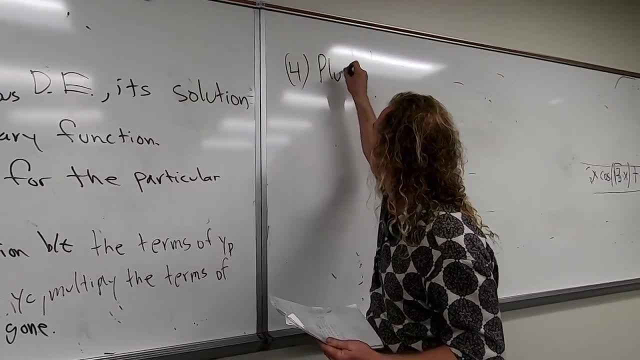 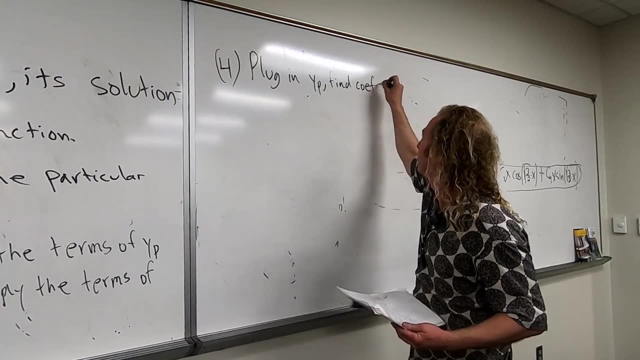 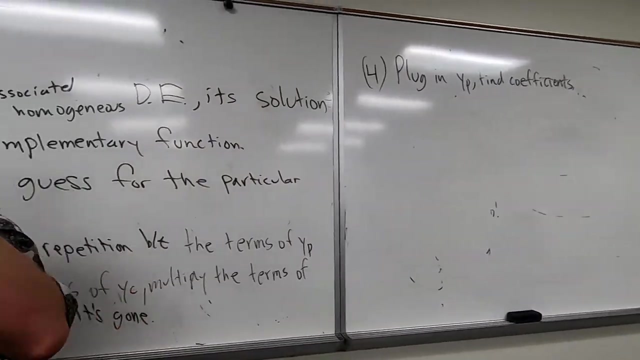 This is messy. So plug in YP. Plug in YP, Find coefficients. So you plug it into the DE. I'll show you this. This is the messy part Again, the old exam that's under resources, and WebAssign is extremely good. 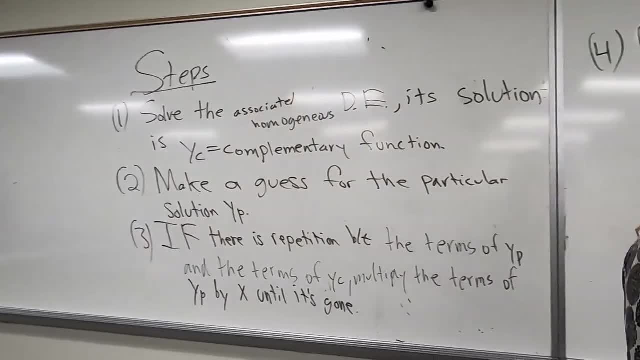 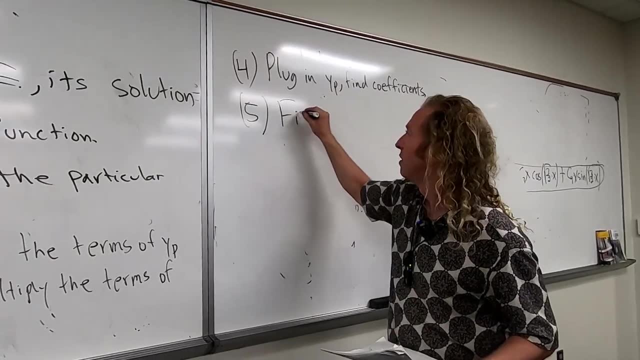 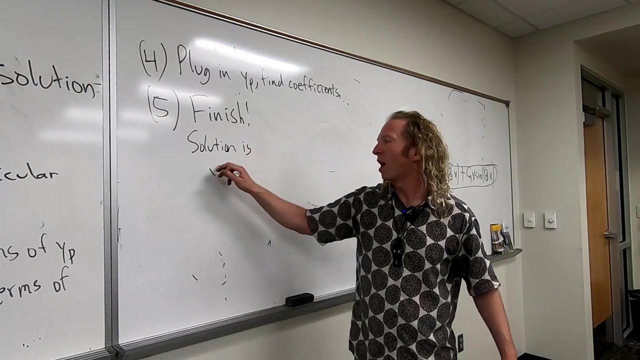 It's got some harder questions. That was a really tough exam. It's got some harder ones, So this will be useful. And then five finish. I think we talked about this last time. The solution is Y equals YC. 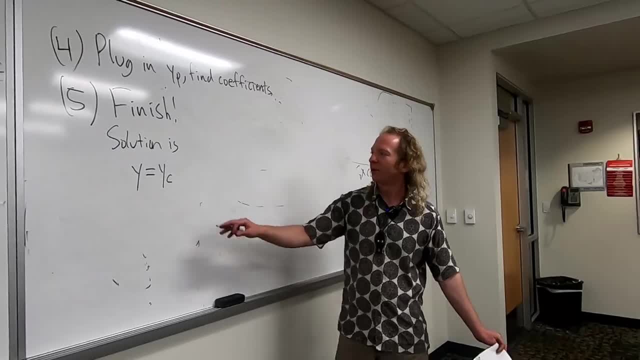 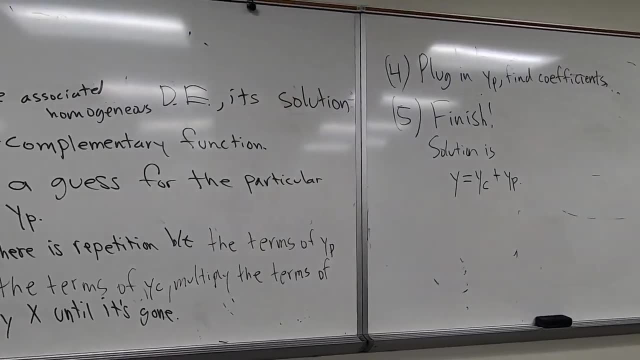 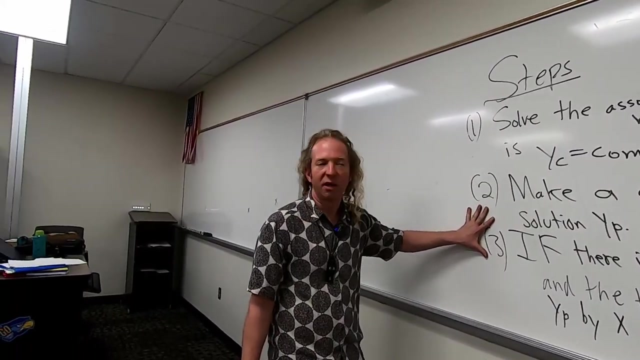 Plus YP. That's the solution. That would be the solution. So, on your test. this will be part A. This will be part B. This will be part C. This will be part D. I'll give you the parts. 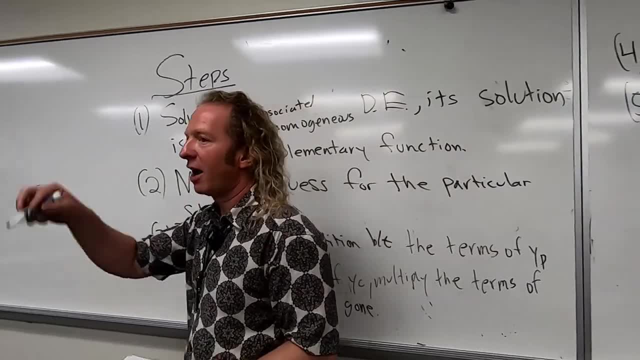 You'll see them Like part A will stay. When we do an example today, I'm going to word it that way, Like I'll write part A, part B on the board. so you see, It makes it easier to grade too. 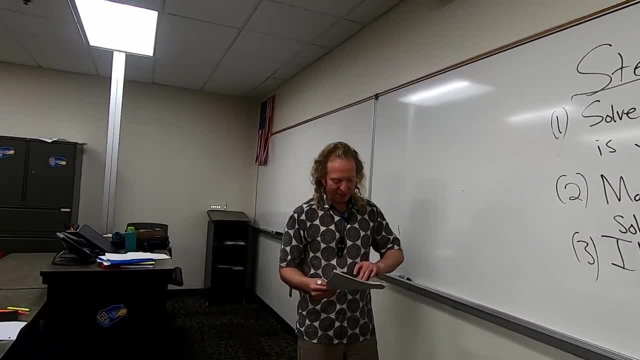 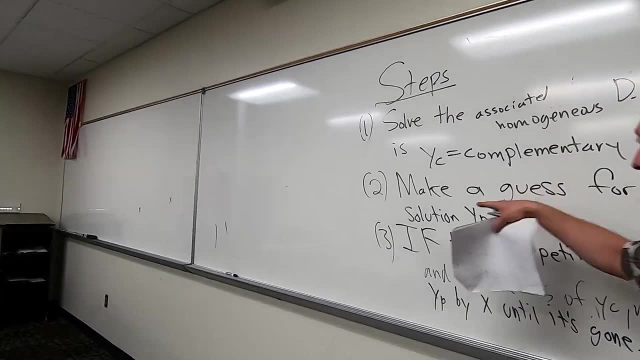 Way easier to grade. Let's warm up. Let's warm up. I have some examples in my notes that I'd like to do. Let's just focus on step two. Let's just do like six or seven examples of step two, of just this. 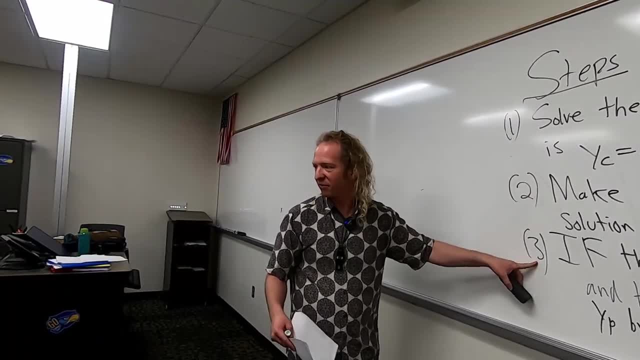 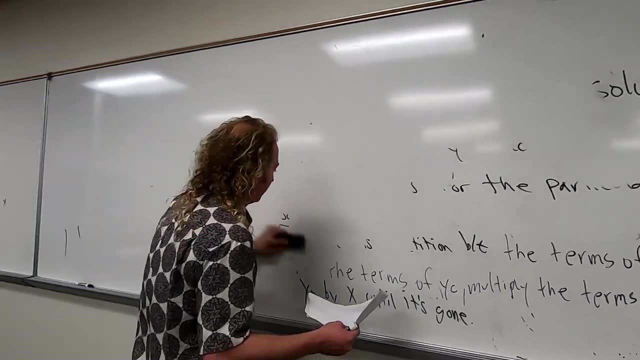 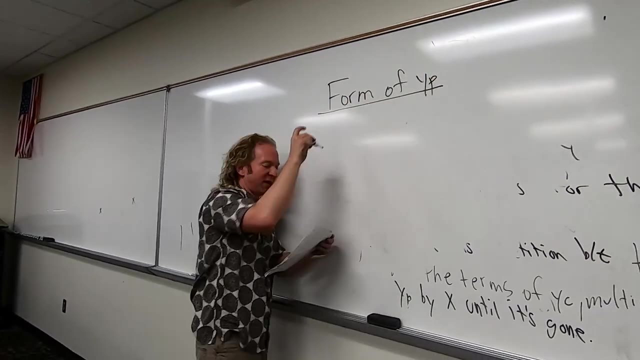 And then we'll do some examples of this, And then we'll do a DE, And then we're ready to do it, Then we're done. So, form of YP, Form of YP. So we're just focusing. 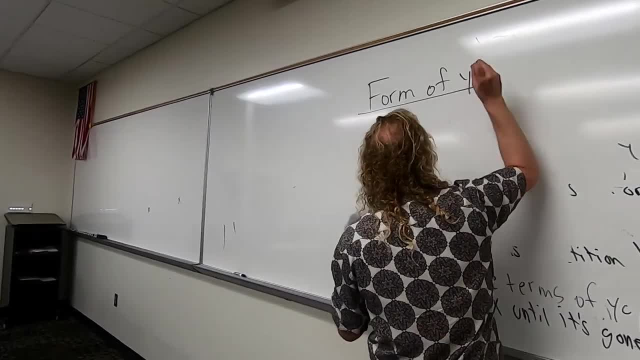 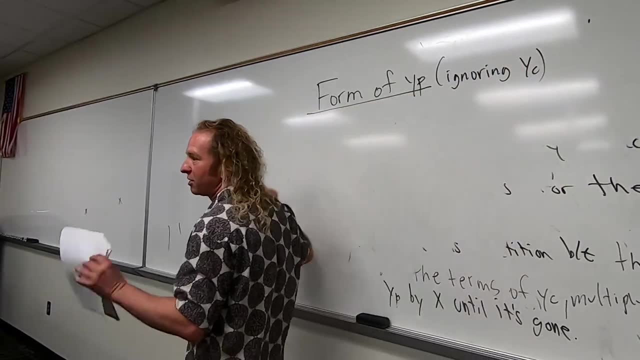 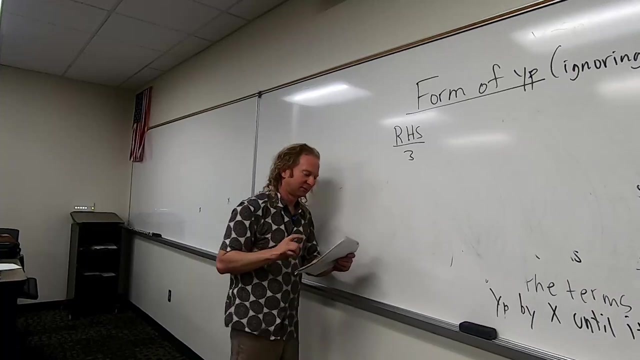 We're ignoring the homogeneous, So we're ignoring YC, So just ignoring This is just step two. we're practicing, okay. So let's say, the right-hand side of your DE is three. Okay, then, over here I'm going to make a table. 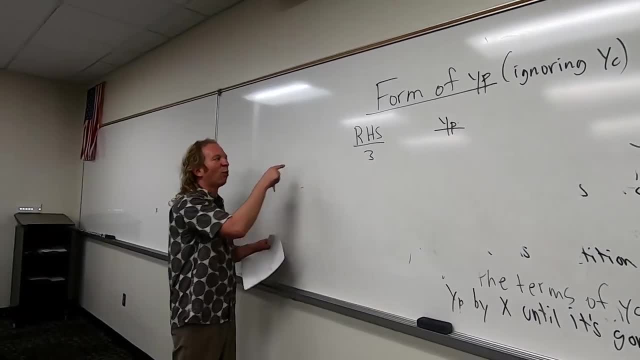 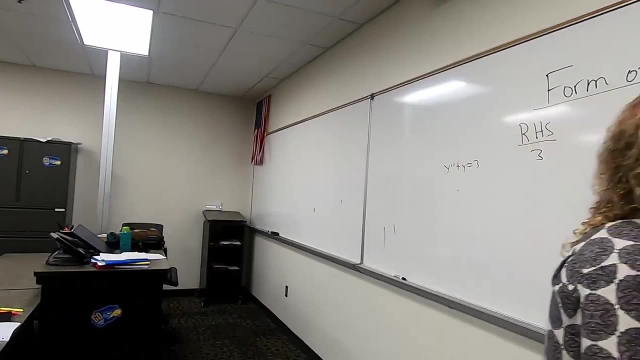 And we're just going to practice. So like say you have like Y over prime plus Y equals three. So that's three is on the right-hand side. That's what I mean by RHS. So whenever you have a number, your YP has to be just generic. 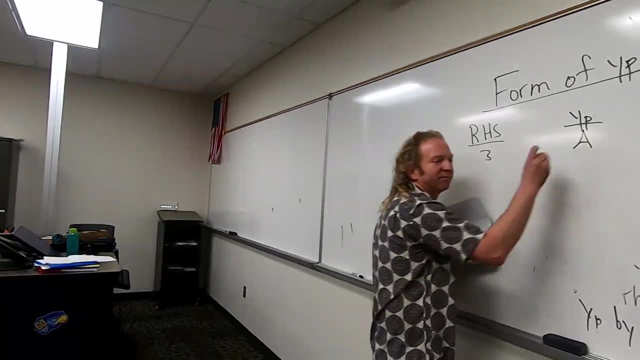 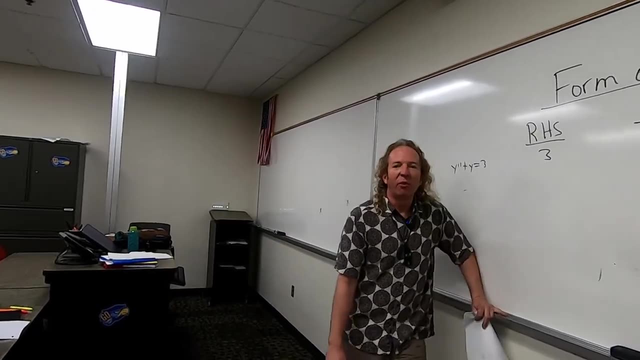 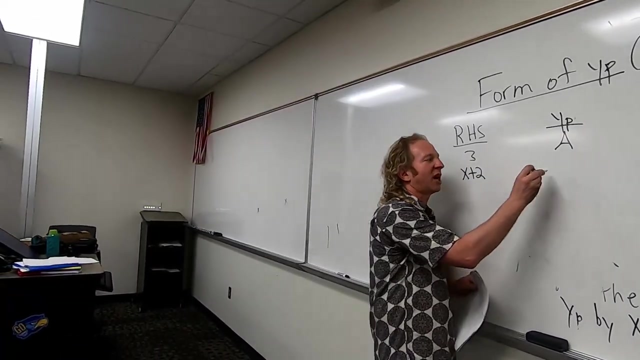 So just A would be the answer. So A. So if it's a number, you just put A. Okay, so just A. What if you had X plus two? This is linear, So you would do AX plus B. 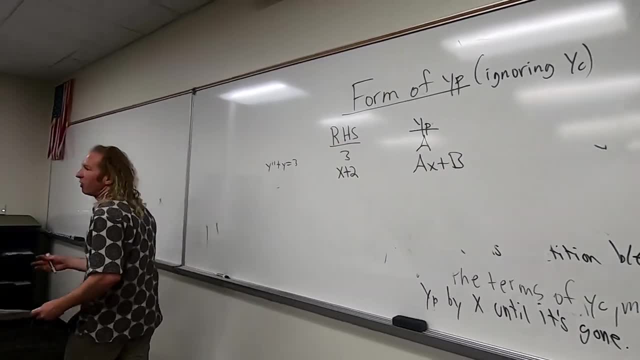 Very good, AX plus B. I know you all want to break soon, but I figured like we should just push a little bit more. I know, Do you need to break soon, Momodou? You're good, You're good. 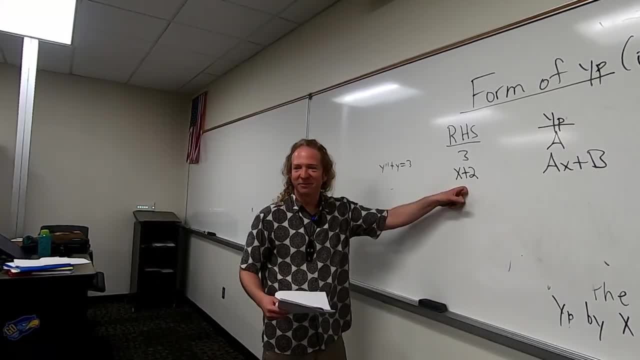 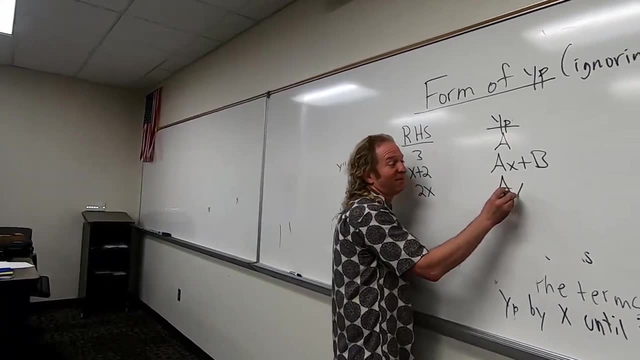 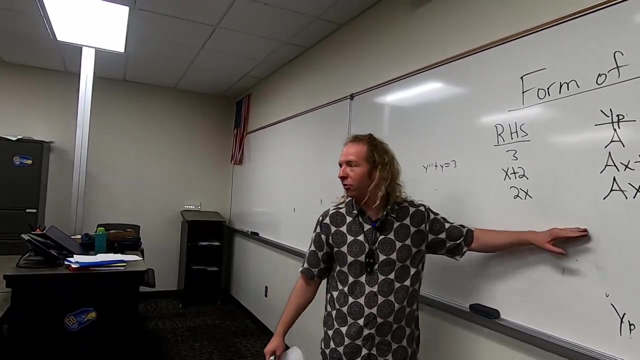 That's all right, That's good. What if it was just 2X? You still need the same right. You need the full linear. because you need the full linear, Even if it's 2X. you want the full linear okay. 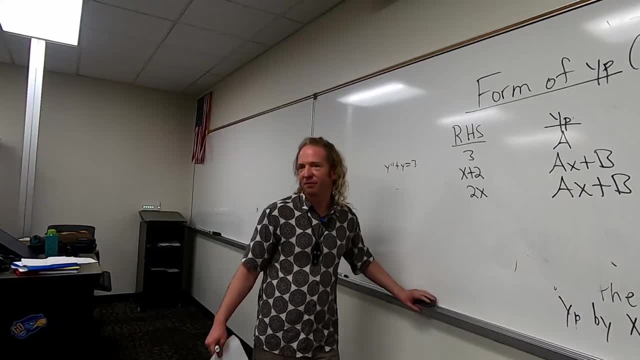 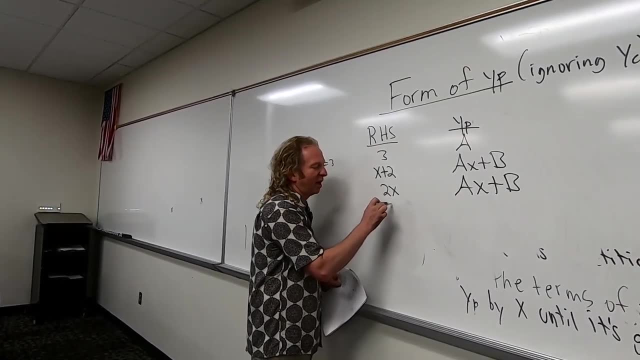 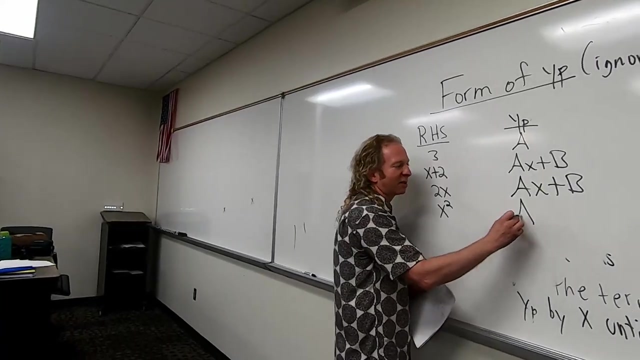 You need the full AX. You need the full AX plus B. Okay, you need the full linear. Let's say it's X squared, Then you would need a full quadratic. Yeah, so it would be AX squared plus BX plus C. 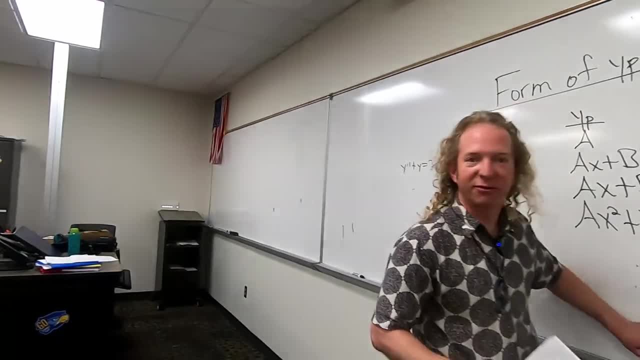 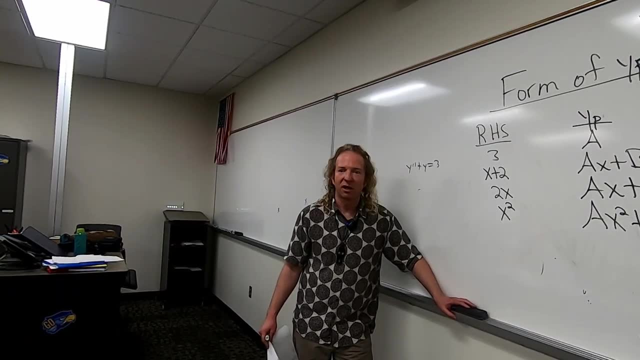 AX squared plus BX plus C. See how it's a full quadratic. It's a full quadratic And we'll be able to determine that From the right-hand side of the DE. Okay, So like if it was this Numbers the rows of these: 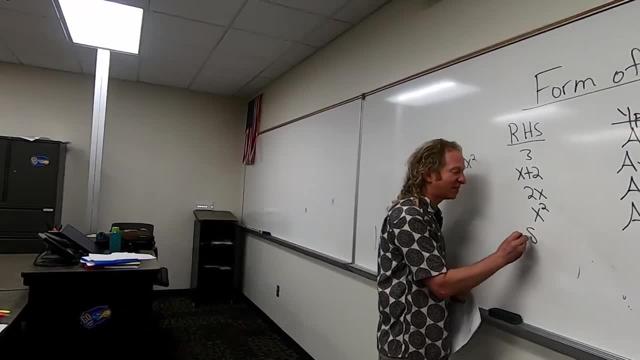 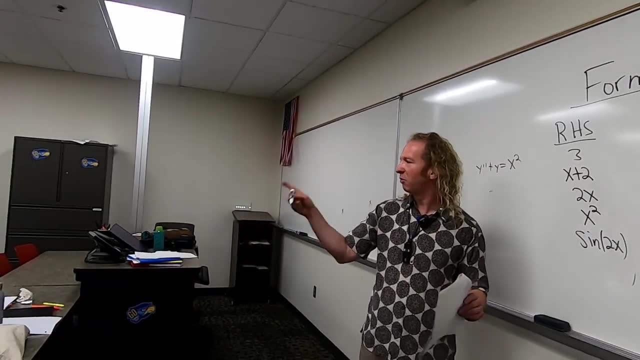 Right, Yeah, Yeah, whatever is here. Say it's a sine, Say it's sine 2X. Do you remember something about sine? Whenever you had the answers, it always came with a what, Also with a cosine. So whenever you have a sine, you have to include the cosine too. 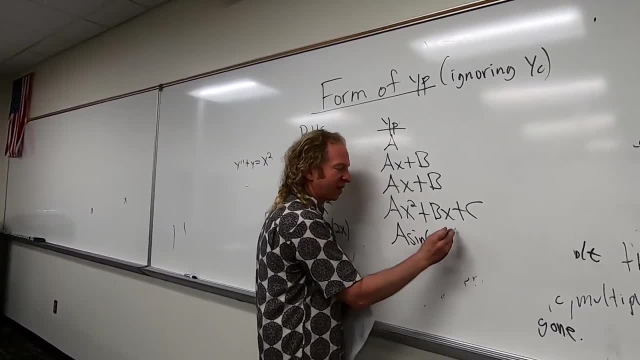 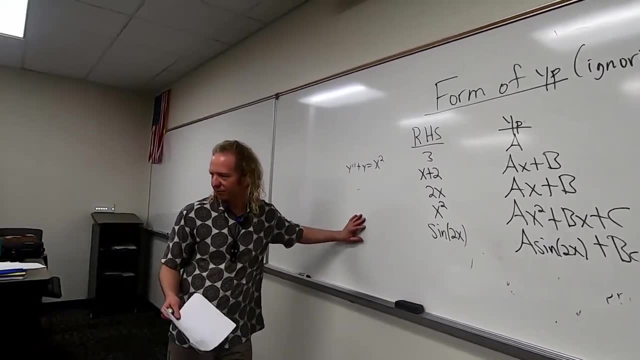 So it'll be A sine 2X. They come in pairs Plus B cosine 2X, So sine's in cosine. This is always true, This is always true. So why is it a guess, I don't know. You can guess. 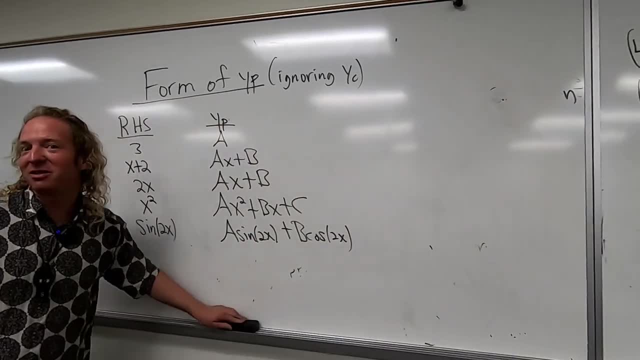 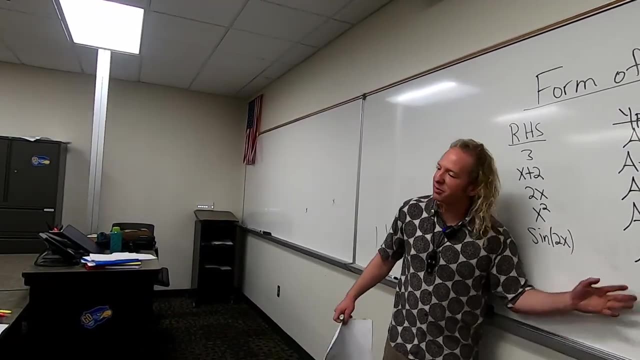 I guess because you can. I guess it's a guess because you can make a guess that's not the best guess and still get the right answer. Like you can deviate from this a little bit and still get the right answer sometimes, Which is not fun to grasp. 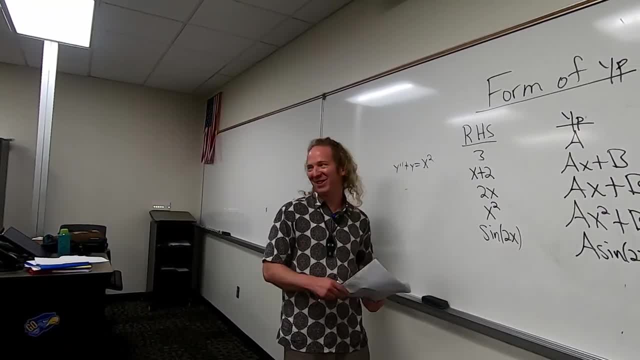 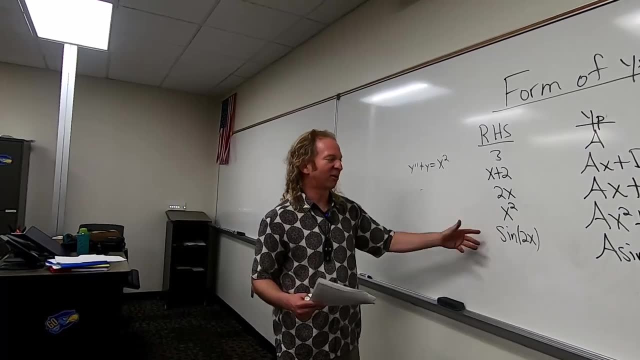 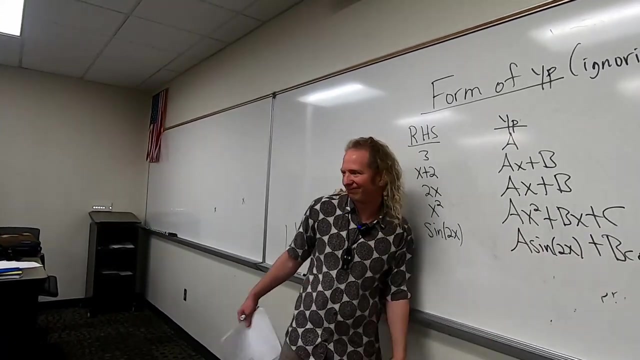 Which is not fun to grade. It doesn't really think about it Like huh, Sometimes people will like they'll make the guess that I don't want and then it's still correct, so I have to let it go Like: if you put a minus here, I still have to mark it right, because you'll still get the same answer. 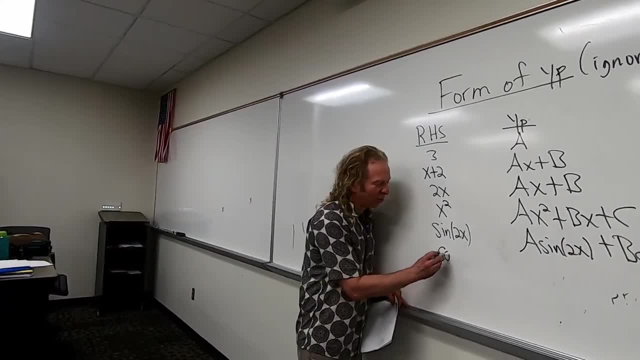 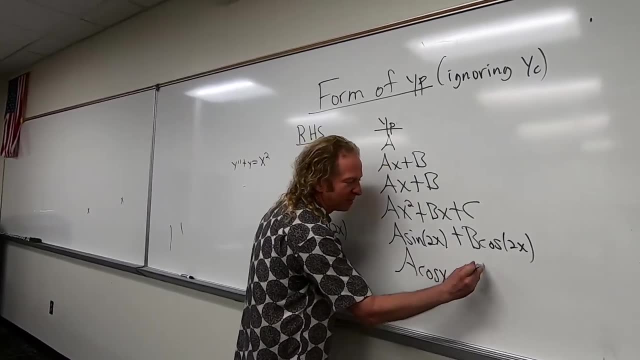 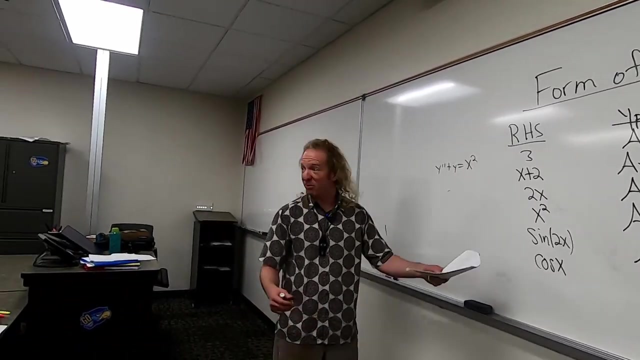 Okay, What if you have cosine X- Same thing, Same thing. So you have A cosine X Plus B sine X. Hey Nick, Let's keep going. I don't know why I said that It has nothing to do with you. 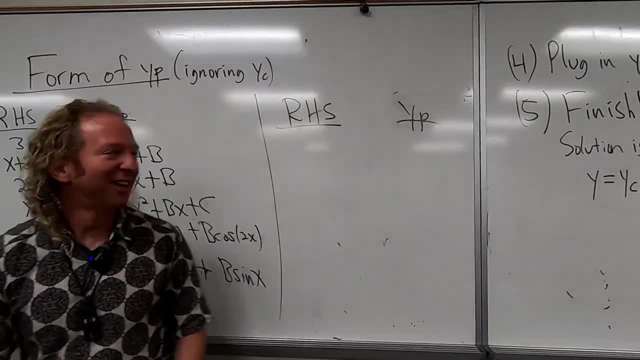 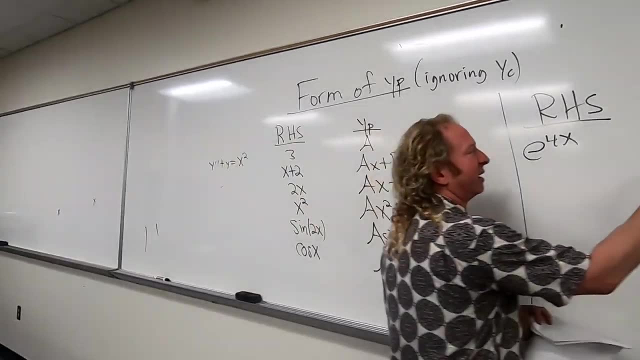 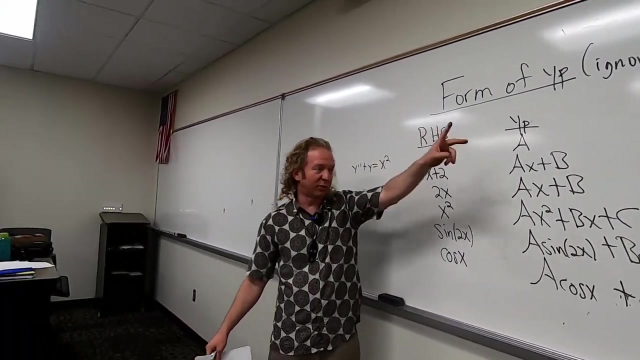 It's just back back, focus RHS. So, oh, what if we have an E? E to the 4X, Then you just put A E to the 4X. Okay, Recap, Recap, So you have number. 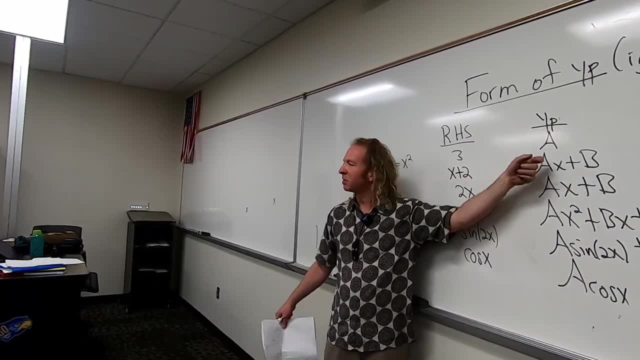 We're going to keep going. But you have a number, you get A. You have a linear. You have to have AX plus B. You have just 2X. You still need the full linear. You have X squared. You still need the full quadratic. 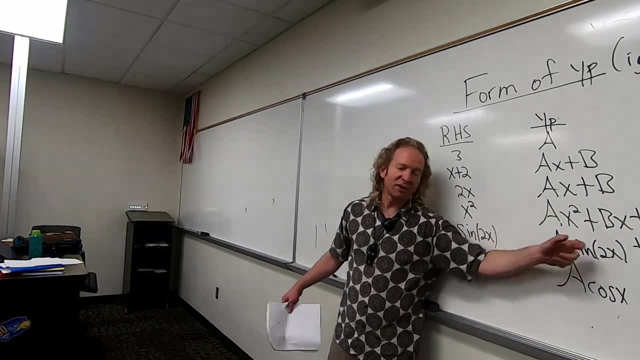 I put a plus 1 here. It's still the full quadratic. When you have a sine, you have to have a sine and a cosine. You have a cosine, you have to have a cosine and a sine. You have an E, you have that. 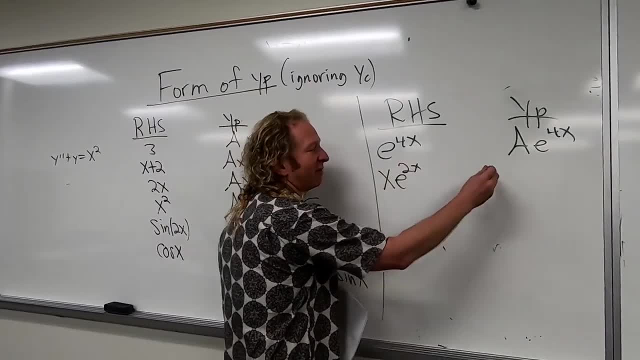 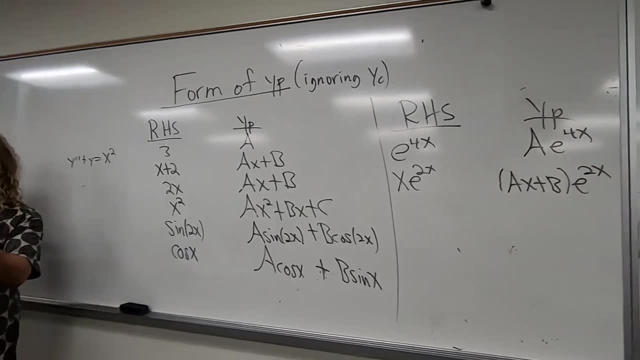 What if you have X, E to the 2X? Well then, you have to have the linear times, the E. Okay, Times the E. You multiply it. You multiply it by the E. Okay, That's it, Yeah. 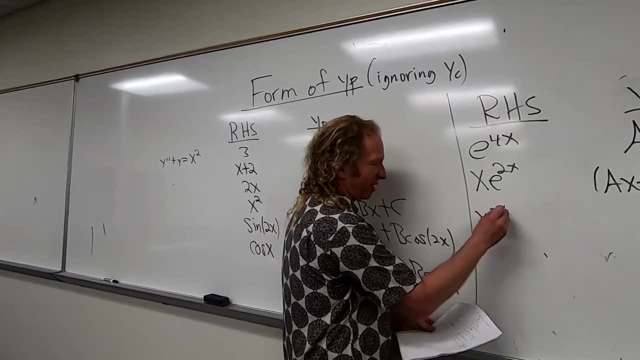 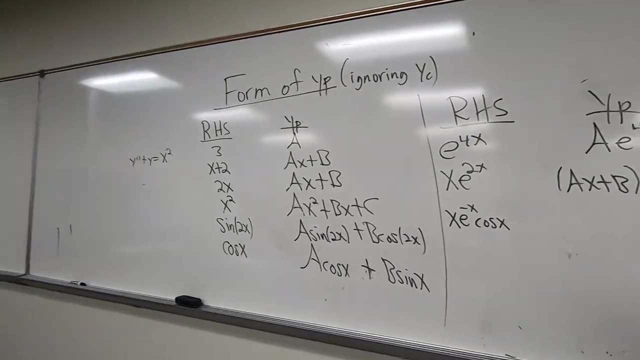 What if you had- Let's go nuts? What if you have X? E to the negative X, cosine X? Then you give up? No, Don't give up. Drop out of college. No, Don't do that, No. 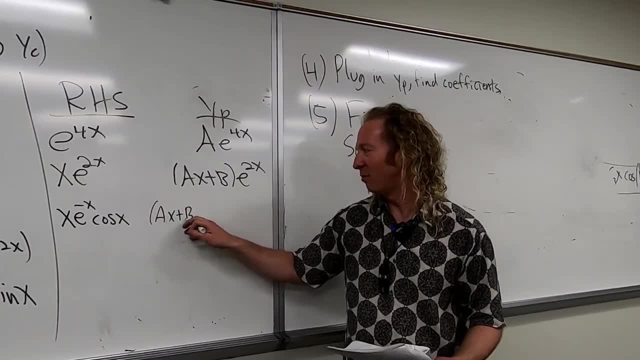 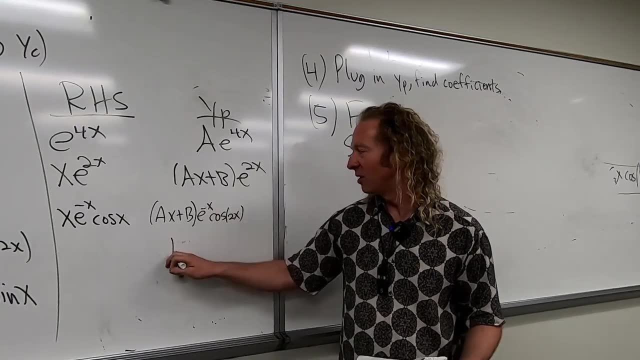 I always say that because I had a friend who told his class that He had a breakdown, And he told this girl that she should drop out of college. Well, the whole class, So AX plus B. He didn't get fired, though. 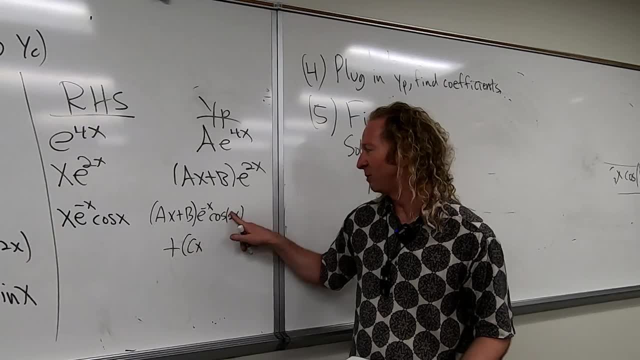 AX plus B. Why is it cosine 2X? It should be an X. Oh, I was thinking about that guy And I messed up. It's his fault. E to the negative, X sine X. Thank you, Rafael, right. 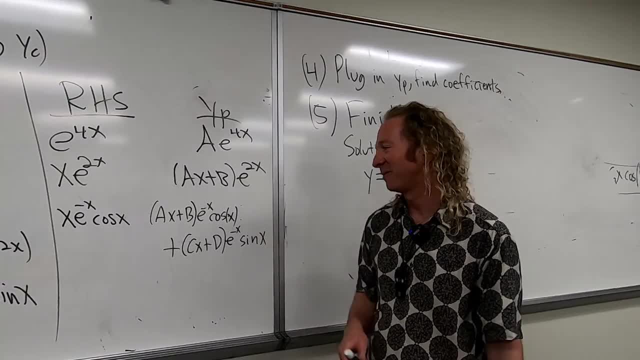 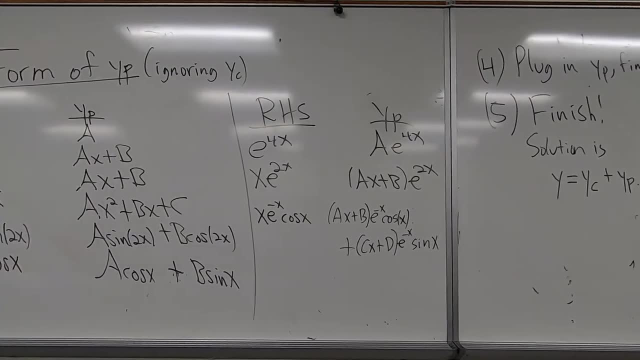 Was it you or was it the whole? I think it was the whole class. Okay, All right, Got it. See me after class. No, I'm kidding, I'm so bad I'm messing around, I'm just I'm kidding. 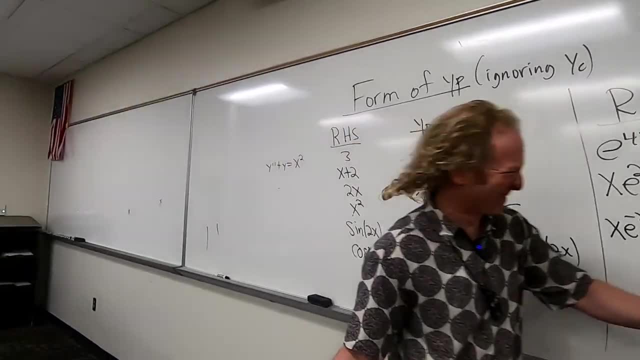 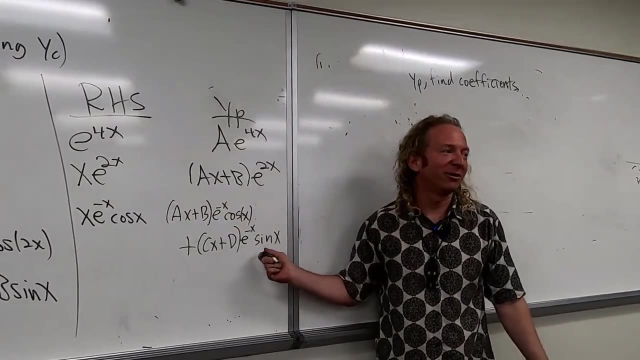 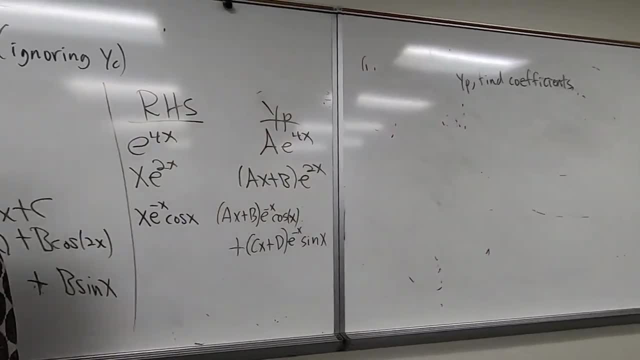 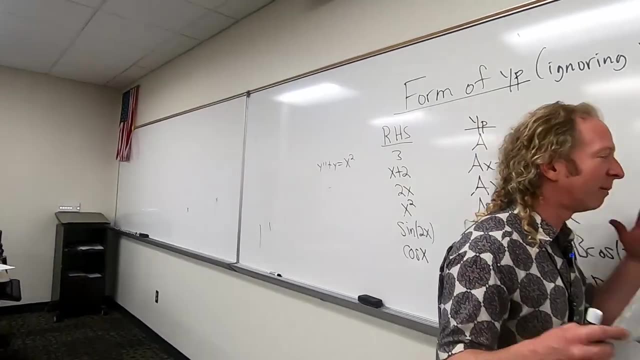 Now my friend. He used to teach a class. It was 8 AM everyday And every day they had homework and it was due the next day. So homework is due every day, Yeah, And it was a really bad class. It was like people who came from bad backgrounds and there was a program and it gave them. 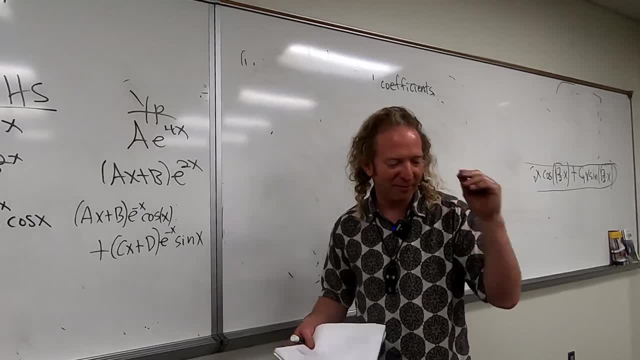 a chance to go to like a good school for free and they had like private counseling and all this stuff And this girl: every day she would say what's due tomorrow And he'd say, oh, it's on the syllabus. 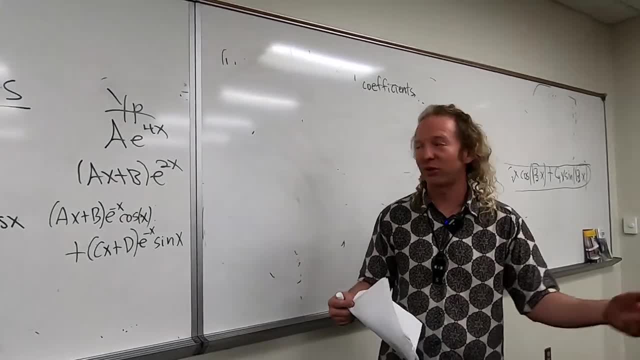 And the class was really loud, They would not stop talking. Like it was really rough. I used to teach one of those classes. It was so hard. This guy threatened me once. Anyways, it was really tough And then one day he just couldn't take it. 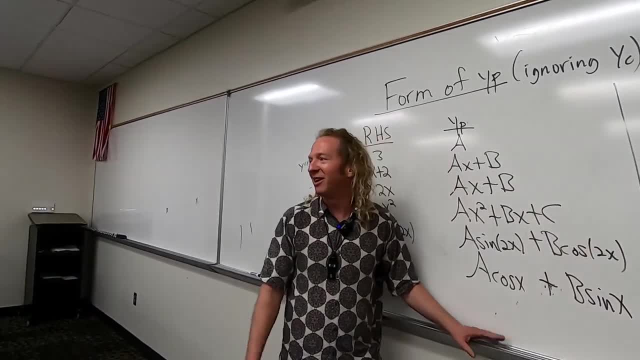 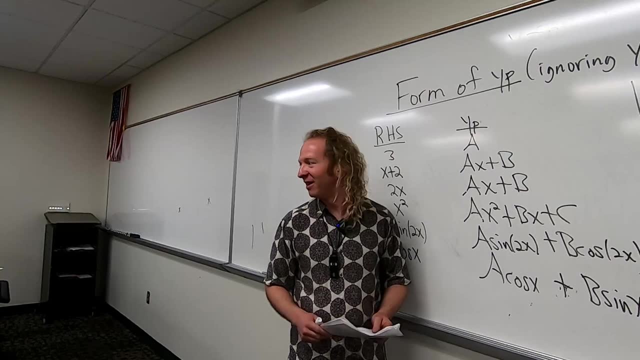 He's like it's on the syllabus, you stupid. And he started cussing and yeah, And the whole class went and they complained, but nothing happened to him, So he just had a mental breakdown. Yeah, he's, yeah. 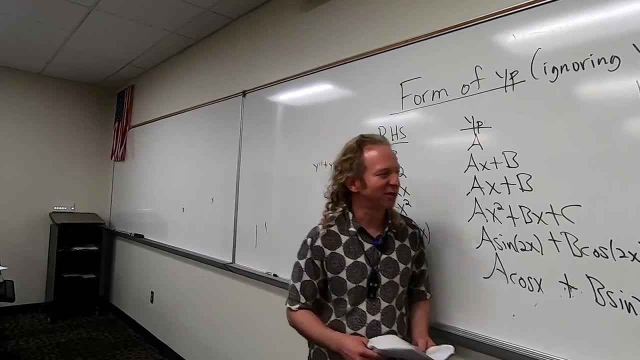 I mean, it was his second try at grad school. Like you know, he already had a master's. You know he was. he had a mental breakdown. Yeah, mm-hmm, yeah, All I know is he was from California. 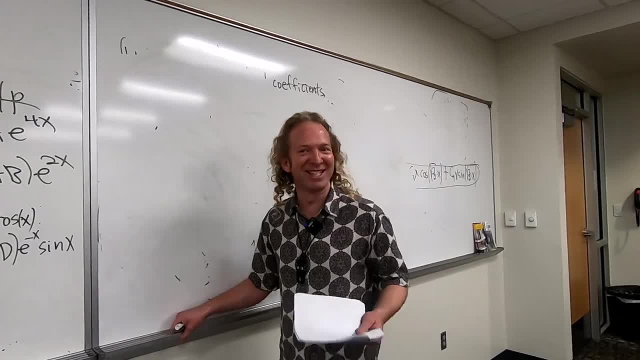 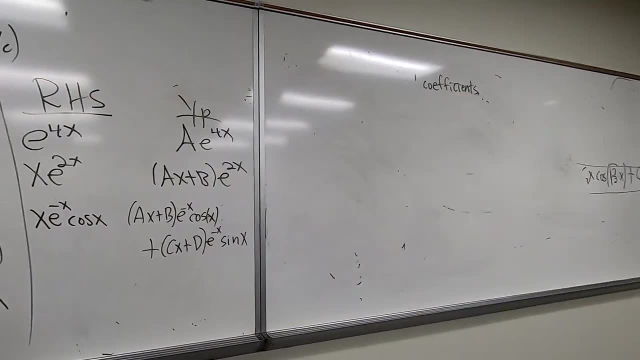 and he liked eating chips. That's all I remember. That's all I remember. Chips and salsa. He was really big on that. He's like: I like chips and salsa. I'm like: all right, That's all I remember. 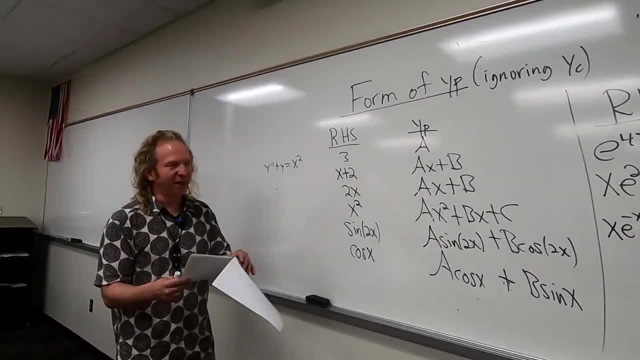 I don't even remember his name. I think I think we're good now. I think you want to take a break now and after the break we'll do the worksheet. So let's take a break. We will do all of these in class. 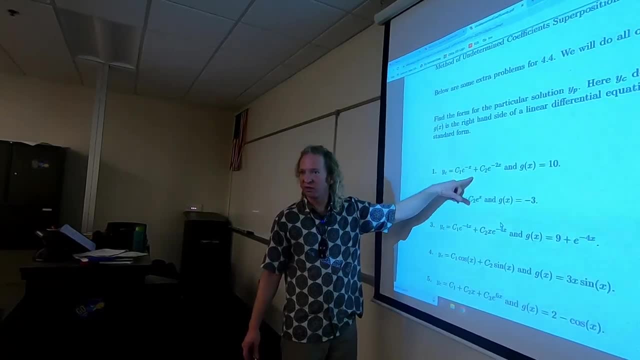 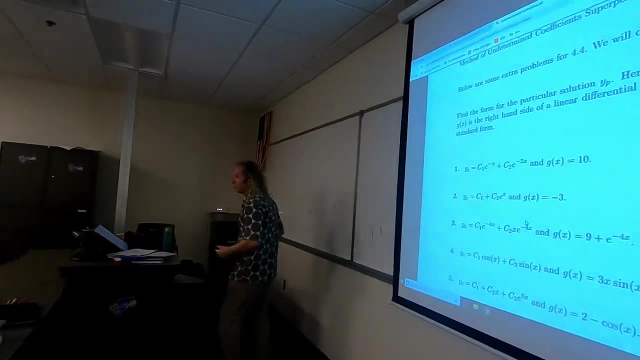 Find the form of the particular solution, YP. So here, YC is the answer you get to the DE, And then G is the right-hand side. okay, So let's do all of them and then we'll do a DE. 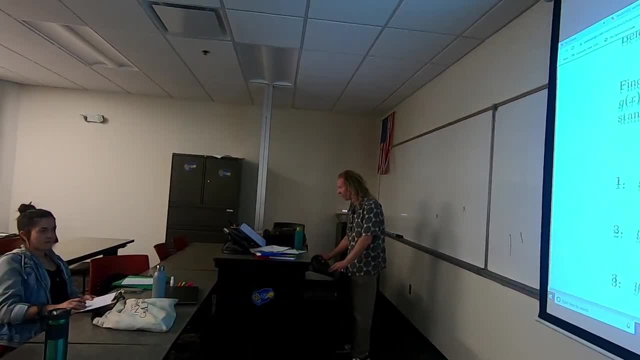 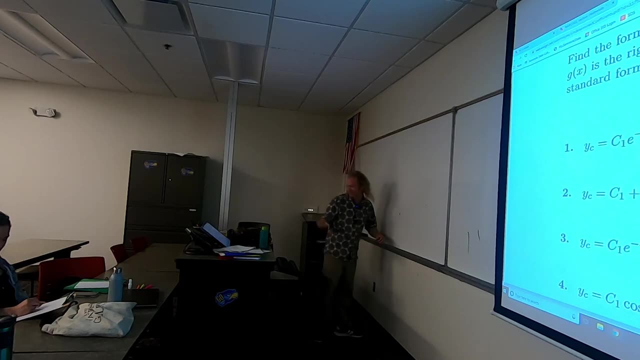 We'll do every single one. right now. I think I think we can do all of them. I know it's kind of dark so I'll write really big. So so number one: Gah, Number one. So number one is this. 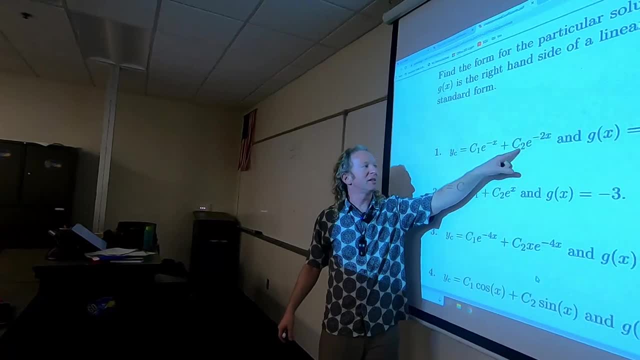 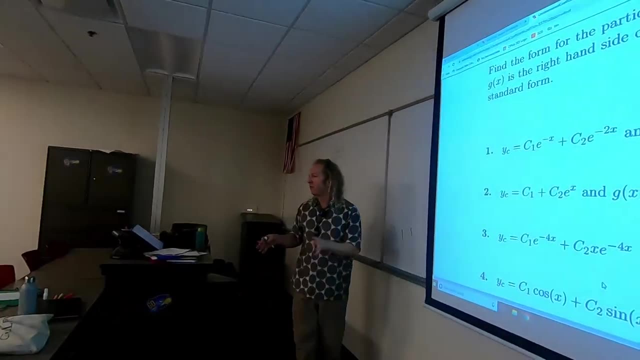 It's YC, C1, E to the negative X, C2, E to the negative- 2X. That's the homogeneous solution, and then there's our RHS, So I like to do these in steps. I don't know if this is the best way. 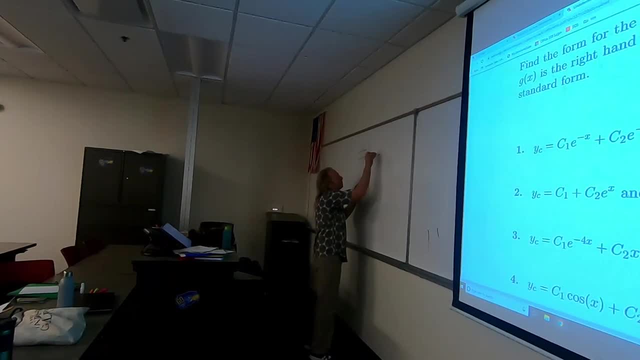 This is just how I do it. So I do two steps. I do initial and then I do modified. You don't have to show the steps You could. you could do it not in steps, It doesn't matter, I made this up. 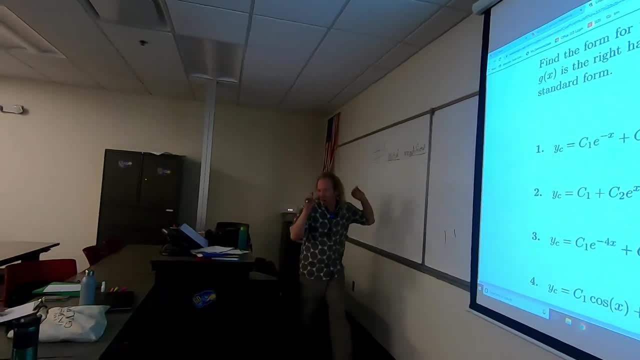 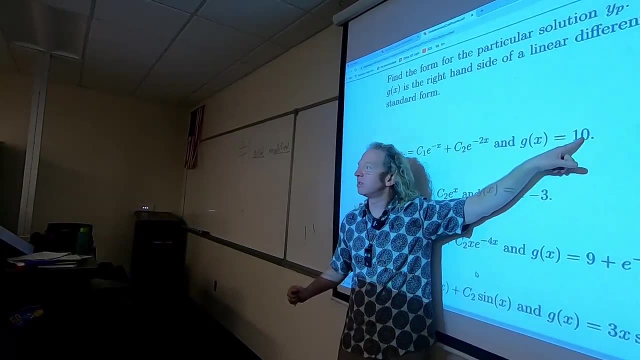 I don't know how other people do it. So when I do the initial, I only look at G. okay, So all you ignore, you have to ignore this. So just looking at this, at the 10,, what would your initial guess be? 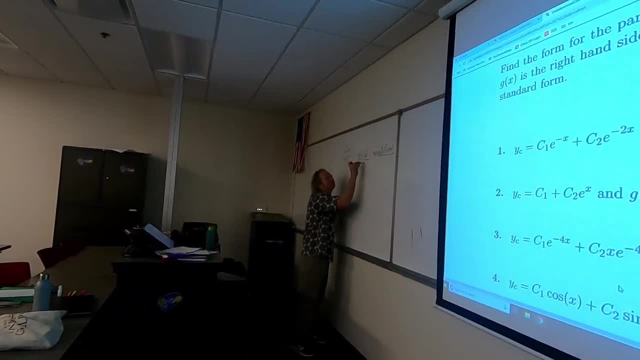 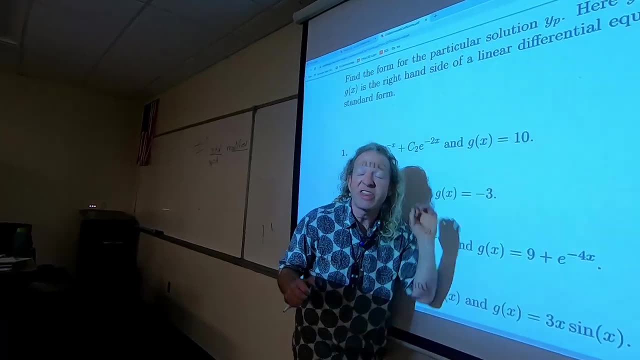 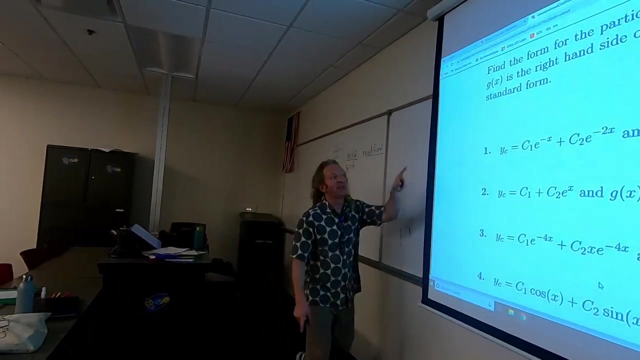 What would? what would A? So then I write down the initial. So, only looking at this, the initial guess is A. So just looking at this one, Then here's the key. So then you look at this and you look at these. okay, 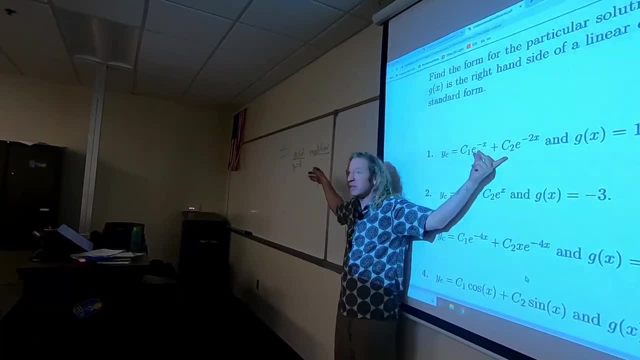 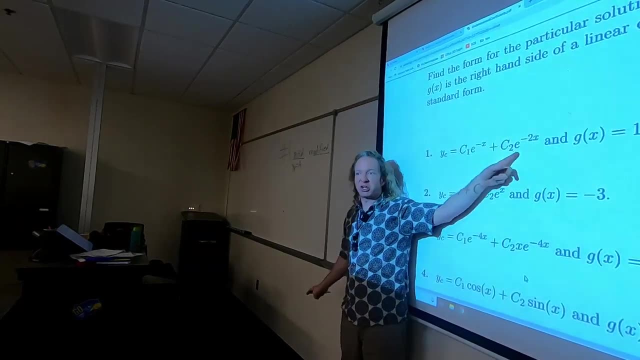 So at the A and at these. So you say, okay, is there repetition between A and these? Well, no right, Because A is a constant And these are exponential terms, So there's no repetition, right, If it was like a C3 here by itself. 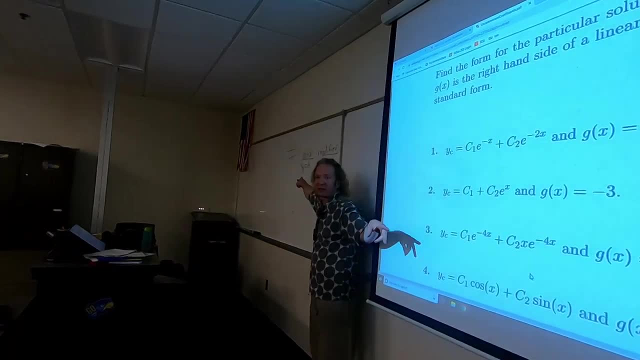 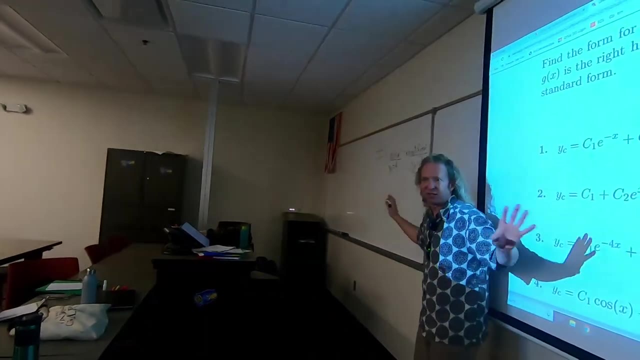 then those would both be constant terms, And then you would multiply this by X. But it's not So, we're done. That's the answer. So YP equals A, So there's no repetition. We're done, That's it. 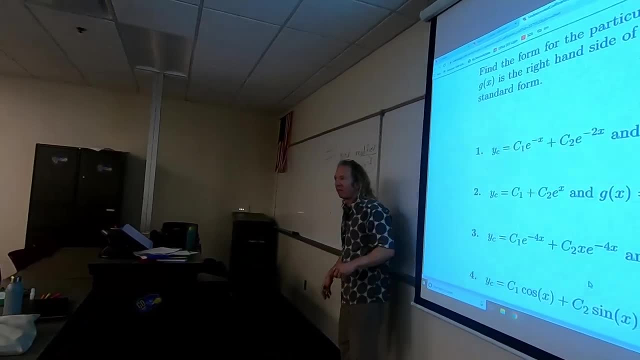 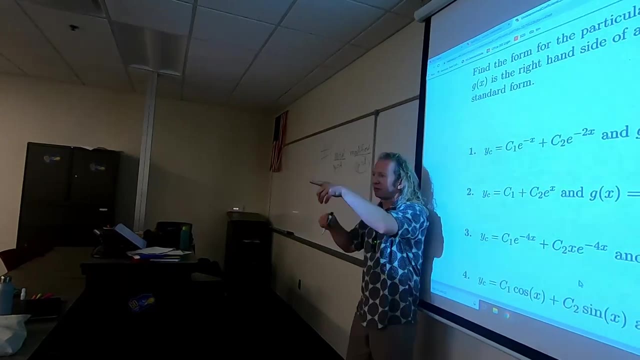 Let's do another one so you see how it works The more we do. yeah, Are you going to be posting this video? I don't know if it's going to record, okay, But if it does, I will. But I think there's already one there on the playlist, I think. 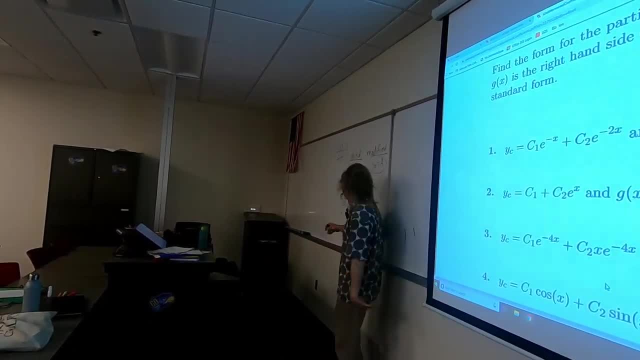 But I'll try If it does, if it posts, okay it's fine. It's really hard because it doesn't see over here. Two: this is confusing. This is like really this is all considered tricky. So two, I'm just going to put init. 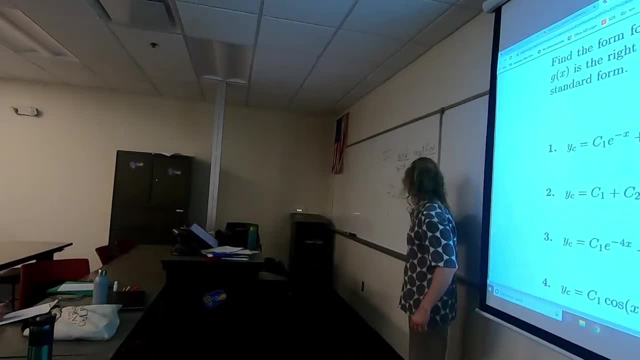 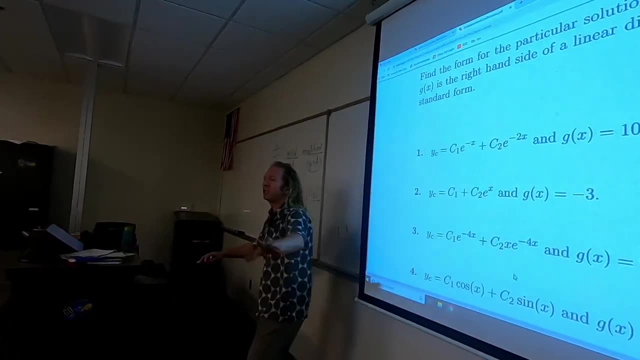 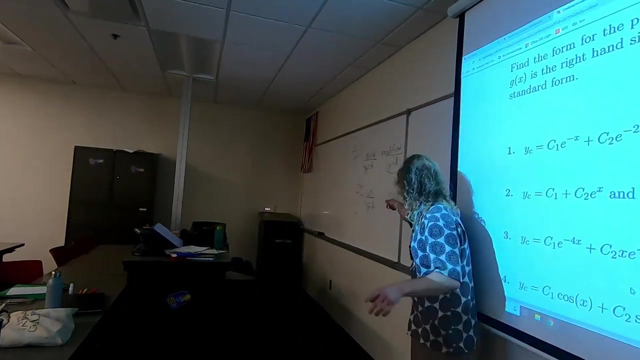 Init mod- Sorry, I'm making up abbreviations- Init mod, Command go. So for the initial, we only look at the number. So what would the initial be in this case? A? Okay, So now we have to look at A and the terms of YC. 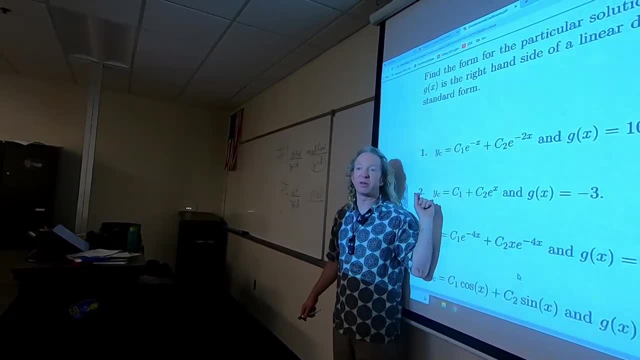 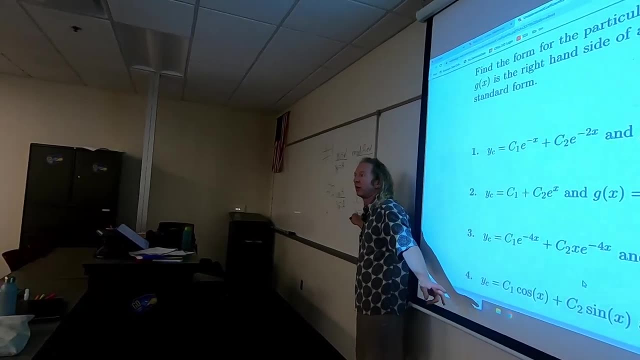 So is there repetition this time? Yes, Yes, with which term? C1. With the C1.. Yeah, there's repetition between the C1 and the A. So for the mod, we have to multiply it by what, do you think? 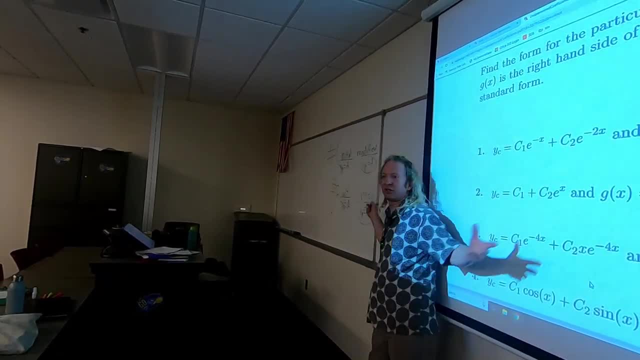 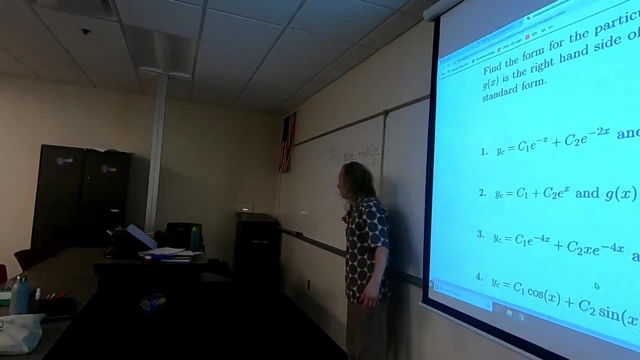 By X, By X. That would be it. Now there's no repetition. So that's it. Sneaky right, Sneaky. Explain that again. Okay, so this A repeats with this C1 because they're both constant terms. 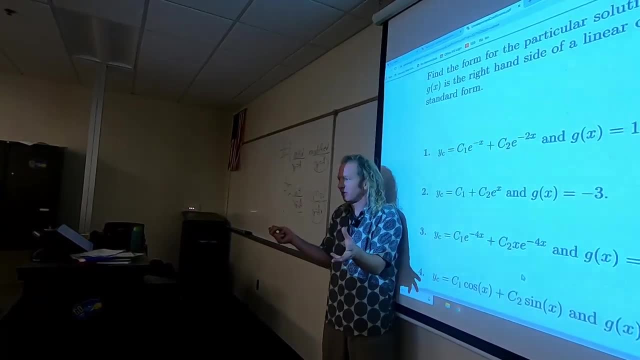 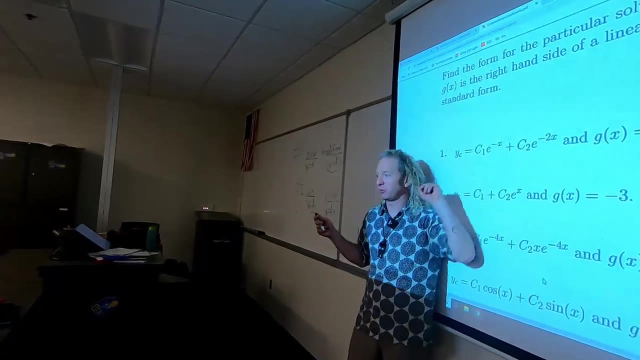 So they're the same right, They're both constants. So you can't have that, So you have to multiply by X. You can't have a constant because it's not by itself, Because there's E, they're exponential terms. 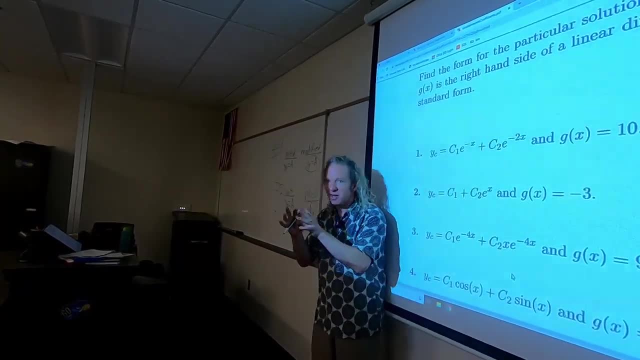 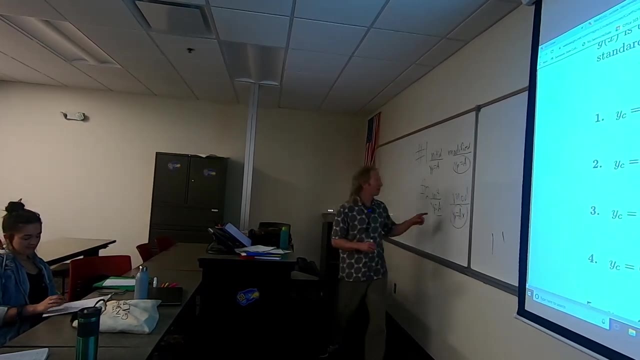 They're considered exponential terms because they have an E Right. it's not a constant by itself. Good, And how? why do you rewrite it as AX? Because you want to make them. the reason is you want to make the solutions linearly independent. 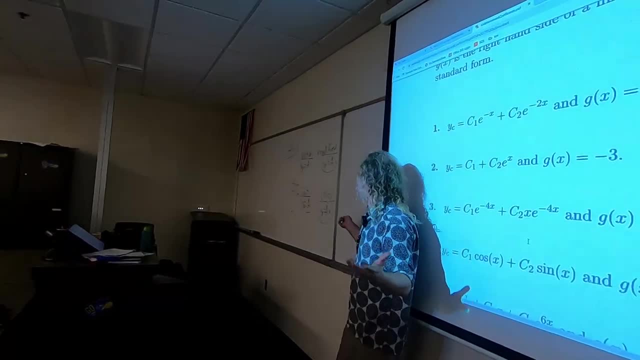 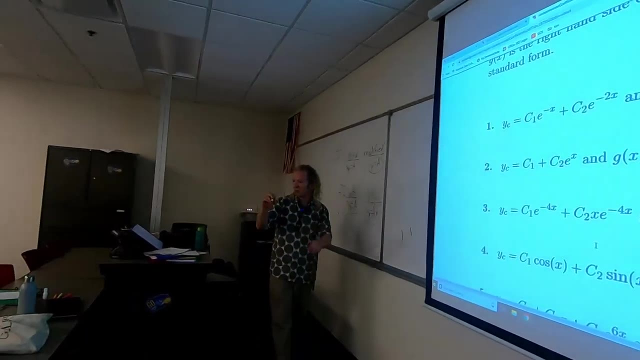 That's why you can't have repetition, That's why, So, basically, you have to eliminate the repetition by multiplying by X, Just like before. Remember before, when we were multiplying by X, when we had repetition With the E, with the the same thing. 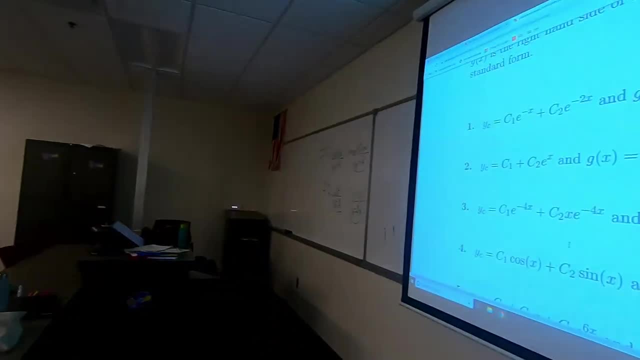 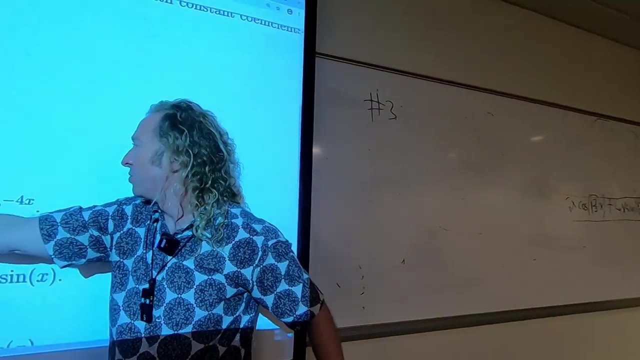 Let's do three. I'll do it over here. Three, I'll write big Three. So for three we have this here. So there's our G, So let's do our in it. So nine plus E to the 4X. 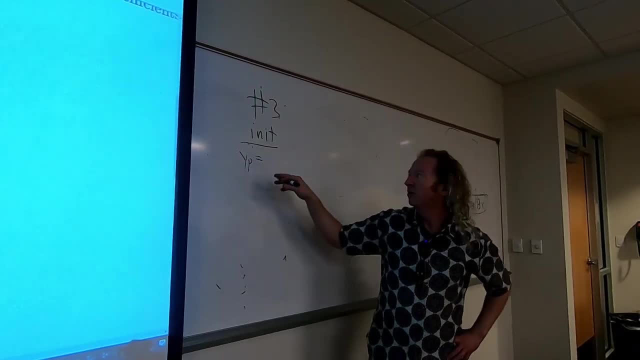 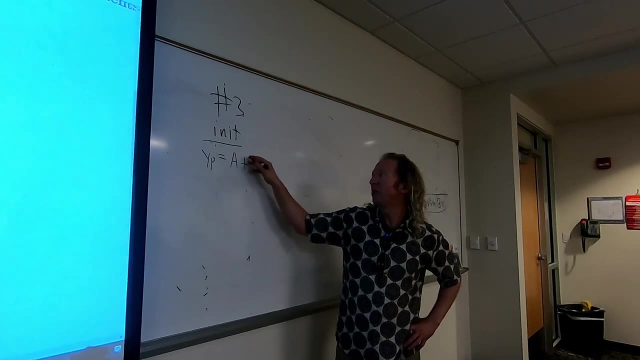 So our YP, our YP. So for the nine, we're going to get an A, And for the E to the negative 4X, we just get B E to the negative 4X. See how we got that. 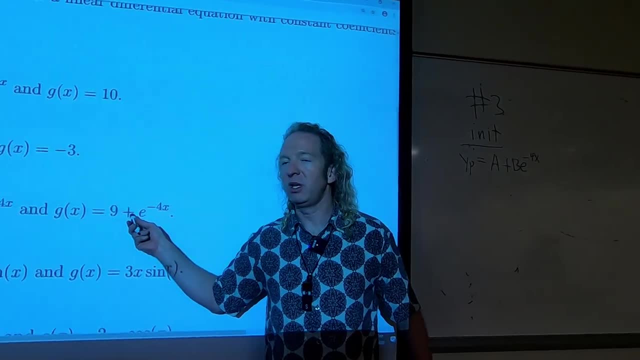 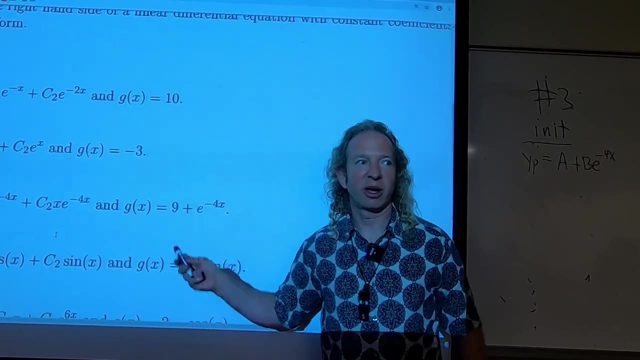 So the nine gives you an A And this one gives you B E to the negative 4X. Right A, B E to the negative 4X. Okay, Now the mod. Okay, the mod. This is tricky. 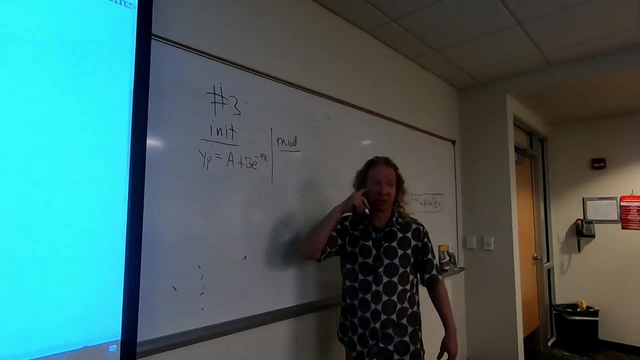 Please ask if you have questions. There's a bunch of these, So we're going to go through all like 11 of these or something. It's ridiculous. You get really good at it. This is like 40 points on your test. 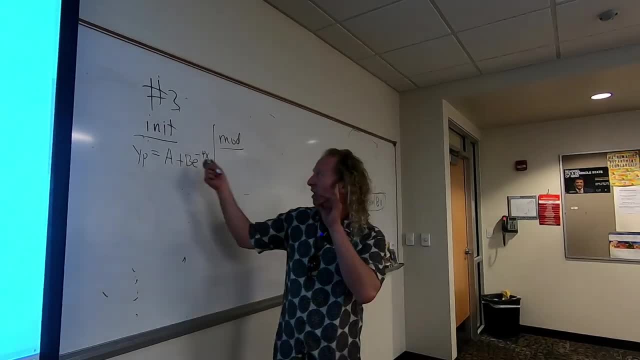 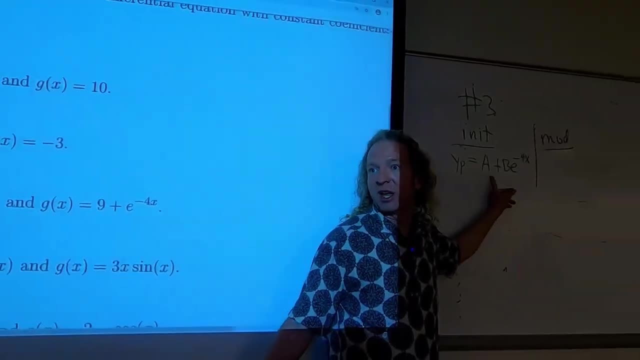 So it's like Mod: Okay, So we look here And we only look here. So let's see. So these are two separate guesses, So they're two separate thought processes. Okay, So for A. So is the repetition with the A. 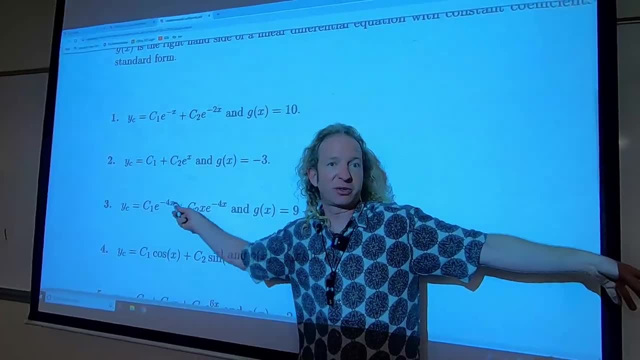 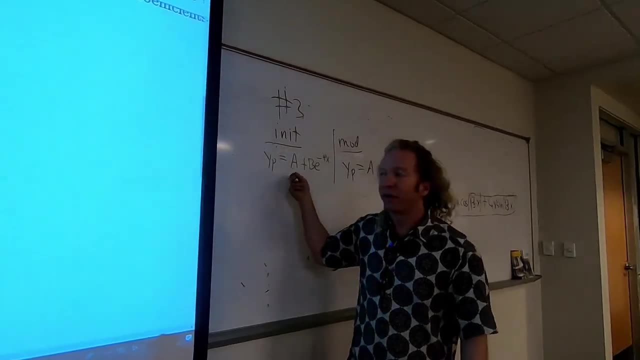 No, No, There's not Right, Because these are exponentials, Right, So the A stays the same, Right. A does not repeat with these, Right? These are not constant terms, Right, So we're good, All right. 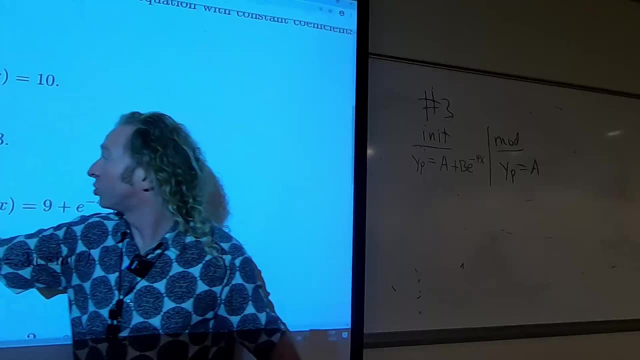 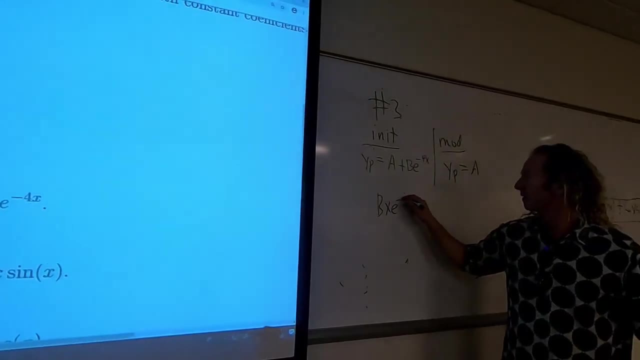 So A to the negative 4x: Yeah, Just on the first one. On the first one, Yeah, On the first one. So watch this. This is where the magic happens. So let's say I put an x, there Is the repetition still. 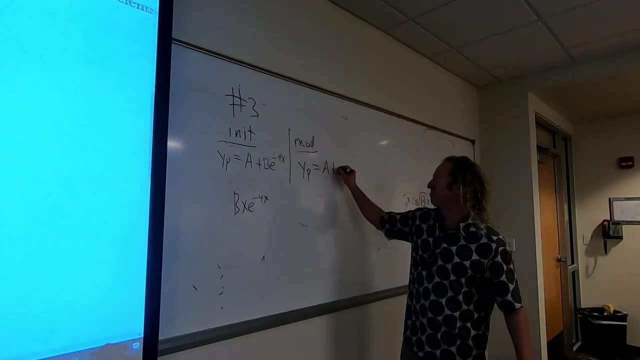 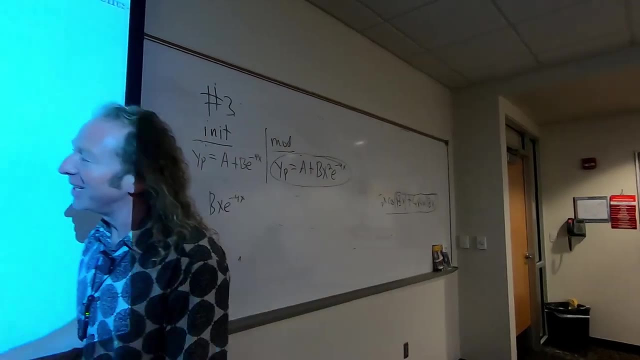 Yeah. So what do you have to do, Do you think? Put it: Yeah, X squared, X squared, Yeah, Hardcore, Right, No joke, Right, It's really sneaky. So this one Putting out the wrong thing. 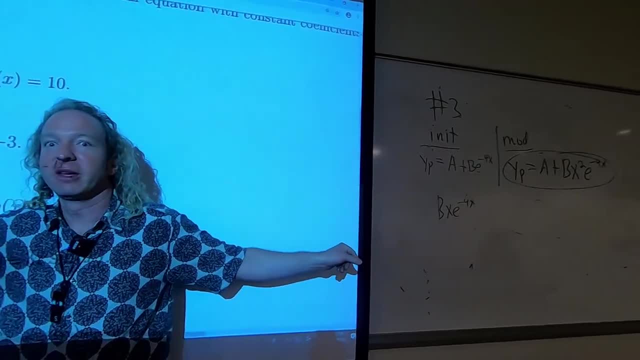 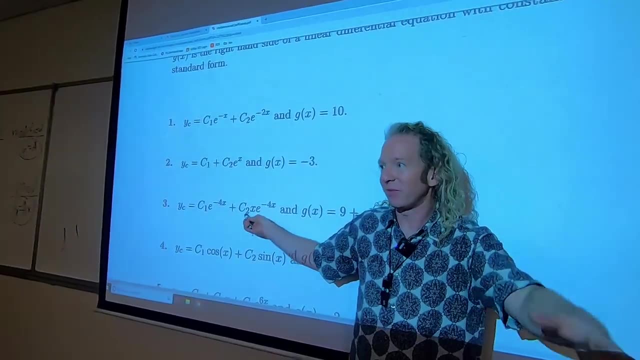 So this one, Right With this one. So you have to put an x. But if you put an x, That's not enough Because of the one that said: put an x squared Right, So sneaky They're the same. 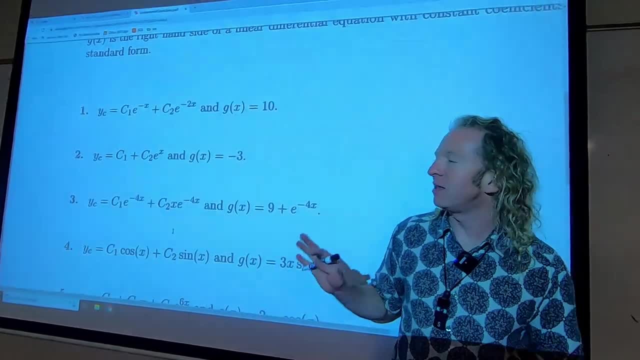 Because they're the same, You want them to be different. Yeah, If you try to make these up, You say: well, what if it was this, Or what if it was that? Sometimes you run into situations that you can't do. The reason is: 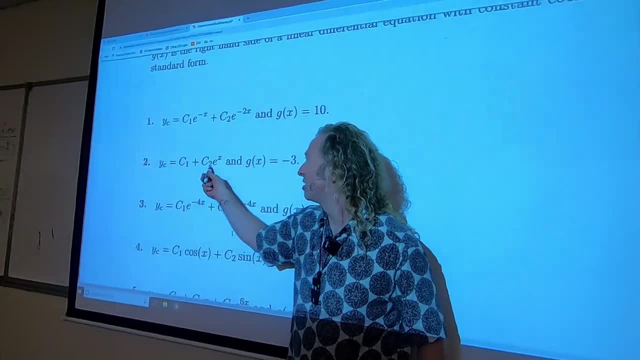 These actually have to be solutions to DEs. Actually, in this case, This is No. no, It could be a solution to a DE, Never mind. But like, if you start making them up, You come up with stuff that you can't actually do. 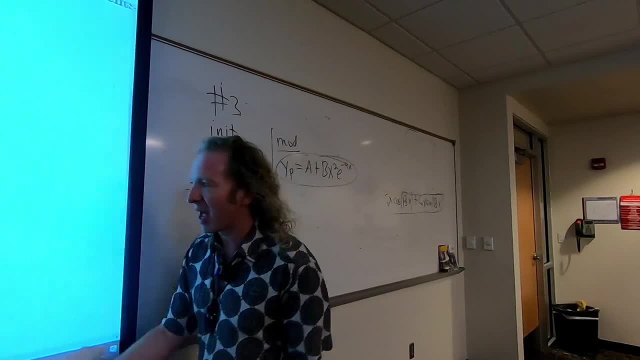 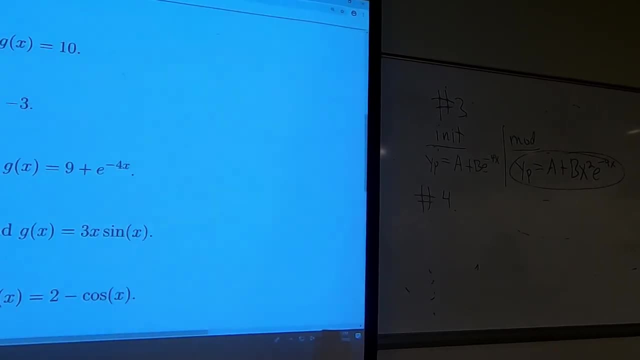 That's because These are actually solutions to DEs, So It has to make sense. Four: Four is the hardest one I'm going to see. Maybe I can make it bigger, So you can, Can you make it bigger? 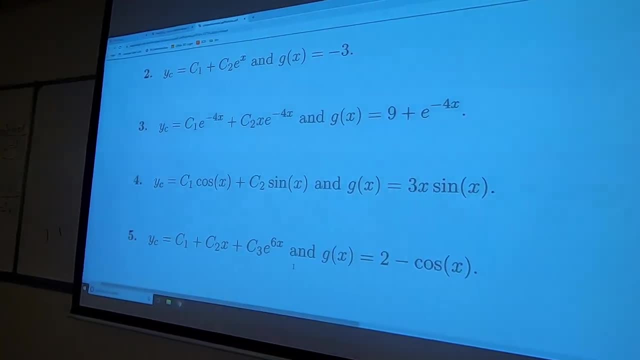 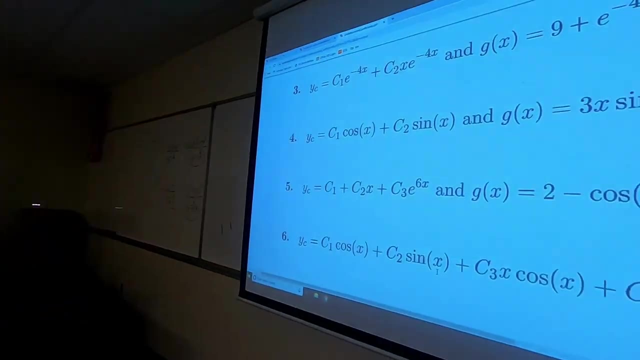 Let's see, That's a little bit better. That's a little bit better. Let's do four, Four, Okay, Four is really tricky. I'm going to do four here, So Looking, So in it We're saving time. 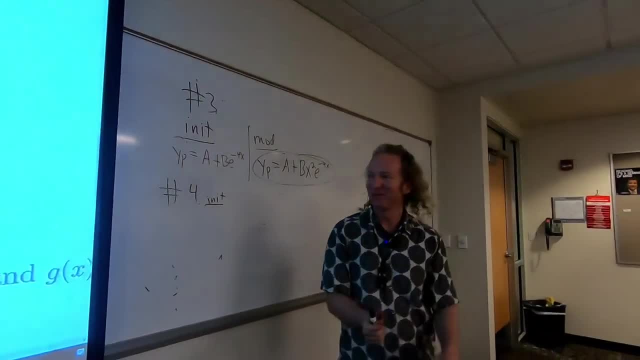 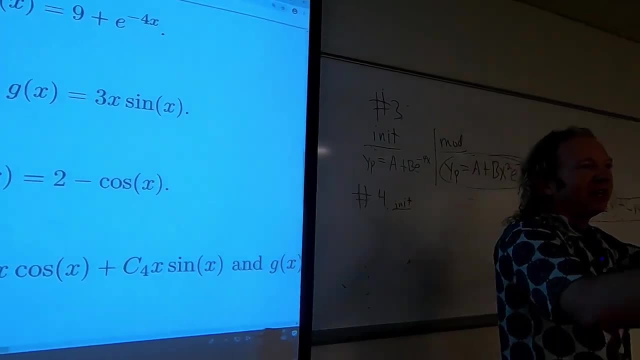 Because I'm not writing the question down. That's saving like An extra five minutes. That's fine Time. So it has a full linear and a sine. So we have to have the full linear and the sine And the full linear. 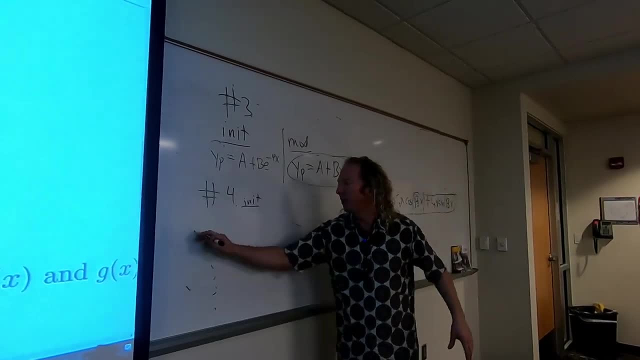 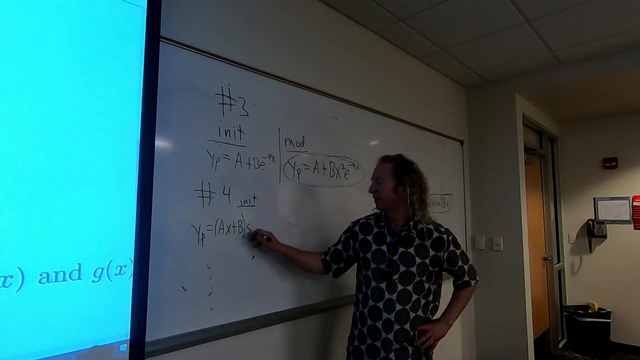 And the cosine, Yeah, Both. So the in it will be Very good. YP equals AX plus B Sine X. This is the hardest, One of the hardest ones, If not the hardest. Plus This comes up in the homework. 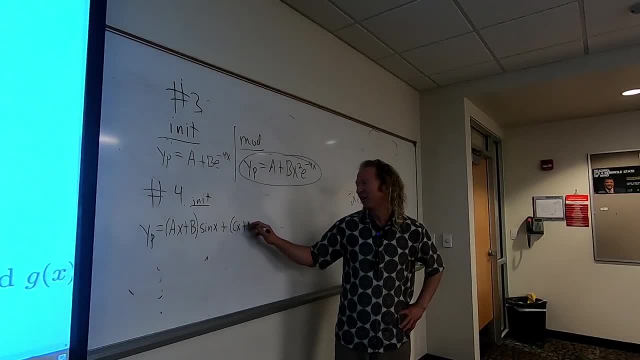 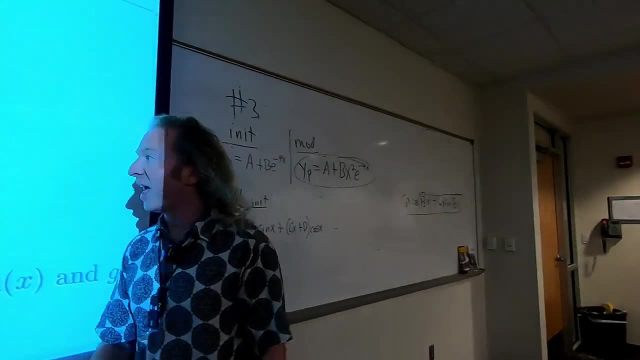 Except you have to actually solve the DE. It's ridiculous Like It takes. I mean It's like 30 minute problem. The first time I did this problem in the homework I did it wrong. I was in a hurry. 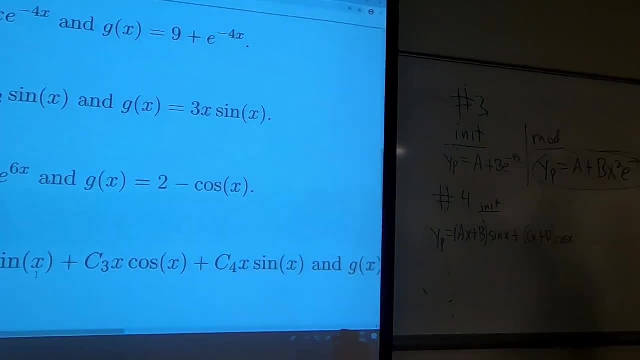 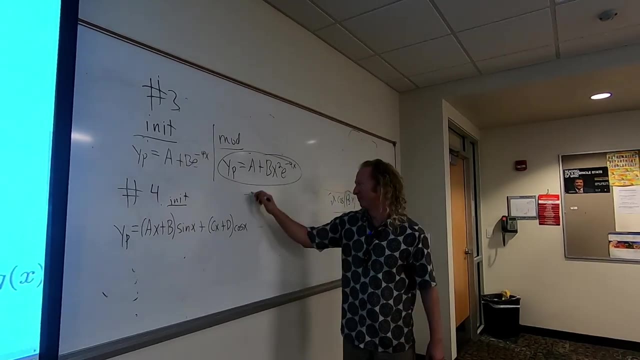 And It wasted an hour of my life. So I'll never forget it. Pain, So that's, That's the in it. That's the in it. What did I do wrong? I'll show you. So, mod, I did the mod wrong. 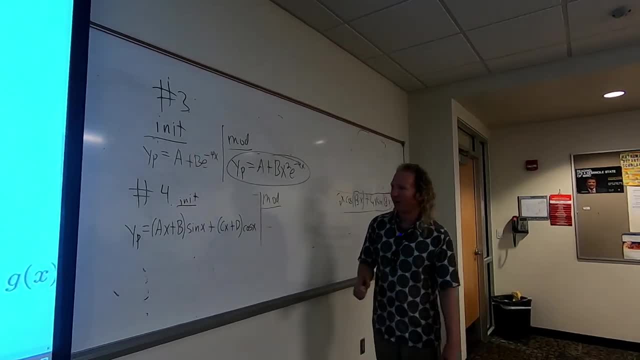 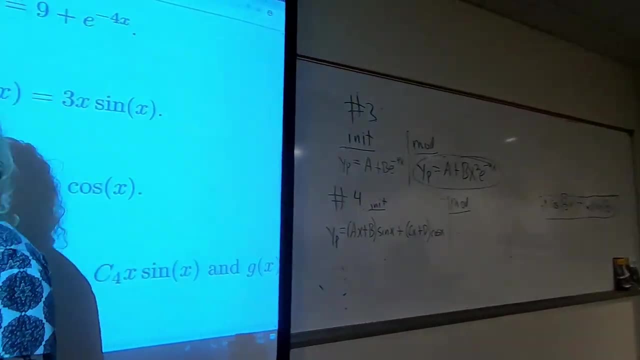 I was like, Oh, Let me just blow through the homework So I can watch TV. No, No, So now we have to look Here And here And see if there's repetition. Okay, So Is there repetition? 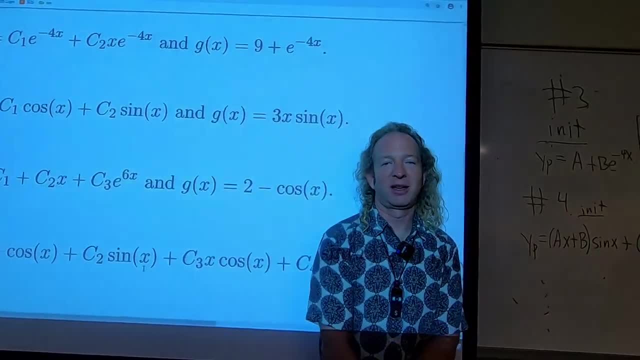 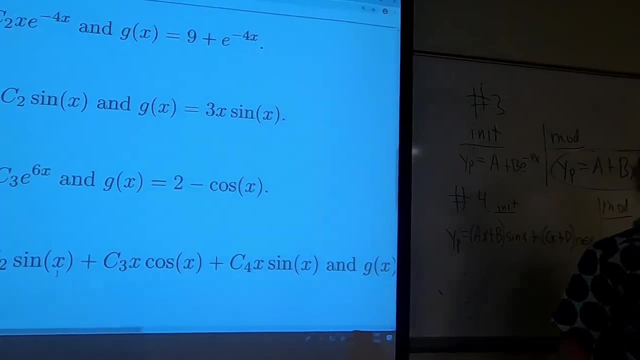 What do you think? Yes, Very good. You have to actually distribute it. Very good, Sarani, Sarani, B sine x Repeats With Sine x, Sneaky, Right, Sneaky, And D cosine x. 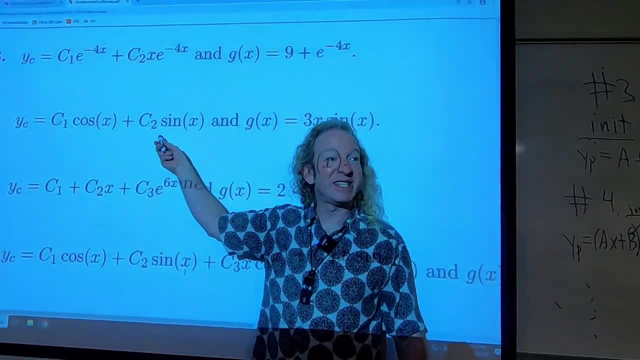 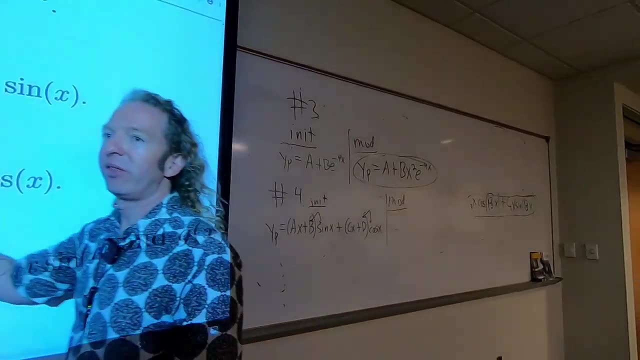 Repeats With Sine x. Sneaky, Right Sneaky. And D cosine x Repeats With Cosine x. So would you recommend we Multiply them? Yeah In your mind, Yeah Mentally. 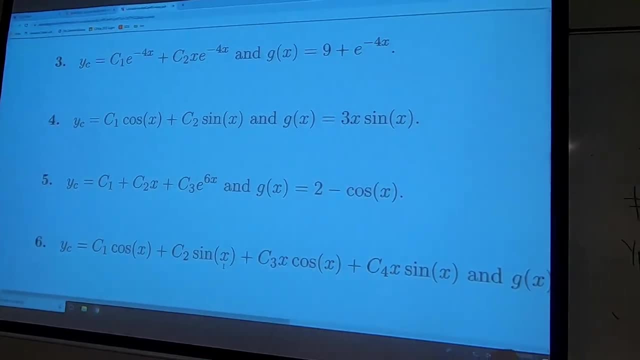 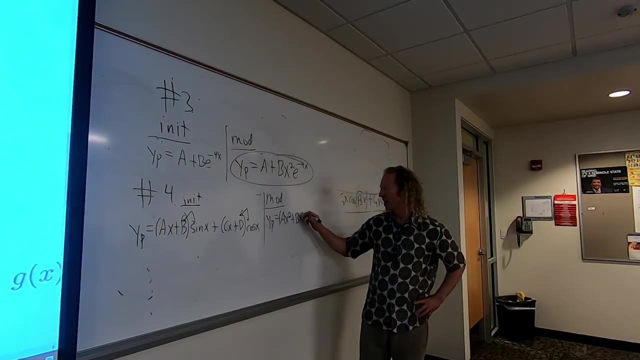 Yeah And so. So now For the mod. We have to multiply by x, So y p Would be A x squared Plus b x, Sine x Plus C x squared Plus d x. This is considered. 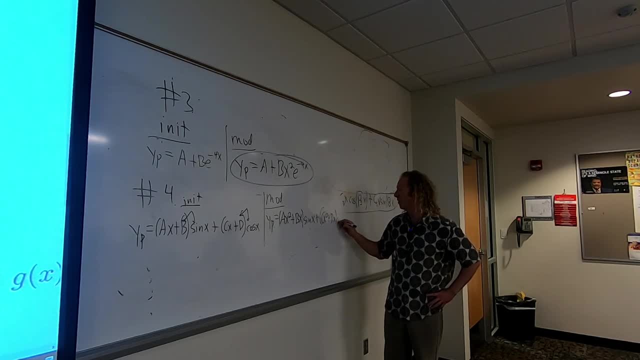 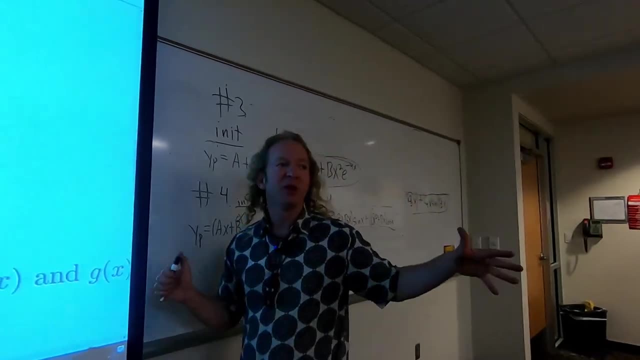 This is considered very tricky For people. People Have a hard. It doesn't always happen, They're not always tricky, But this, This, This. You have a homework problem Where You have one like this That you have to solve. 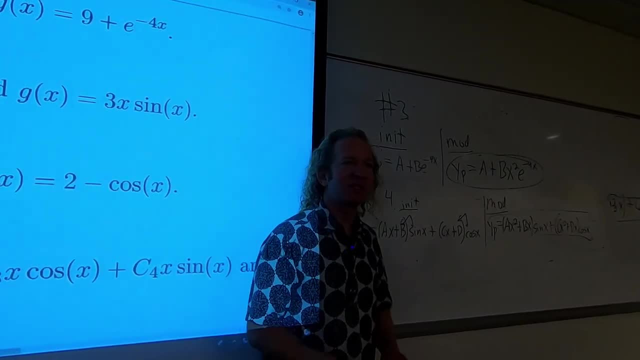 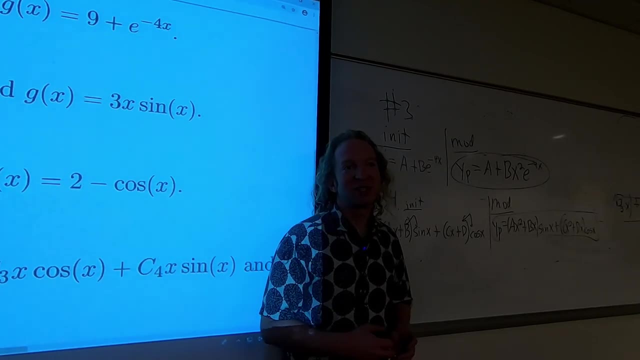 Yes, sir, Yes, Urosh. Is there any other way You could learn this? I think this is the easiest way. Why Does it make sense? None of it. What part, Urosh, I don't know like What you're referring to. 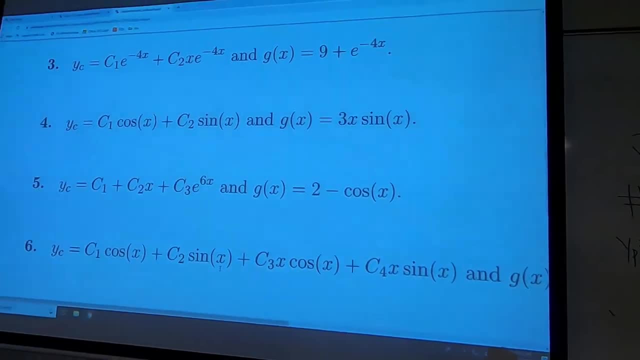 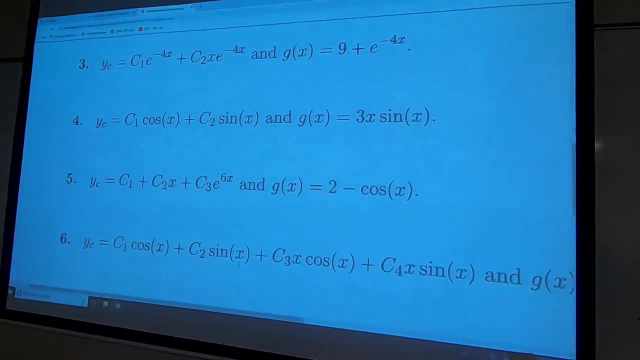 Well, okay, You want to go back to the beginning? The first one, Or Or just this one? Do the easiest. Well, let's do this one. So do you understand How to get the initial? No, Do you know how to get the initial? 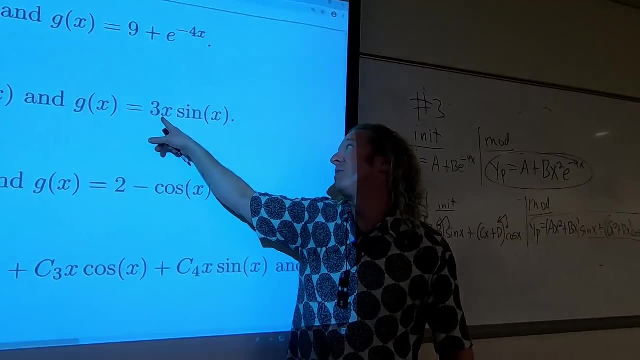 I know you look at the right side, But I don't know, I don't know the right side. Yes, Okay. So because it's three x, You have to have an a, x plus b, Okay. And because it's sine. 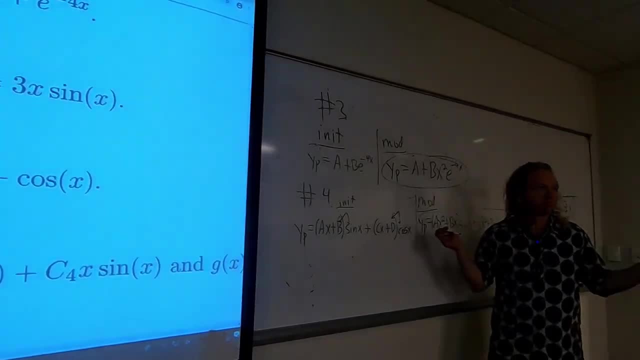 You have to have sine and cosine, So. So how do you know the split Between a x plus b? Because you have to have sine and cosine And they can't be the same letters. You can never have more than one. I think it's better off like: 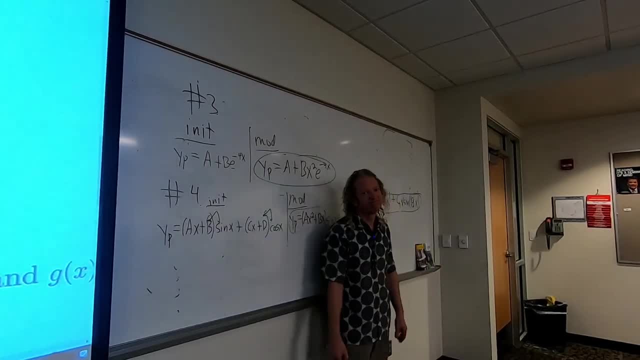 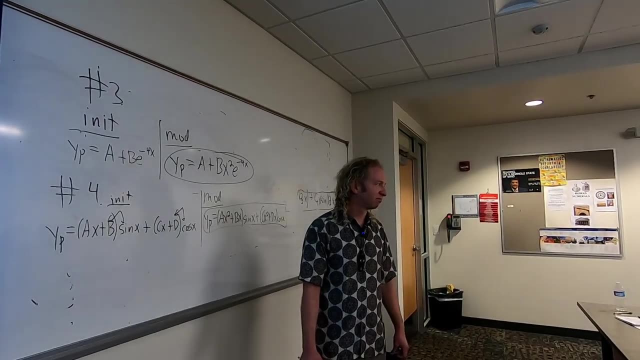 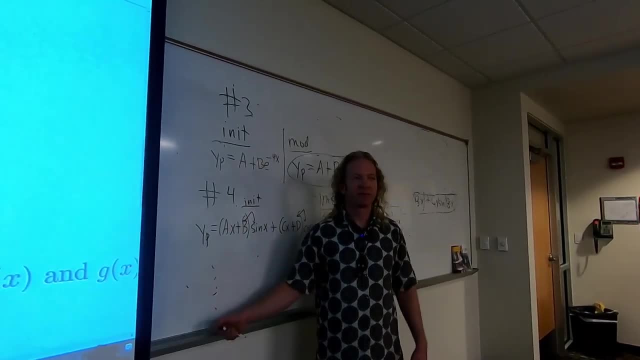 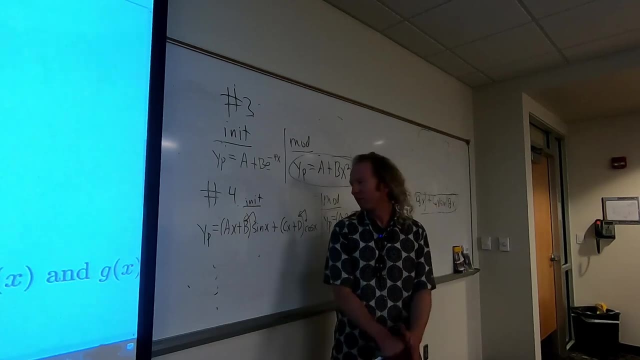 So Do. Do you know how to get the sine and cosine Now? No, Yeah, I forget why We just I'm going to get up to there. Oh, So you're going to get up to this, Yeah. 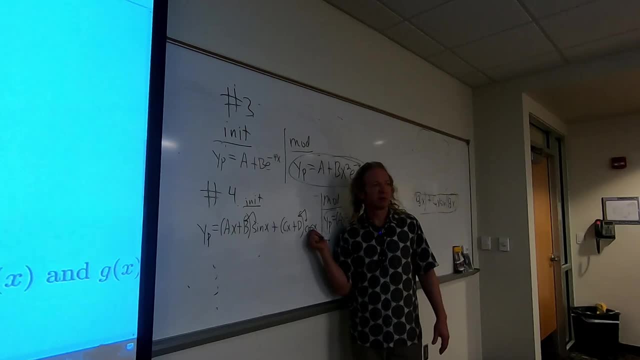 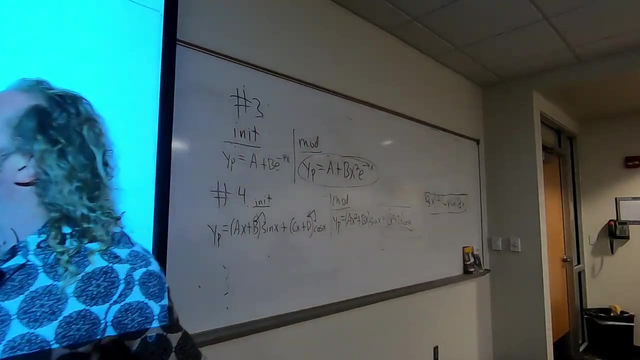 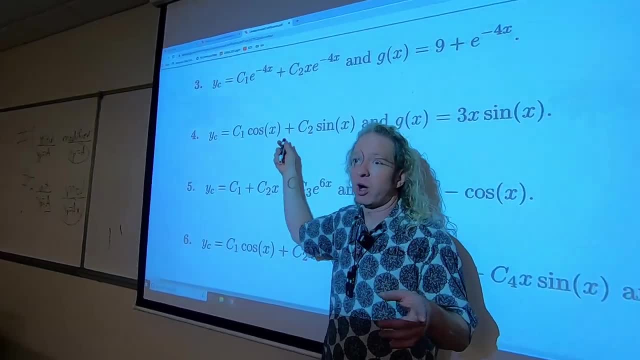 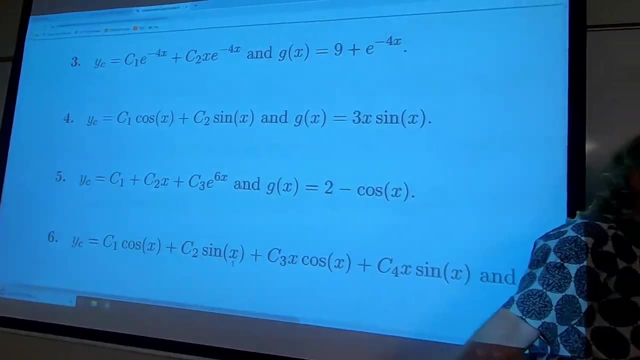 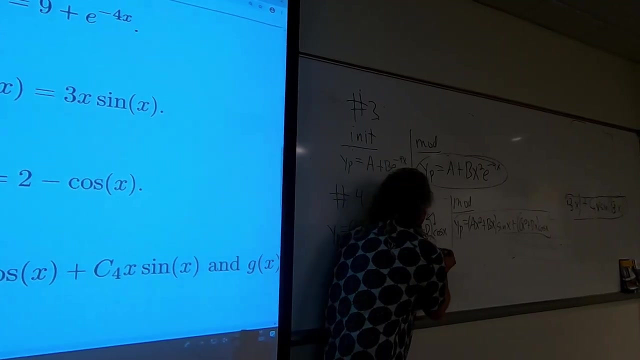 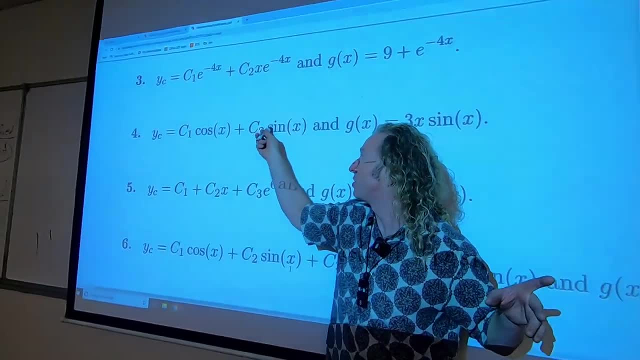 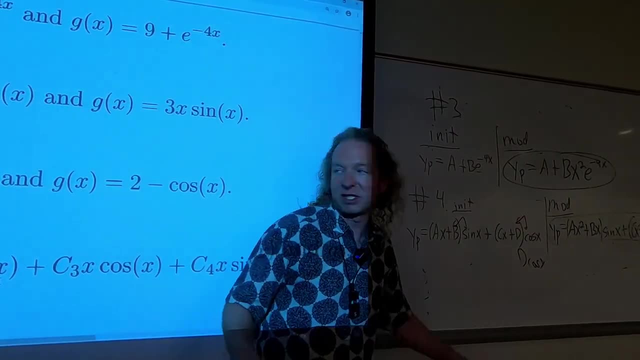 it's going to repeat with this one Same thing with sine right. Look sine Here. you would get b sine. So it repeats. No, you don't want the same thing If you go back to. let's go back to number three. It's still on the board. Here's number three. 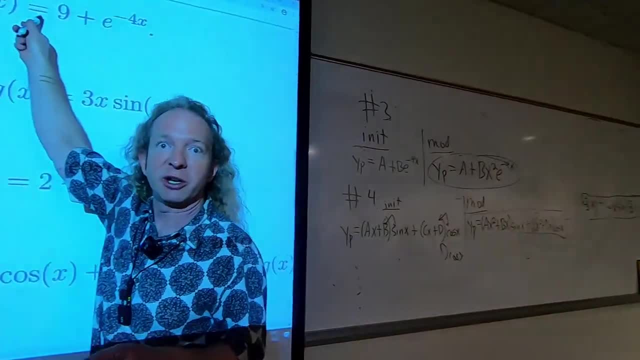 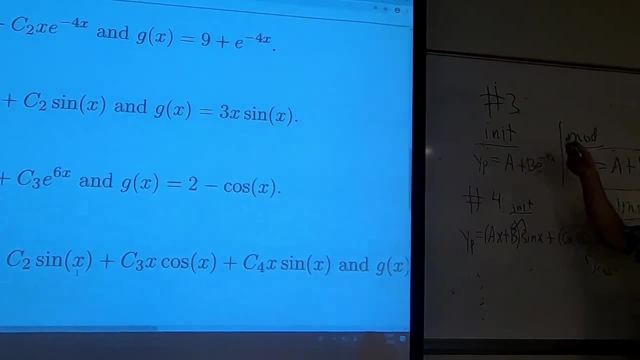 Look at number three really quick and we'll keep going. So number three, the initial, you look here. So for the nine it's a, For this one it's b, e to the negative: 4x, right, You see it Right here. Boom, Right, Okay, now. now Uta check it. 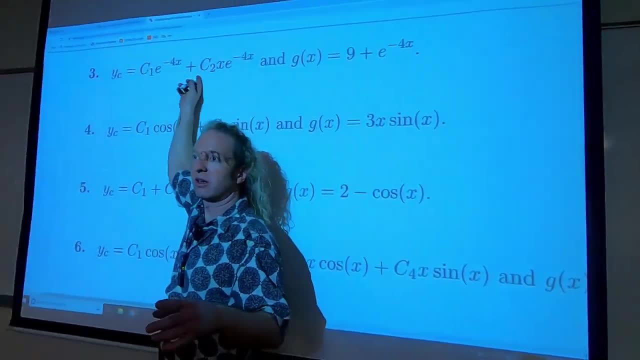 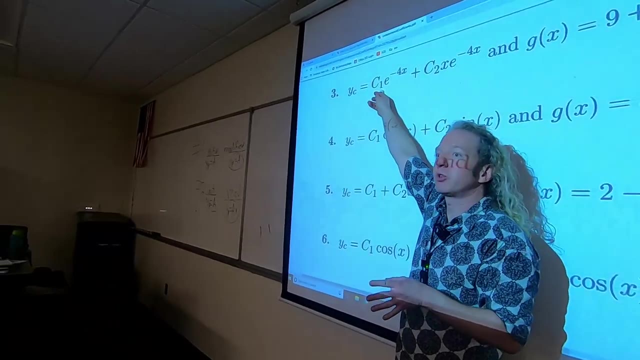 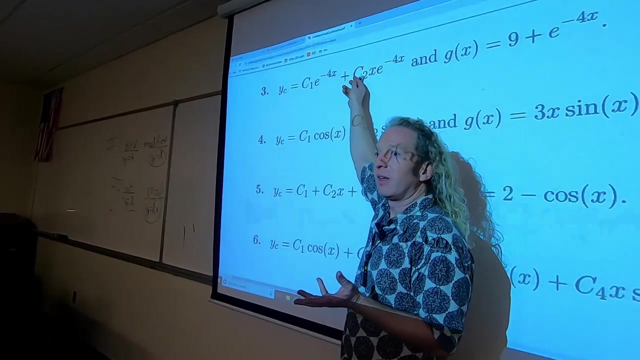 out A A Does a repeat with these? No, okay, Is this a constant term? No, It's an exponential term because there's what An e right, So it doesn't repeat. What about this one? Does it repeat? 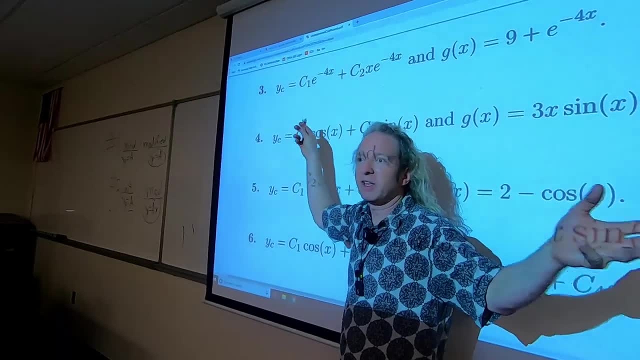 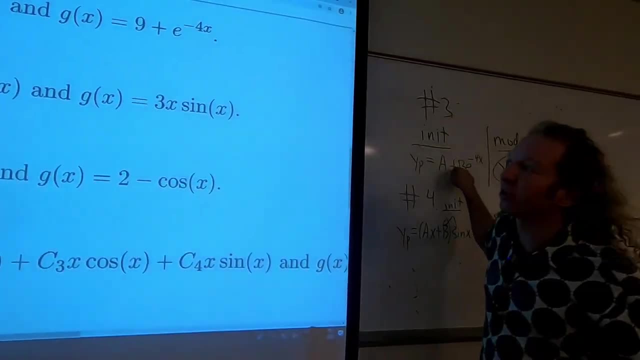 Okay, is this a constant term, So it doesn't repeat. If they're the same, it repeats. So watch this. So this one b: e to the negative 4x. This is an e to the negative 4x term. It repeats with this one, right, Do you see that? Okay, so you. 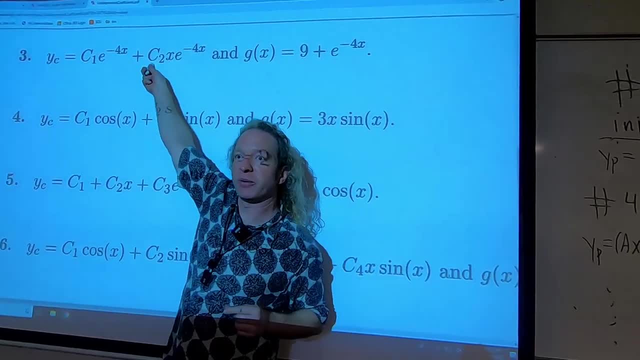 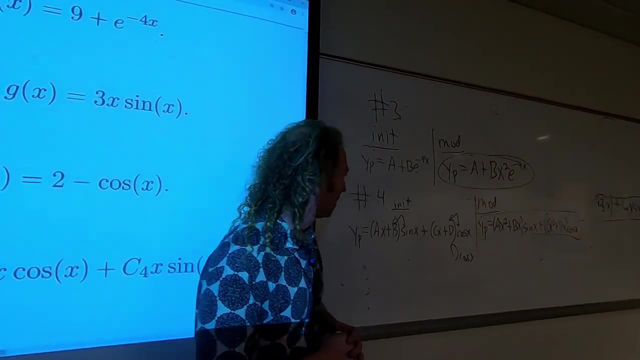 have to put an x. But if you put an x, it repeats with this one. So you have to put an x squared. So why don't you square the a x and the c x? It won't work if you just put an x here and an x here. It won't work. I've tried it. 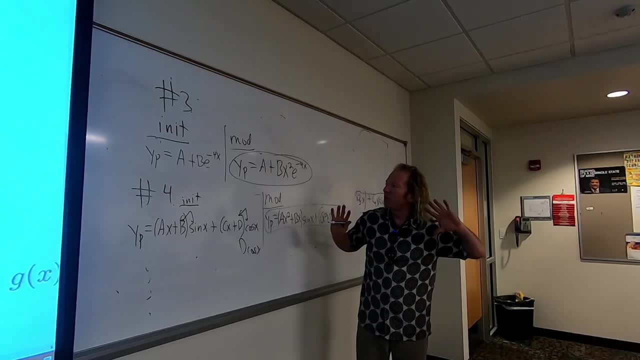 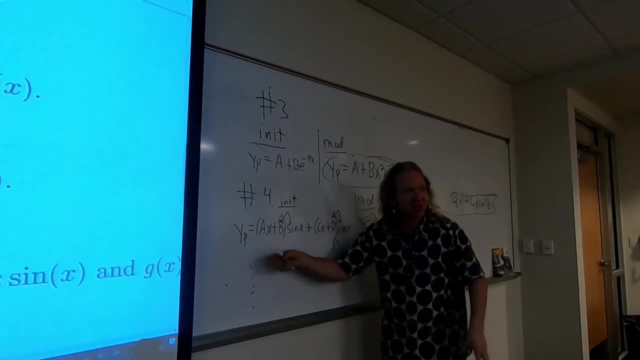 You won't get the answer You need to. Is it because they? No, it's because so this is one thought. that's a hard question. This is one thought process. So, because there's repetition here and this came from one thought process, you 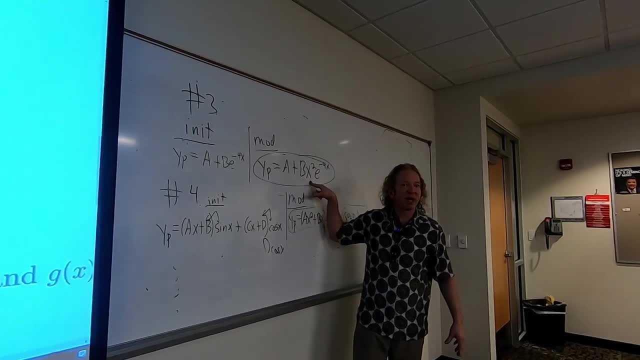 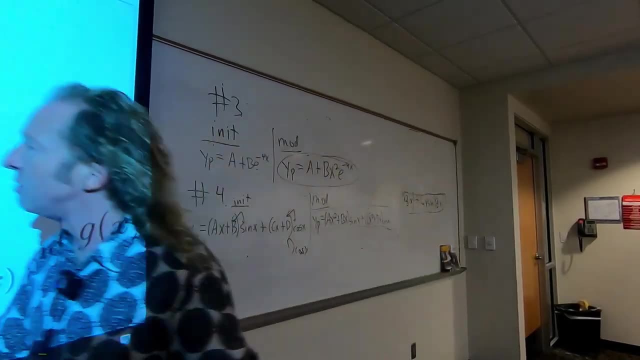 have to multiply the whole thing by x. Notice, here we only multiplied this by x Because this was one thought process. This came from the nine. They're separated. They're separated by a plus. Let's keep going. and you know, let's see, Let's do. 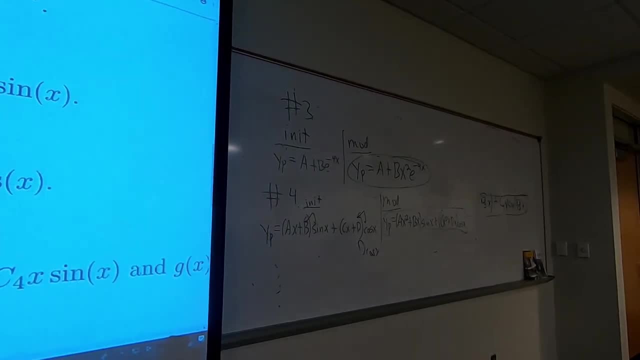 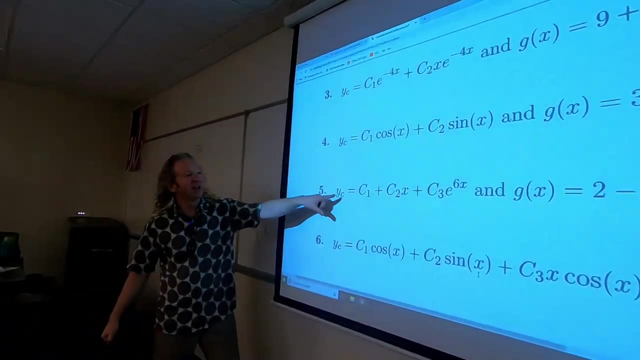 number five. Maybe it'll make more sense If you multiply them and lay them out. they wouldn't be in the same process, but they'd separate. Right, then you're separated, Yeah, So let's do five. Five, This one. So, looking here at 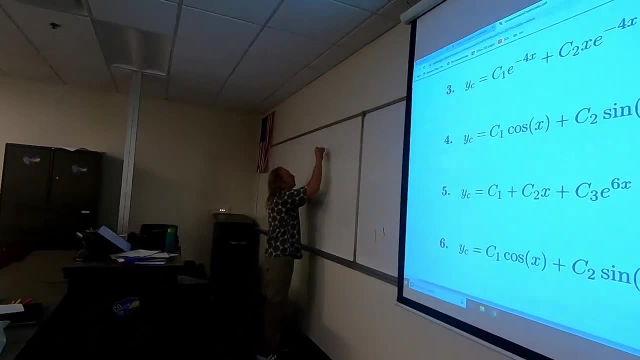 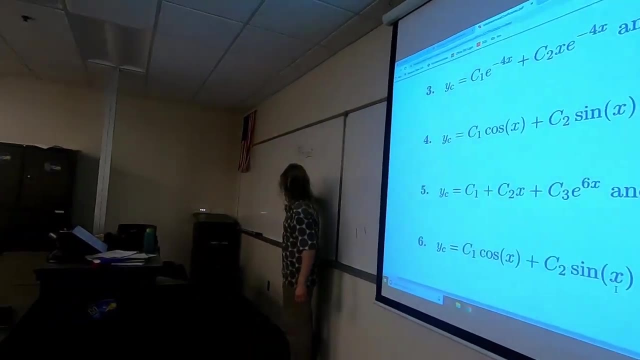 this one. so we have initial Initial. So the initial for this one, the two. what is the two going to give us A? A Good. The two's going to give us A right. Everyone see why that two gives us A, Because 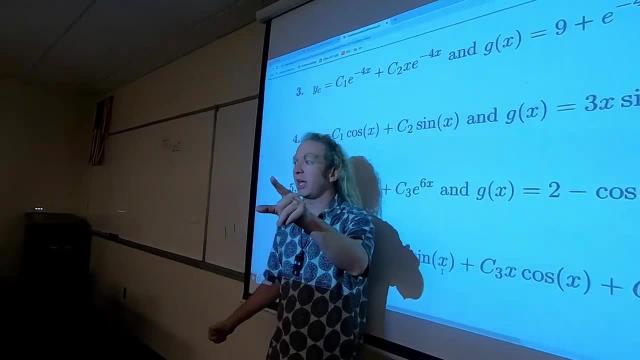 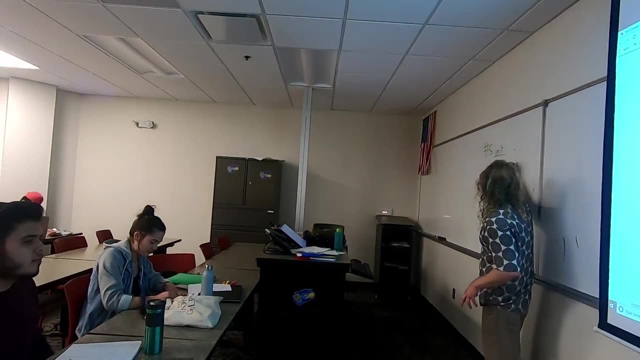 it's a constant. So what's the cosine going to give us? The cosine and what? And A, A And the sine, So both Yeah. So plus B, cosine x, plus C sine x. The sine doesn't matter, The sine doesn't matter. If you put a minus sign there, I'll want to mark it wrong. but 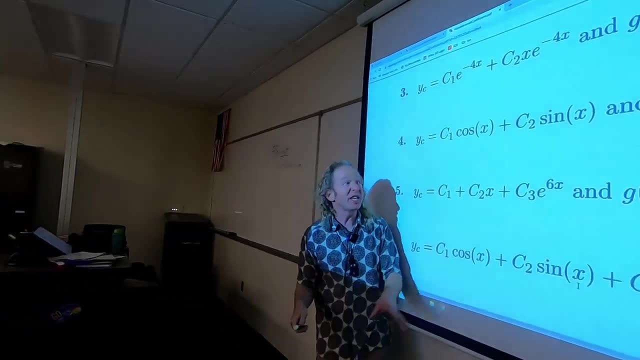 I can't because it's not wrong. But you don't need it because it gets absorbed, So the minus doesn't matter. It could be like a five there, right, And it wouldn't matter. Everyone okay with the init, with the initial part. 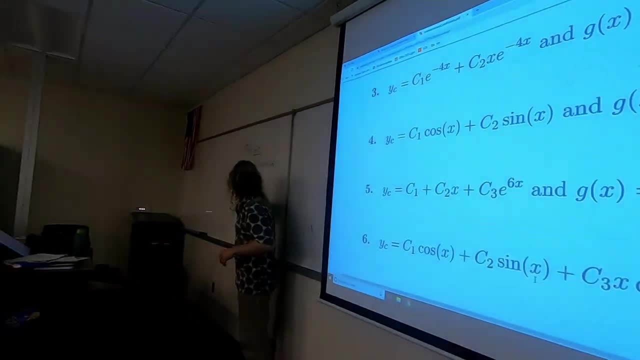 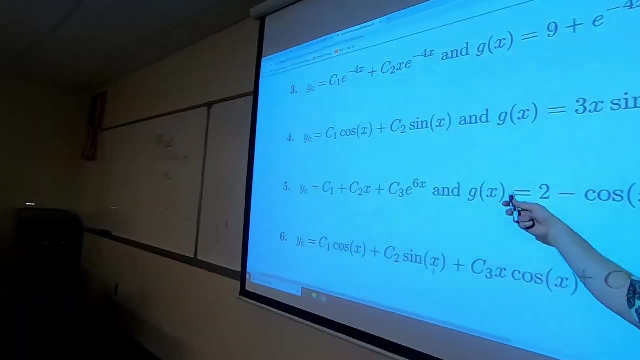 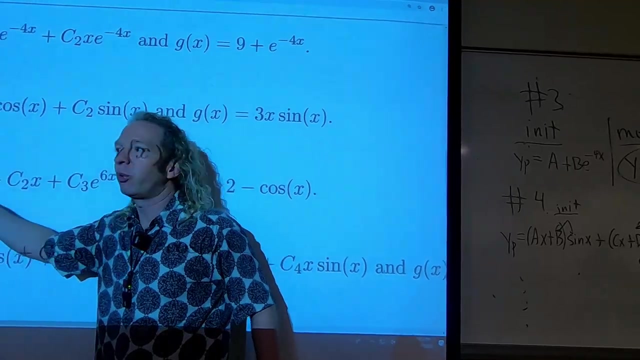 Modified. Okay, the modified, then. So mod, So mod. So for the mod, you look at the two, You look at the two. So the question is, does this two repeat with any of these terms, With which one? C1.. 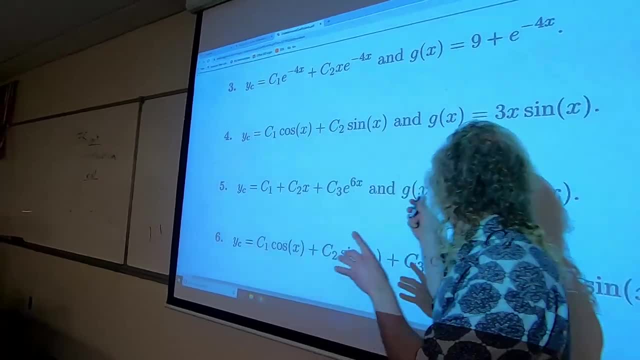 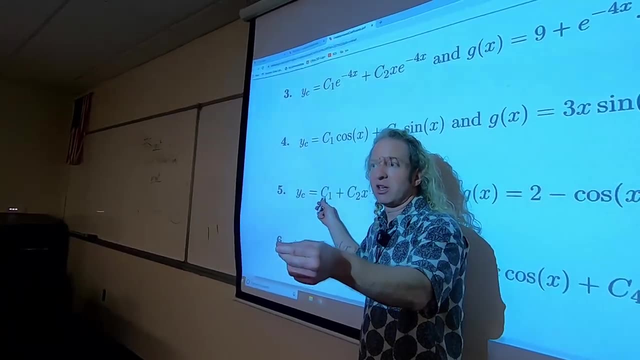 The C1.. Do you see why? Urosh, Okay, Urosh two is a number, right, It's constant. C1 is a number, But is it not a constant? It's constant, So they're the same. They're both constant terms, So they repeat That's. 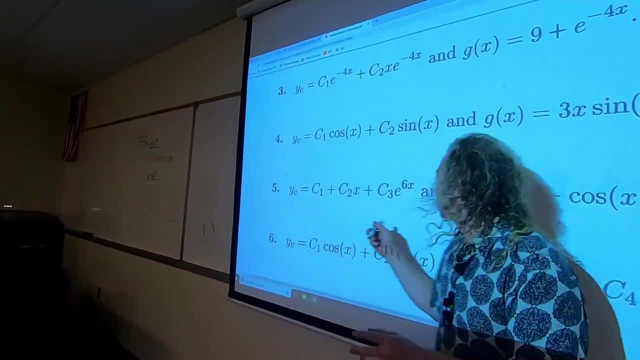 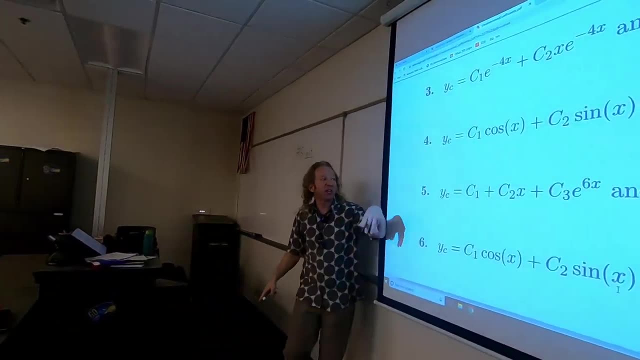 what I mean by repeat, Do you see now? Yeah, So, because they're both constants, So it repeats. So that means you have to put a what on the A, An X, An X, But then you have an AX. 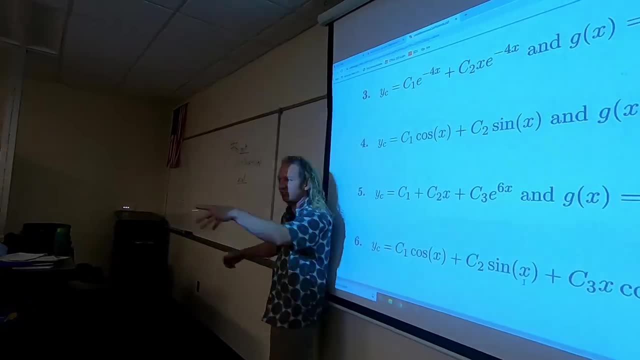 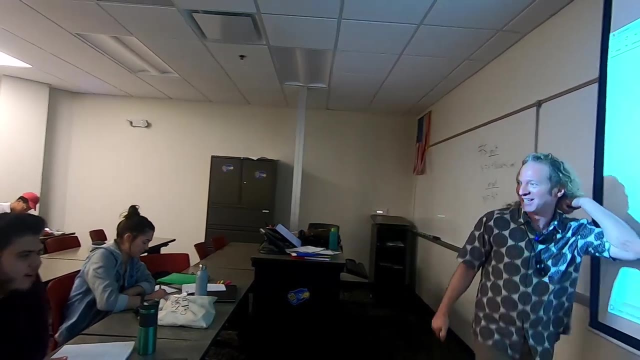 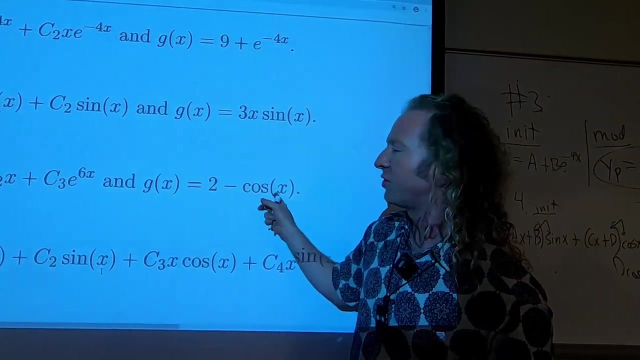 AX, AX, because it still repeats, right, You see it now. Oh, it's better than nothing. Okay, so YP equals AX squared. So because two and C are constants, So that's why it repeats. And then, oh, what about the cosine term? There are. 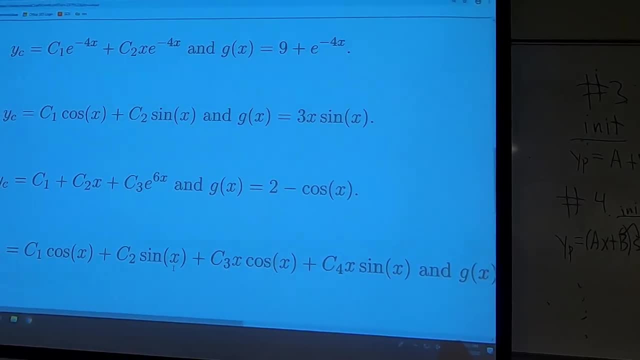 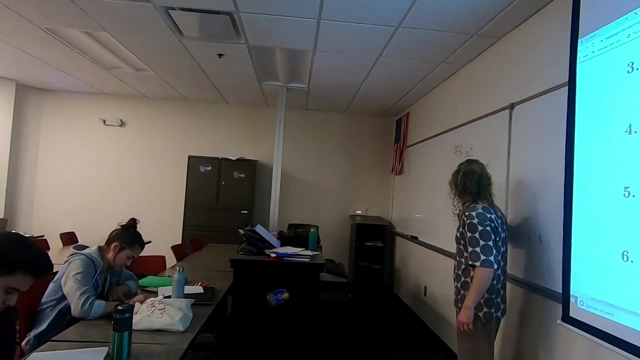 cosine terms. None of those- repeat, None of these- are over here, So we're okay. So, plus B cosine X, plus C sine X. So that's the answer. Let's do the next one. I'm going to pull it up. Oh, the next one's easier though, But 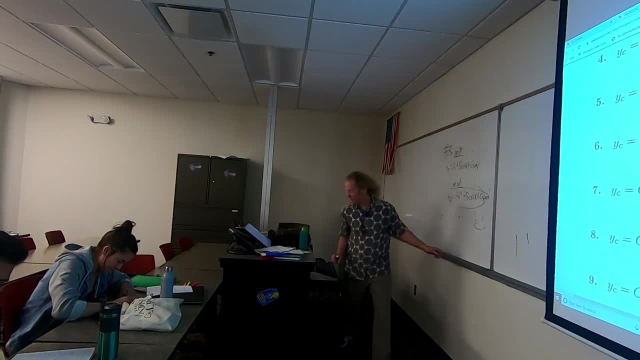 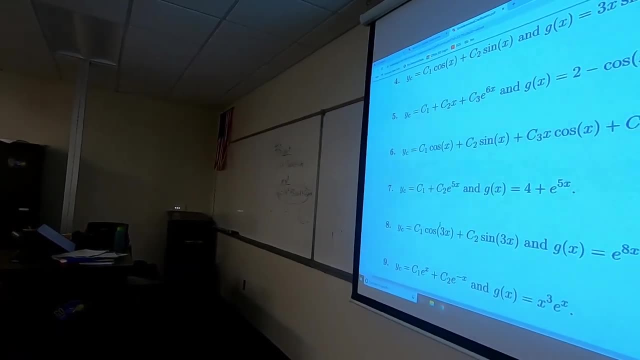 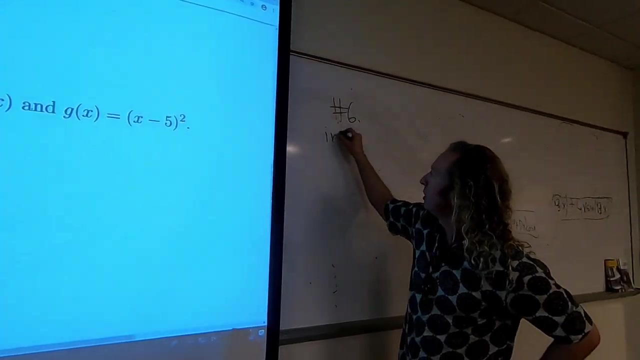 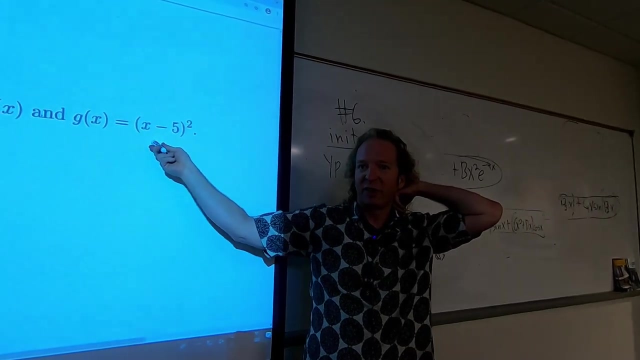 let's do it anyways. It's easy: Six, Six, Number six, Six, All right, number six, All right. So, looking at the right-hand side, we're only looking at G. So if you look only at the right-hand side, if you multiply this out, you get X squared minus 10X plus 25.. 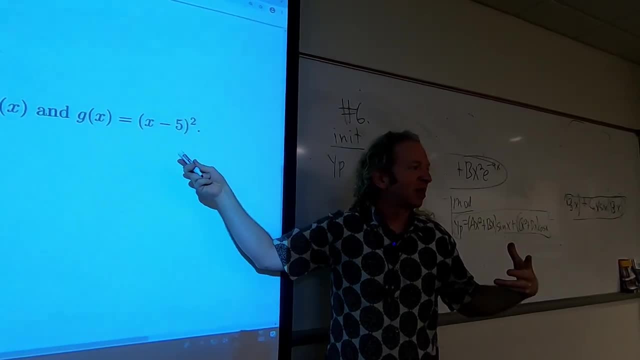 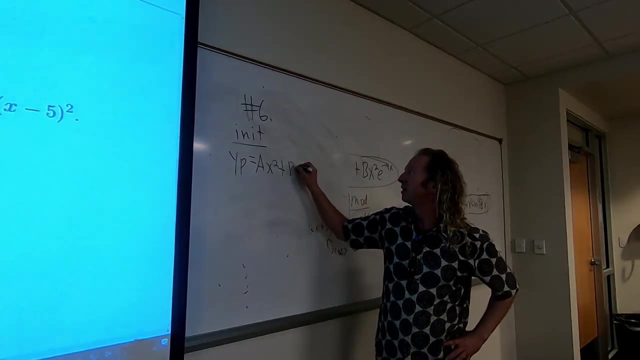 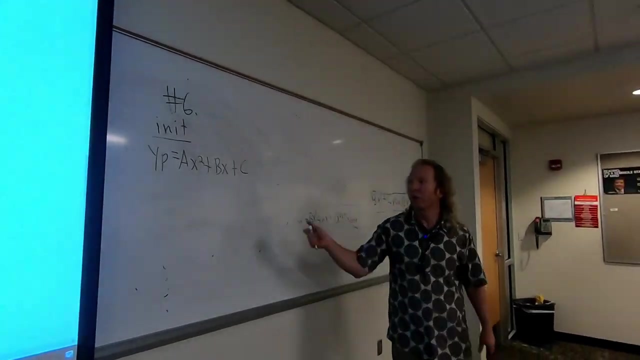 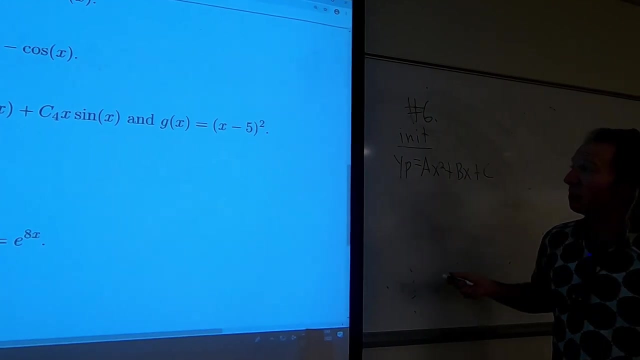 Right, So you get a quadratic. So the initial guess is just a quadratic. So it would be AX squared plus BX plus C. Everyone okay with. why it's that? So, because if you multiply it out, you get X squared minus 10X plus 25.. So it's a full quadratic. All right, is there repetition? No, This is. 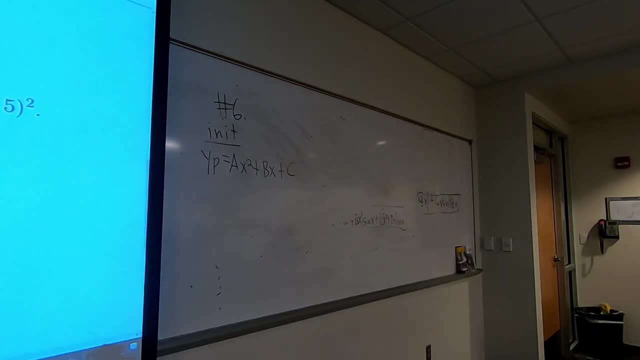 an X sine X. These are all trig-phjas. Isn't x sine x? These are all trig functions. There's no x here. There's no x squared here, So that's it. I'm not even going to write the mod. 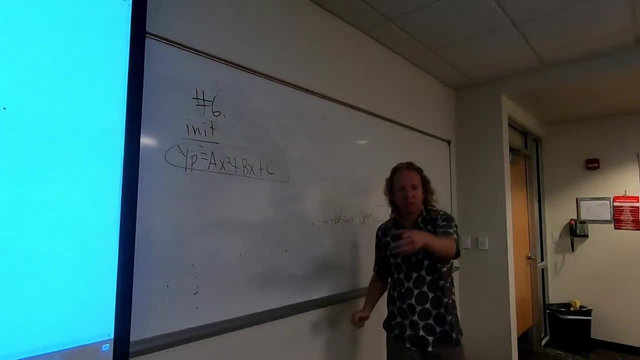 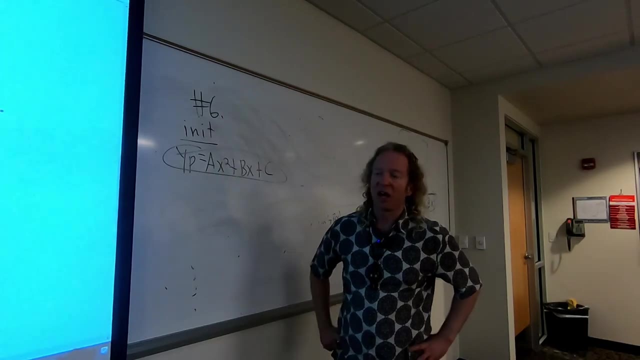 That's the answer. There's no mod. It's the same. So if you have an x squared, you're building more than whatever single x that comes after that. Uh-huh, Even if this was just x squared, you would still have the same thing here. 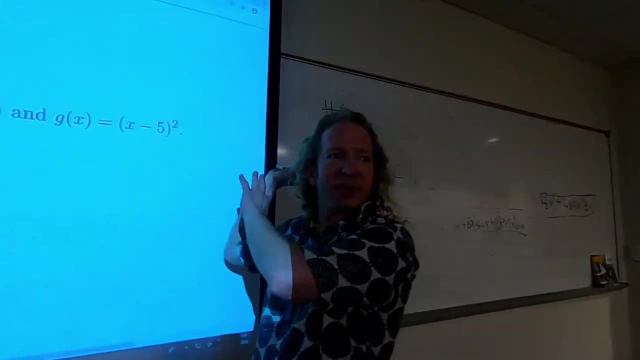 If it's x squared plus 5, same answer. If it's x squared minus 20,000, same answer. It's a quadratic. Yeah, 7 is a really good example. If you understand 7, then you've got this. 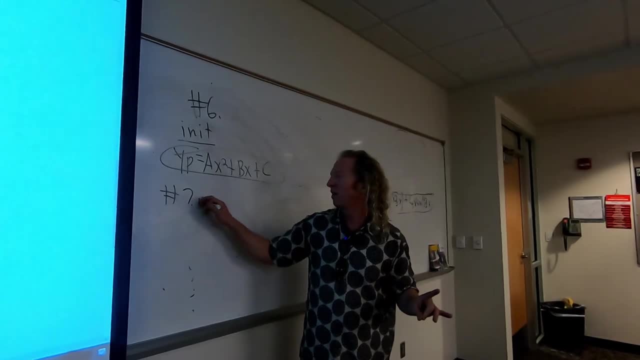 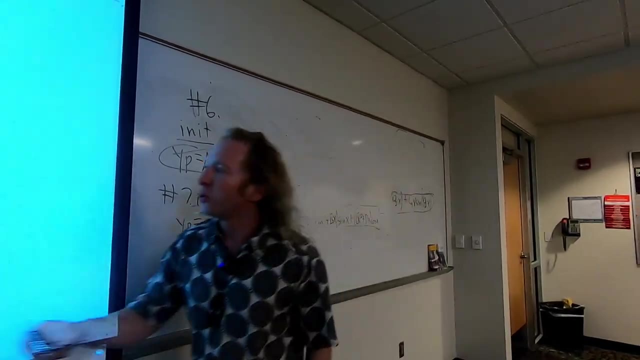 7 is really, really good, Because it could be better, but it's good. So the init, So the init. it's going to be two separate yeses, right? So first we have to make a guess for the 4.. 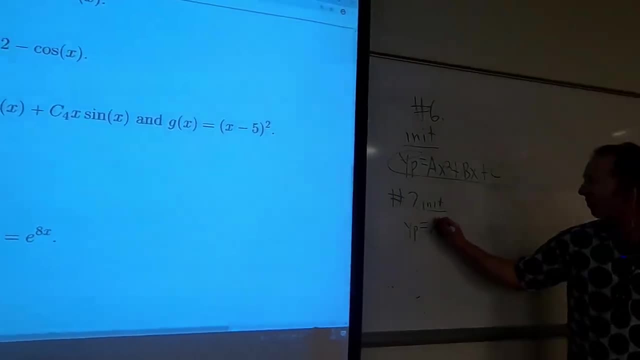 So what would the guess for the 4 be? A, Yeah, just A, right. And then for the e, we just have to put a b in front of it, right? So b? e to the 5x. So that's our init. 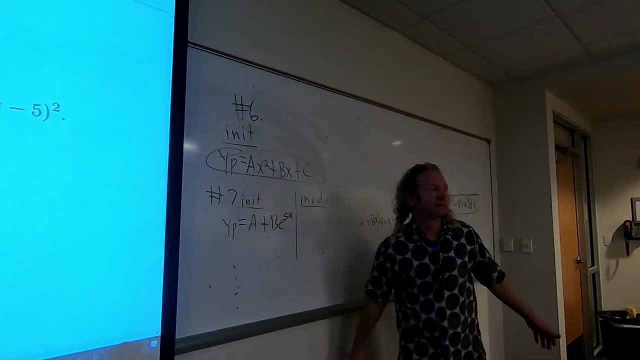 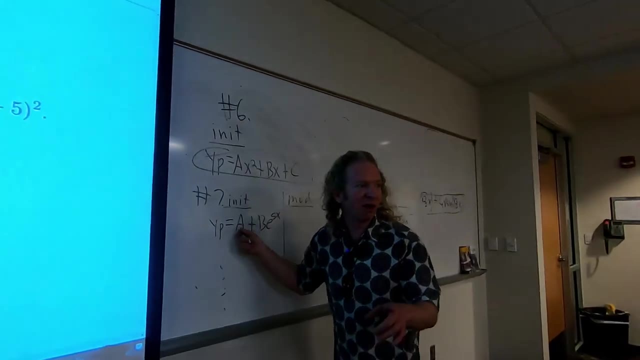 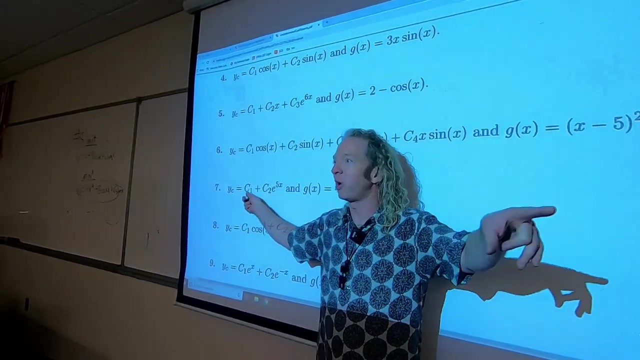 Pause here for a minute, Mod. Okay, so now we have to look at the a and our yc. So does a repeat with any of these terms? With which one? With the c1, because they're both? what terms? They're both numbers, right? 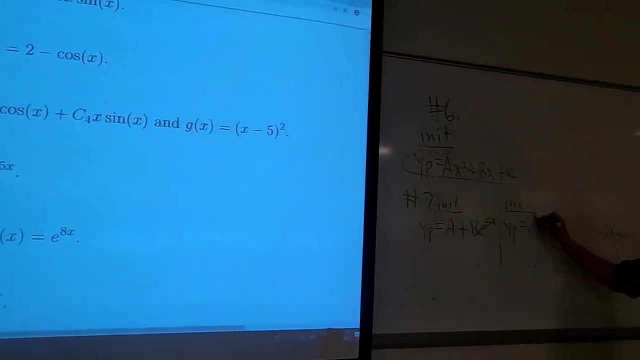 So you have to put an x in front of it. It's not x squared. No, it's not x squared, though Right, it's only 1.. Okay, so now we have to look at our e to the 5x. 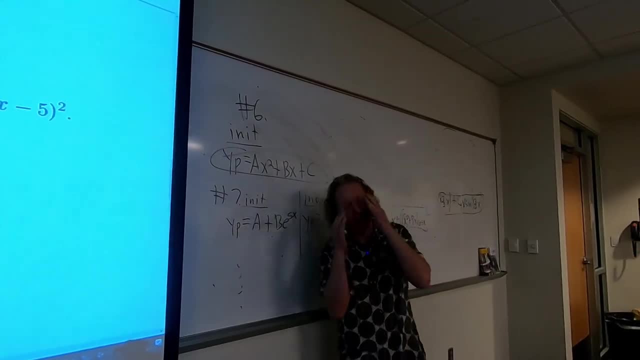 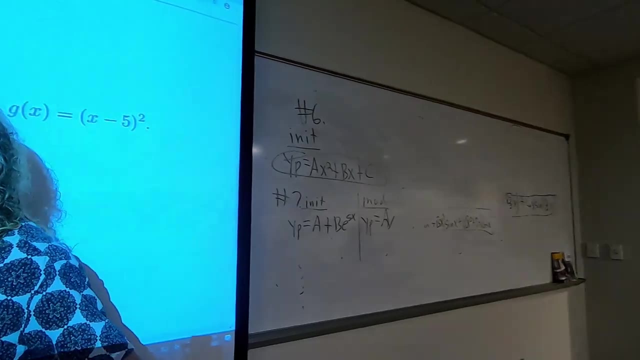 Do you have to leave Momodou? Really? No, Okay, it's all right. it's all right, That's okay. You get it Okay. b e to the 5x. So does b? e to the 5x. repeat with these. 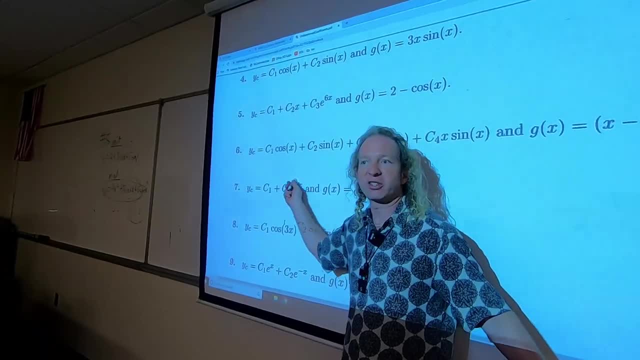 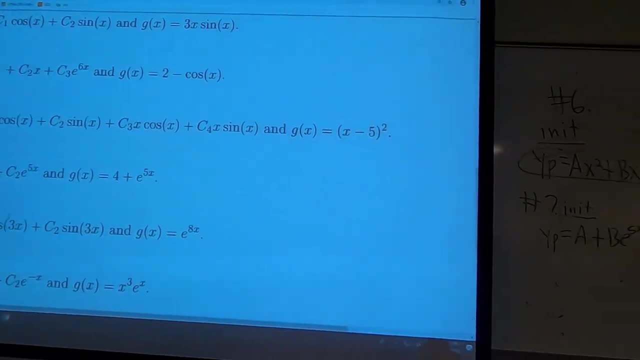 Yes, with this one right, Because they're both e to the 5x terms, right, They both have an e to the 5x, So what do you have to put in front of it? An x, Very good, an x. 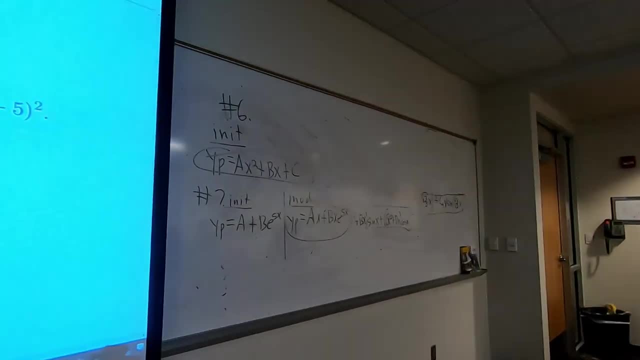 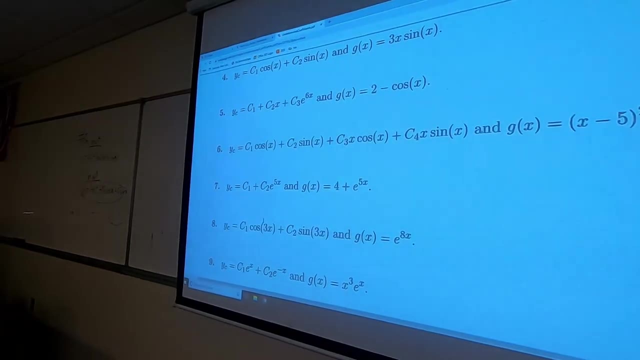 An x. Does it make sense now, Udash, Huh, Why you don't get it? What don't you get Udash in 15 minutes? Tell me. no, what is it? what is it Like? I get the a part and 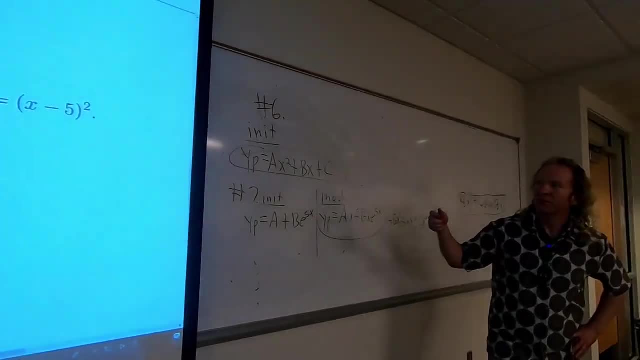 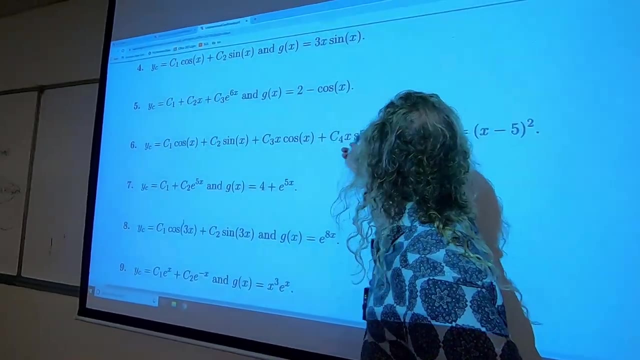 Is it this Like in the last? I think it was the c1 cosine. Yeah, this one. So what happens with those x's? No, no, no, number 6.. Do you see those? how it has c4x and c3?. 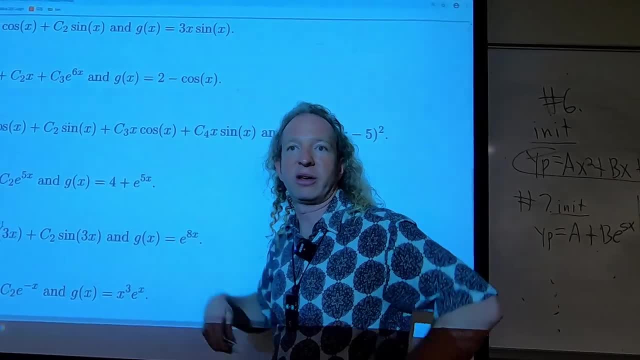 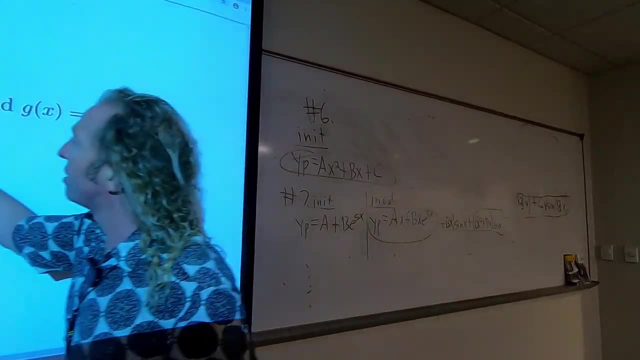 You don't even. you didn't use it Because there's no x squared. Because there's no x squared, So we got this from this, Yeah, And then this: These are x's and x squared's. There's none here. 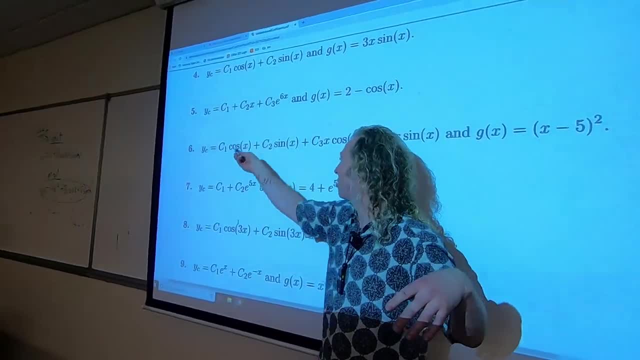 So you just look for the first term and then You look for all of them. There's no x's. Where's the x? That's an x, cosine x. That's not an x. It's got to be an x by itself. 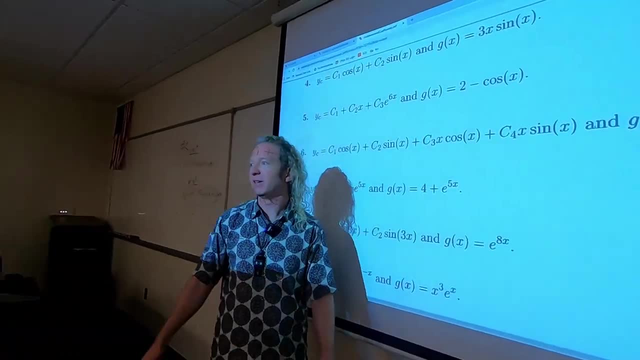 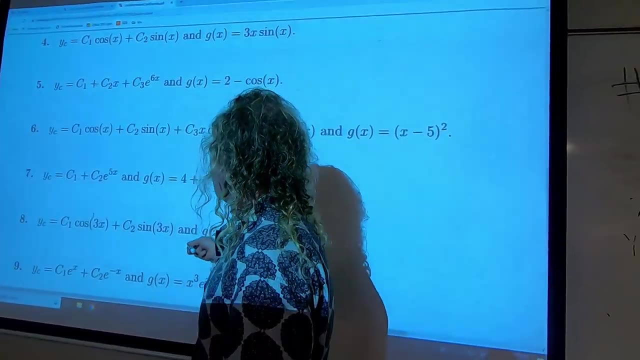 Or an x squared by itself. Right, You see it. Oh, that's it, That's better. See, now you see it. Let's keep going, Number 8. Let's do this 8. Weak, Uh-huh. 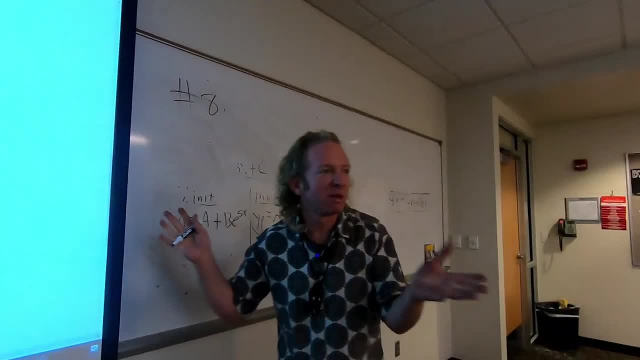 You don't have to do any like sine cosine Because that isn't on the right side. That's not on the right side. That's not on the right side. Yeah, you got to. It's really. You have to really look at the right one. 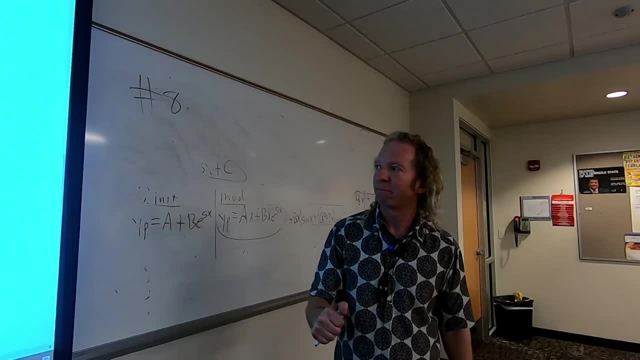 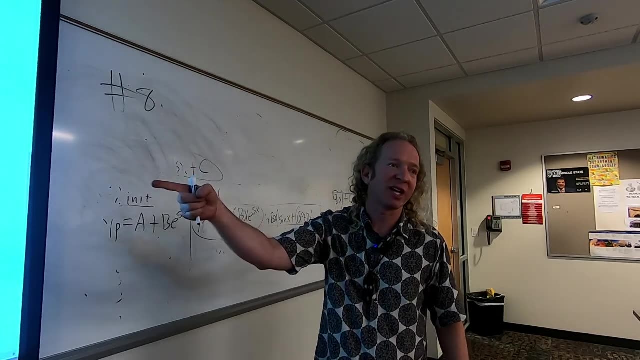 Yeah, good, Let's keep going. Yeah, So when you have the ax squared, bx Plus c, Does it have to look like that? It has to look like that, But it won't. It'll never look like that actually. 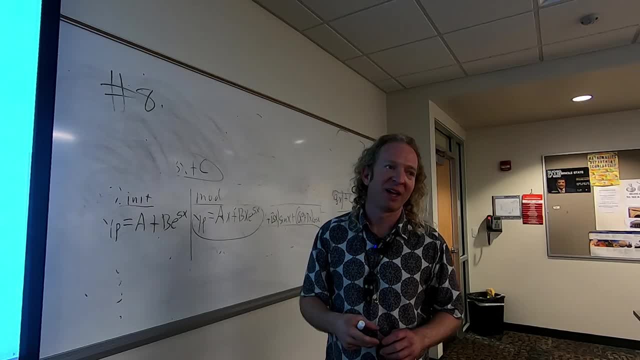 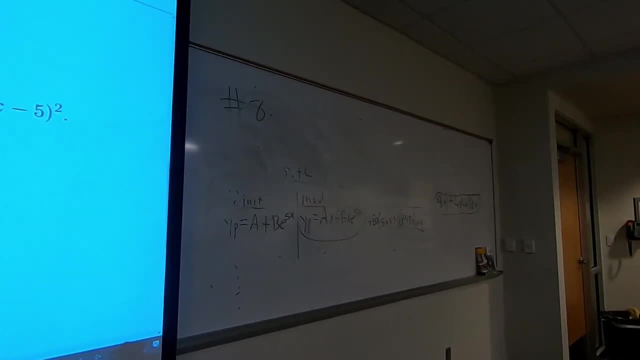 It will never, ever. It can't just be like an ax squared and you go. That repeats, It has to be the whole thing. It'll never show up here Because it'll never be the solution to one of our questions. You're always going to have e's sines and cosines here. 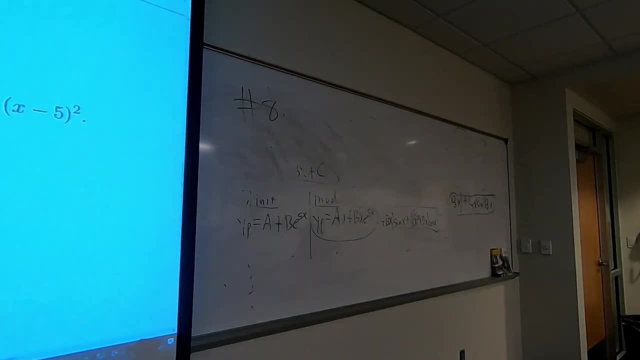 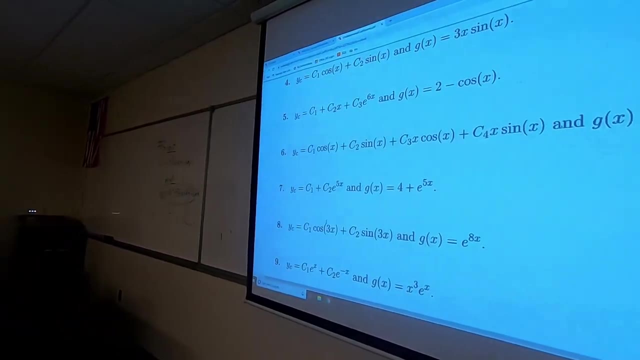 You're never going to have x's here anyway. so, Oh yeah, you might. You might have cx squared. That's not true, I messed up. Yeah, you could. Yeah, it would have to. If it's just c1x squared, does that mean? 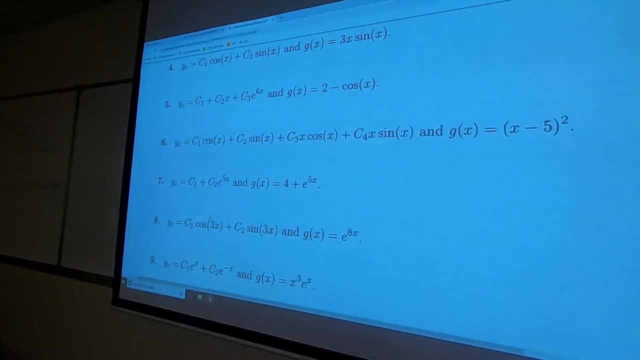 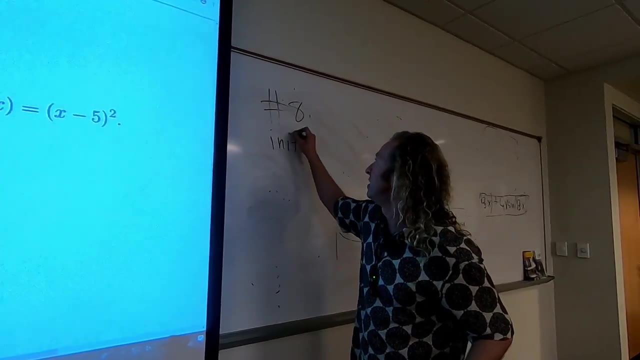 You'll never have just c1x squared. You'd have to have c1 plus c2x plus. Yeah, it's impossible to have that, So 8. 8. So in it, 8's really easy. 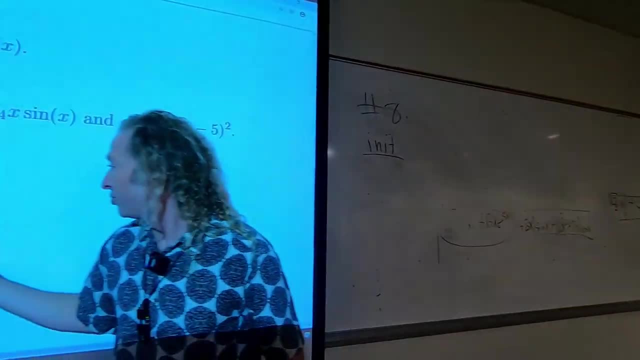 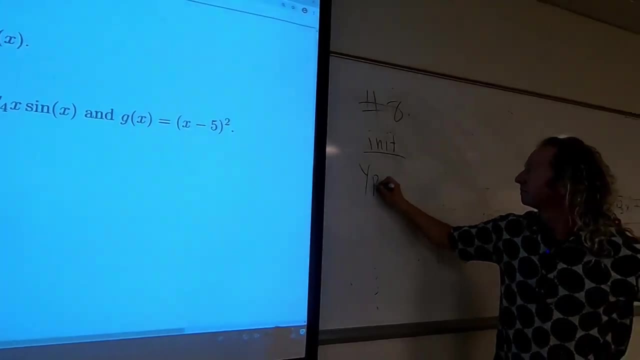 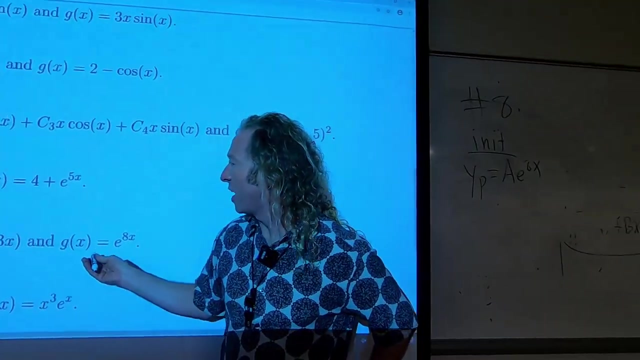 So, but easy is good. So on 8.. So you look here to make the initial guess. So it'd be ae to the 8x. And then are there any ae? Is there any repetition? No, because these are sines and cosines. 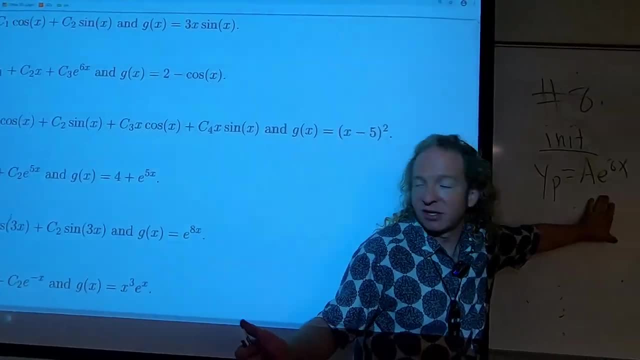 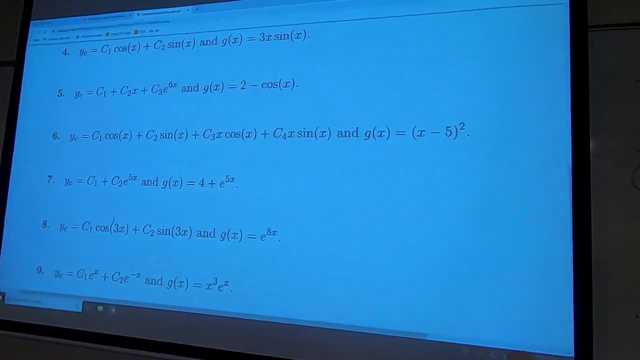 So here's the thing: You look here and you compare this to these And they don't match. so that's it: 9. 9. 9's better. 9's a much better example. Let's do 9.. 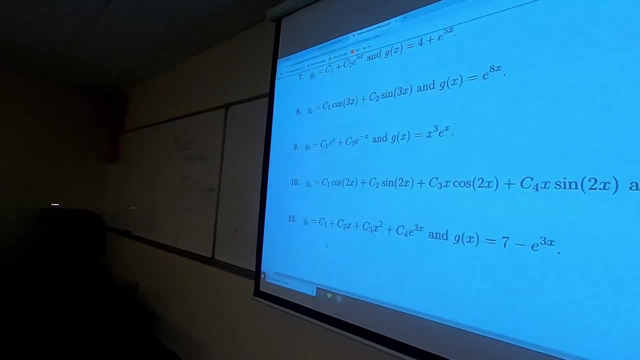 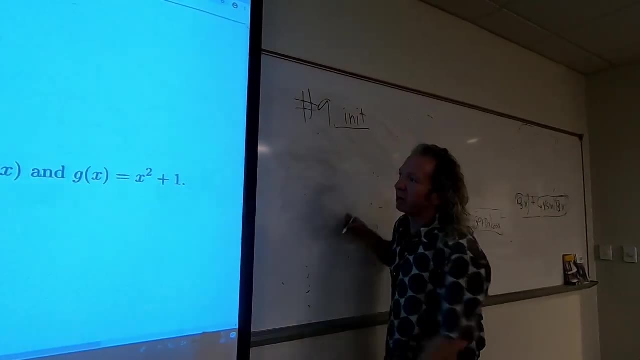 I'm going to write it here: 9. 9. 9. 9 is hard, So So in it, So the in it for 9.. So we have a cubic in front of the e, So we have to have a full. what? 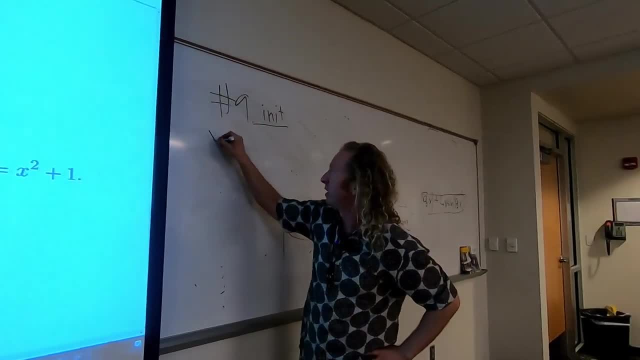 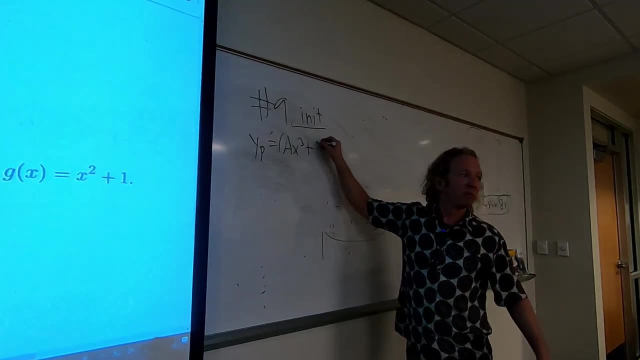 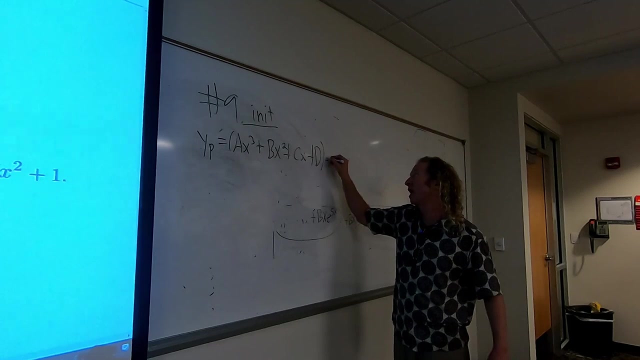 A full Cubic. A full cubic, So it'd be: Yeah, full cubic. So it'd be: ax cubed plus bx squared, plus cx plus d. This is a hard topic. This is a hard topic, So that's our initial. 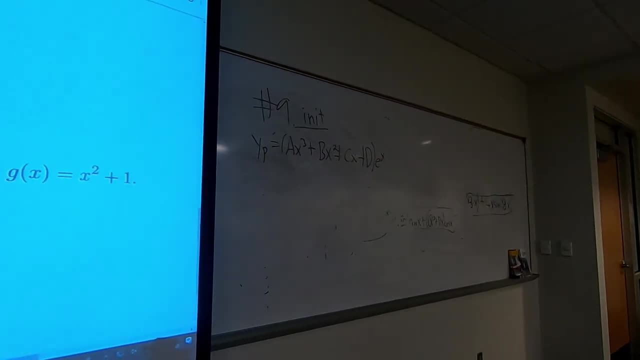 Okay, I'll let you write it down. Take your time. We got time. We still have 13 minutes. We'll be able to do a de. I'm just going to do a really easy one, So is there any abdx? 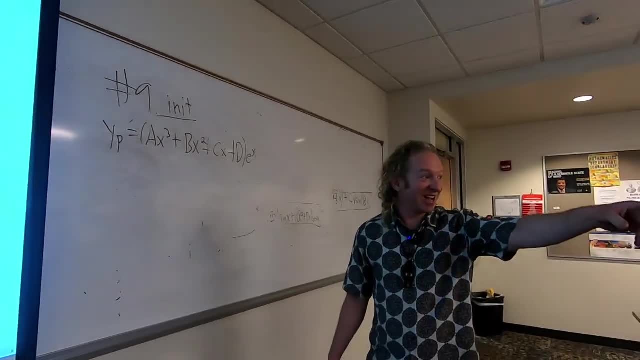 Yes, You're right, Urash. So there is repetition Because, look, It's like what Sadani was saying. Think about de to the x, It repeats with With this one. You see, It repeats with this one. 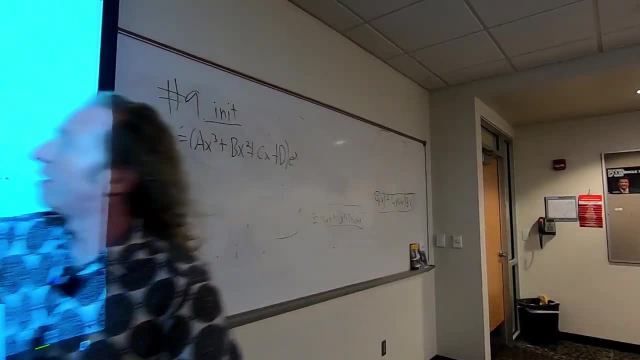 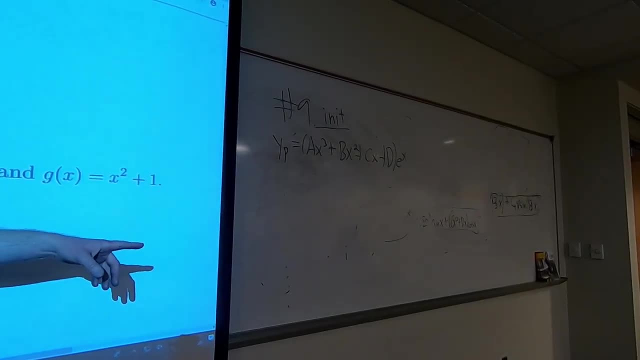 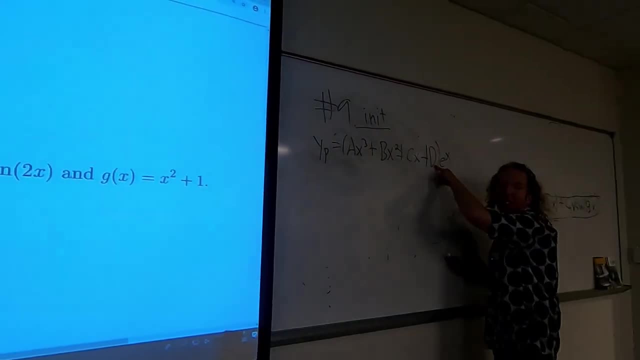 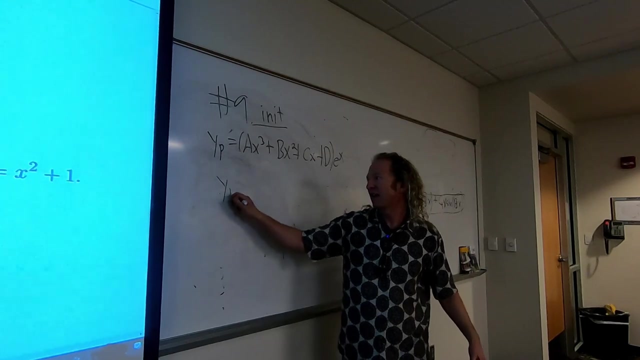 So a really good question. Rafael was saying: can you just put an x here? You can't. This came from one thought process, So you have to put an x on the whole thing. Okay, I think that's the trickiest part. 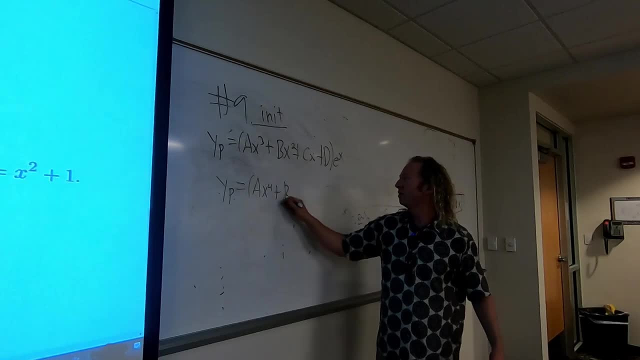 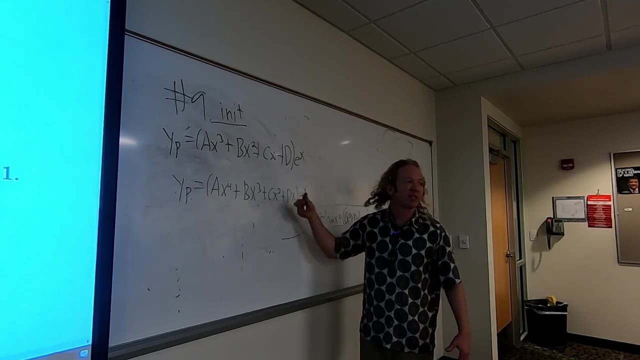 After you like master everything, you get stuck with that. I'm distributing it because that's what I usually do And because typically that's what you would want to do. If you were solving a de, That's what you would want to do. 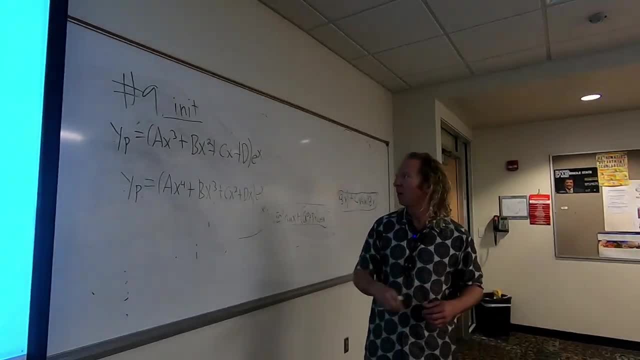 Yes, Ian, Can you just put the x on the Onto the ex, Onto the de, No onto the ex. Yeah, you could Like over here. Yeah, just to distribute it. Yeah, you can. 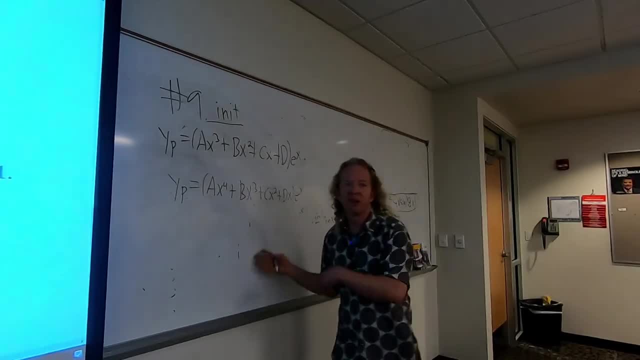 You don't have to distribute it. I just figured I would, because when you solve the de's, that's better. You have to take the derivative of this stuff later Like it's crazy, But it's messy, It's not. 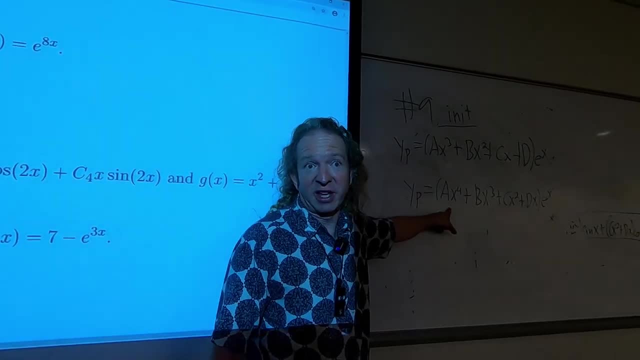 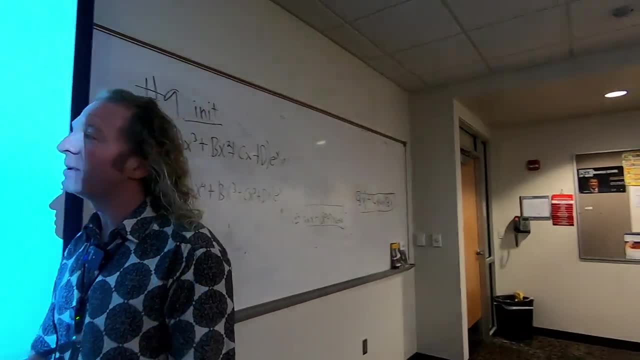 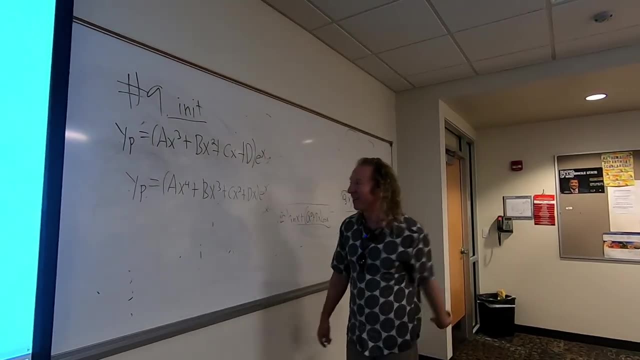 It's not. Messy is pretty tricky. you know what I'm saying. Messy can be, But you know This thing is called partial credit, Right? So This is like you know. It's almost hit or miss. 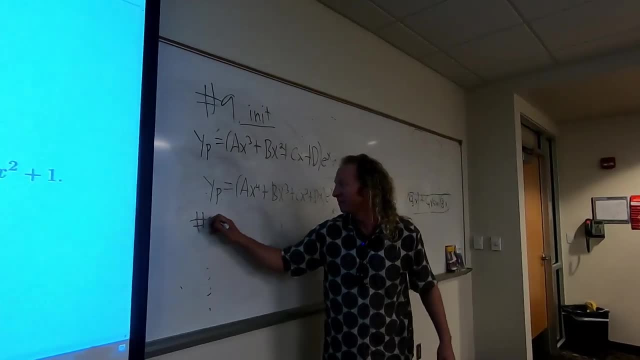 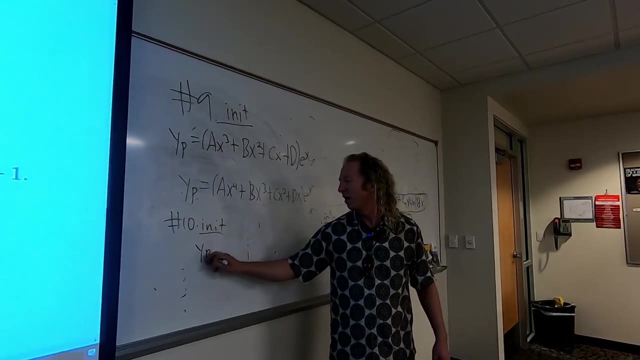 All right, Everyone okay with this one. Ten, So for ten. Ten's really easy. What's the, What's the init for ten N squared E s, C Plus C. Right, So full credit Right. 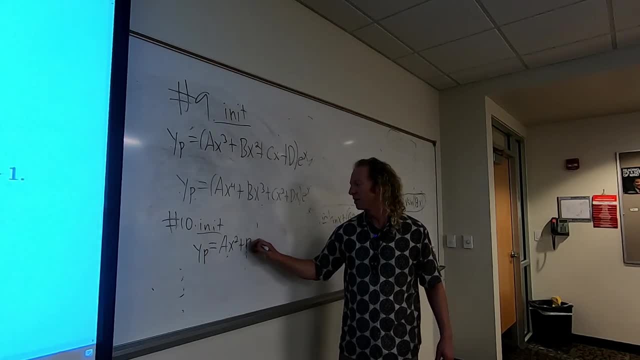 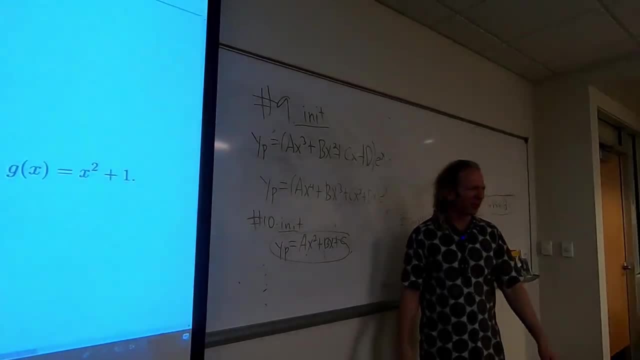 It comes from here, Full quadratic. That's it, And that's it. Oh, Matthew, you didn't get a hundred Because there's no repetition, Right, There's just all sines and cosines You are. One time there was this guy. 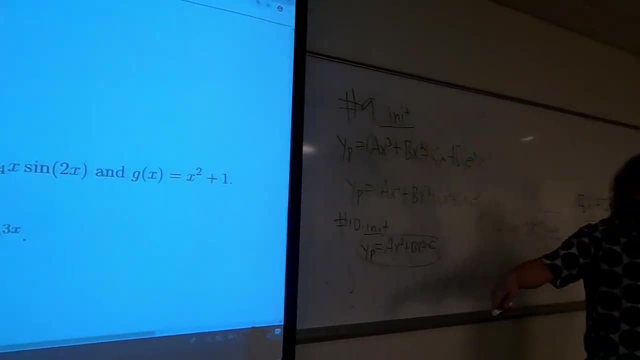 It's a really bad story. And he was in my office And he did all of these before the test. Every single one. He's like I get nervous during the test. I just freeze. Then he took the test and he got them all wrong. 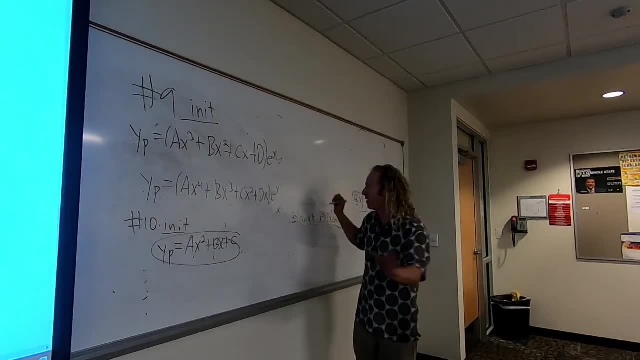 Almost all of them, I know I felt really bad for him. He's done now, He has a job, He has a degree- Like life goes on. I just remember him, though, And every time he was in my office since then we joke about it. 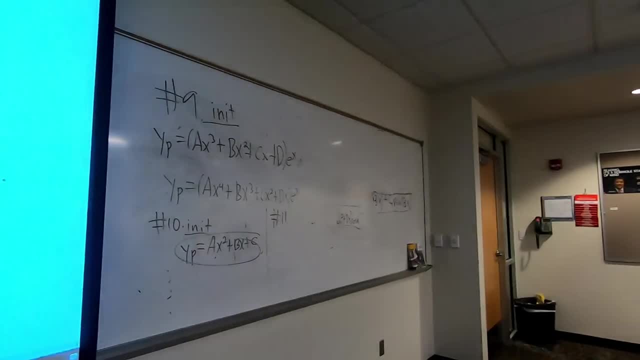 Like, remember that test And I'm like, And I watched him- He was sitting like right here during the test And he was just like I'm like, oh my God, He really is freezing up, Like 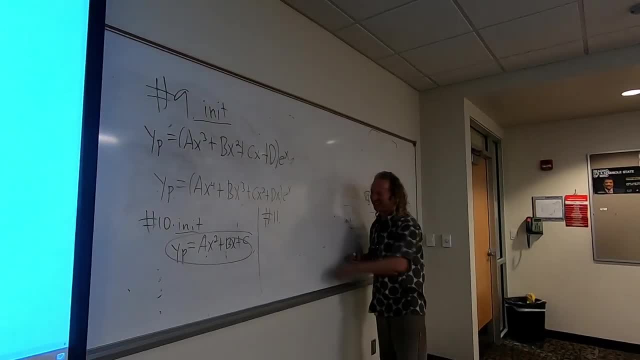 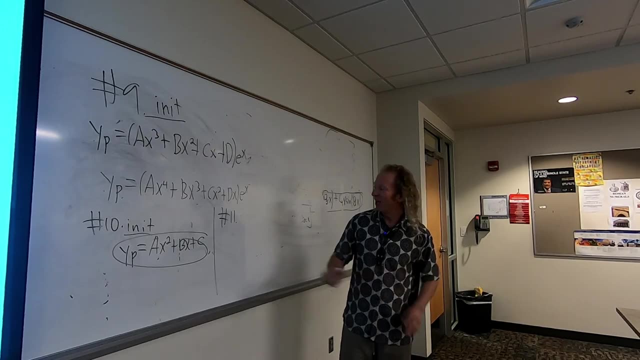 He made it. He got a degree, He has a job, He's a high school teacher now. Okay, Yeah, He's, He made it. He made it In it, In it. So the seven In it. 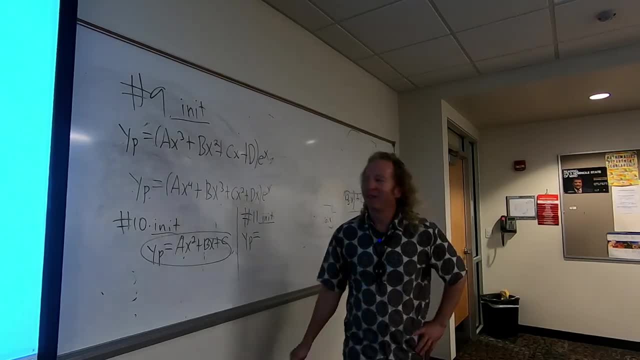 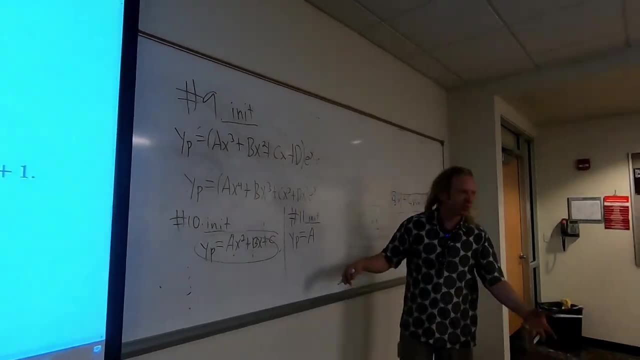 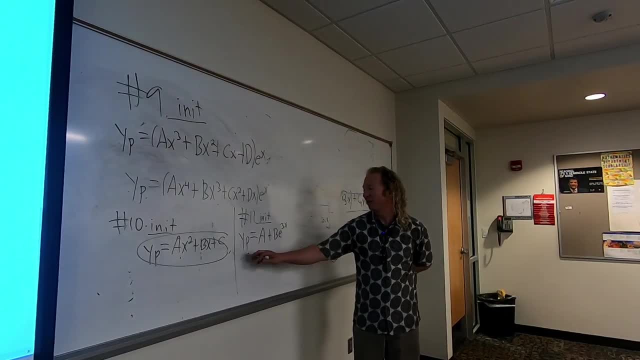 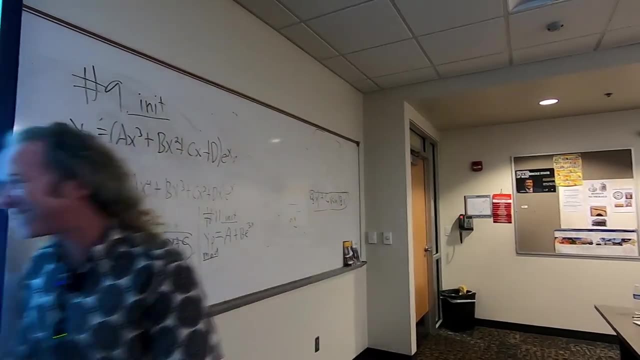 This one, this one, This one's the ultimate question. Save the best for last. Would it be AX cubed? Oh, yes, it would be AX cubed Right, because if you put AX, ooh, too bad. 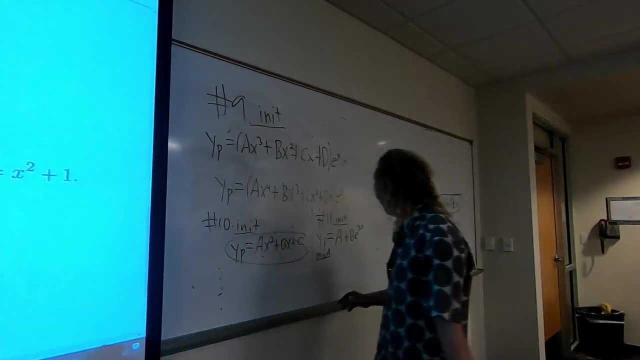 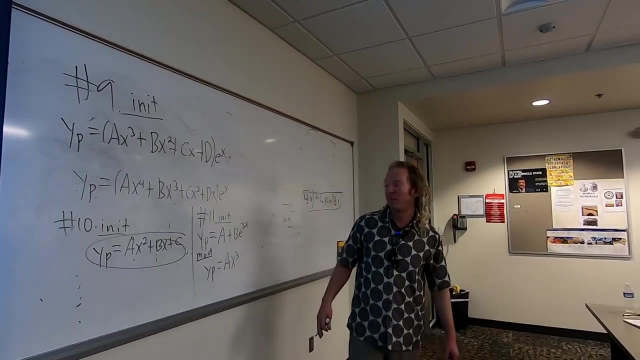 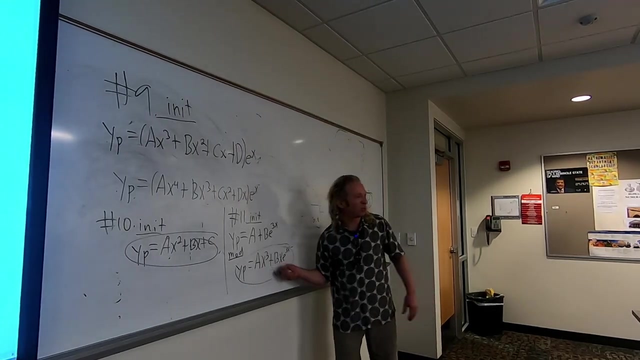 AX squared. ooh, too bad. You got to do AX cubed. Yeah, Yeah, Absolutely So, AX cubed. And what is it? BX? yeah, BX. See, I like this one because it's a different number of Xs for each one, right. 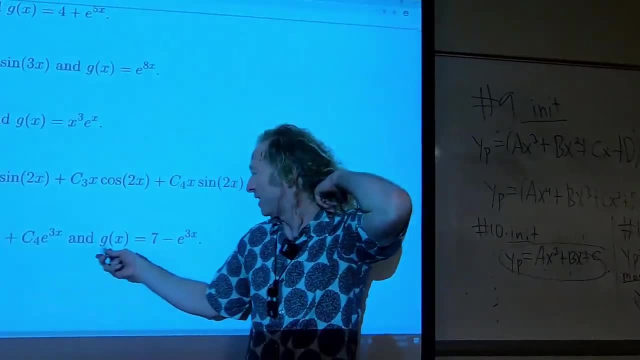 You got to have an AX cubed because of this and then you have to have- I guess you get it now. Udash, Oh, oh, so proud. No, no, you got it, I just want to like: oh, let's go, let's go. 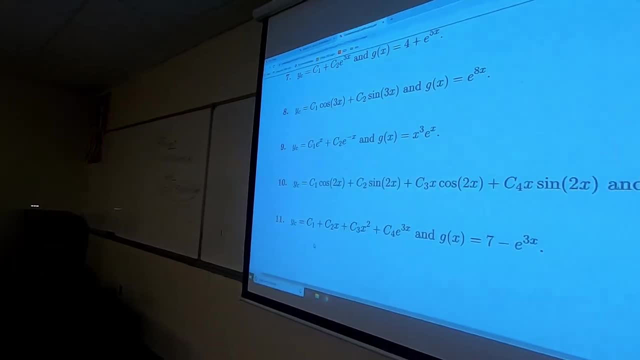 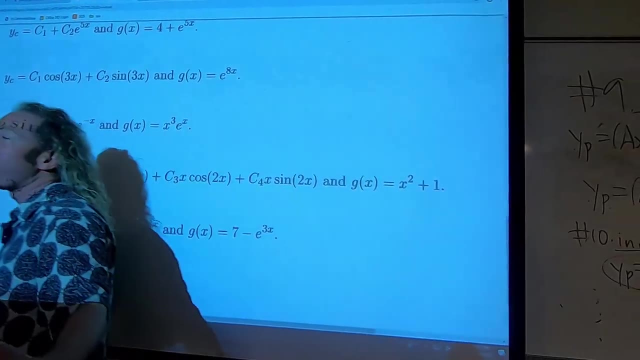 So if you have Xs, basically you can add it to the constant. If you have A, Yeah, I think yes to what you're saying. Okay, All right, we have nine minutes. I think it's time we do a DE. 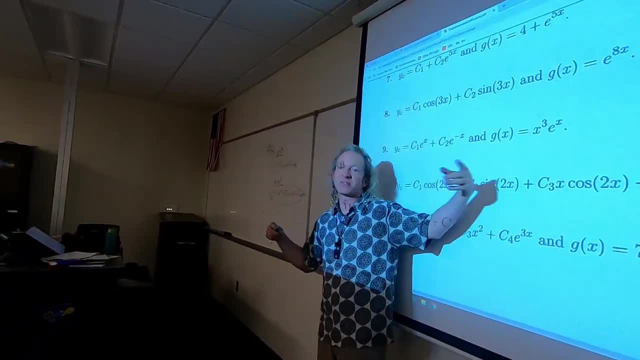 Any last questions? We're going to do this again next time. You know why? Because we'll have some review time and I bet you'll want to review this right. Usually it's like: all right, we have 30 minutes to review. 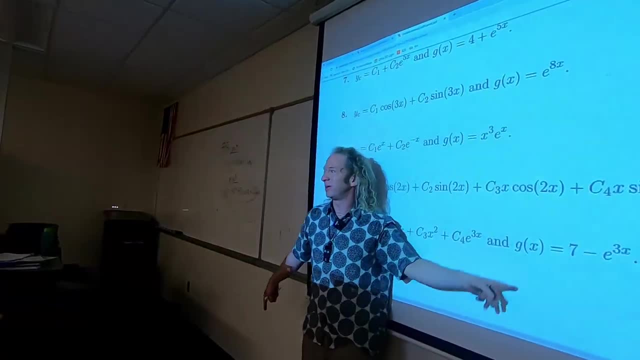 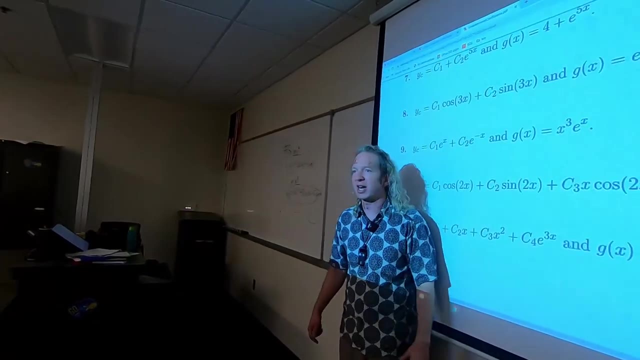 What do you want to review? And it's like 40 points, right? Yeah, I know, I know we will review it. We will review this next time. Any other questions on this one, You think you got it All right. let's do a DE. 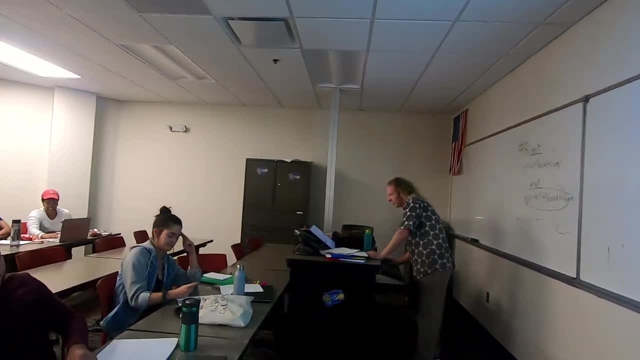 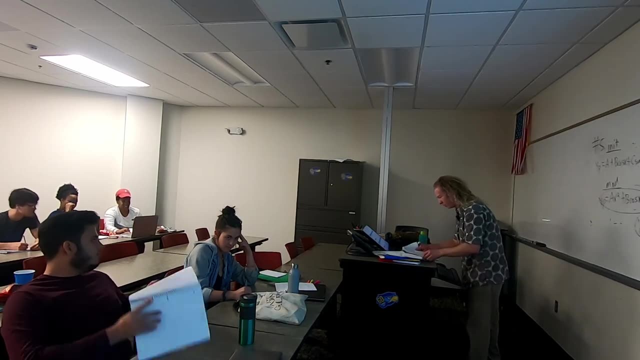 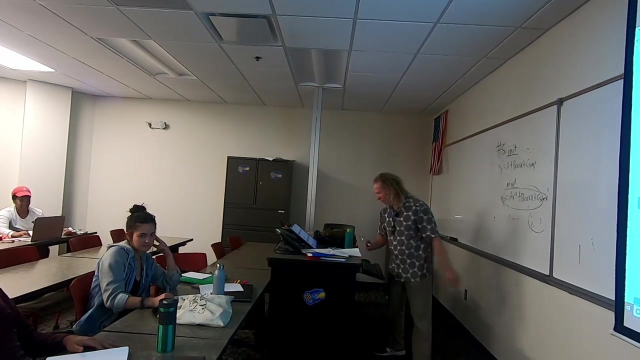 Let's do a DE, Let's do, Let's do, I think, number. I wonder how hard number two is Yuck. How about number three? Yeah, let's just do one. One's really easy. We still haven't done step three. 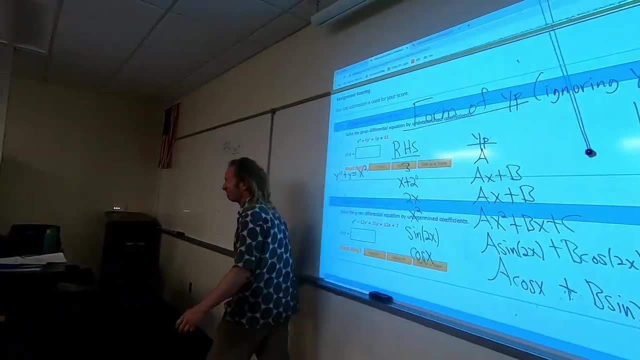 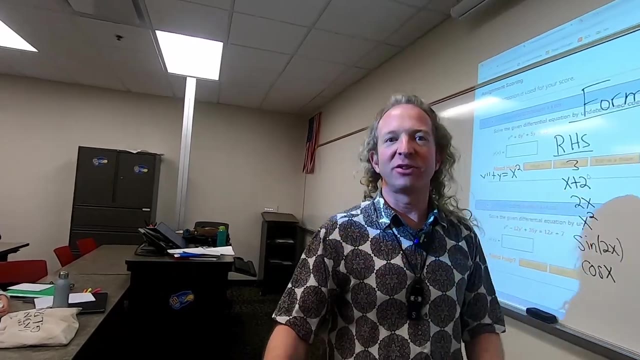 Yeah, let's do number one then. That's all the steps, All of them. Was this step three? No, that was step. This is step two and three combined. This is step two. This is just step two, So step three. 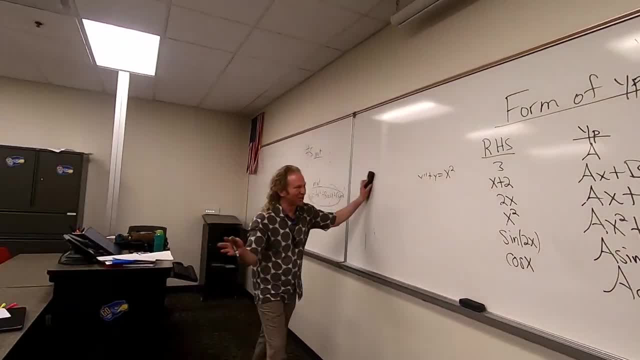 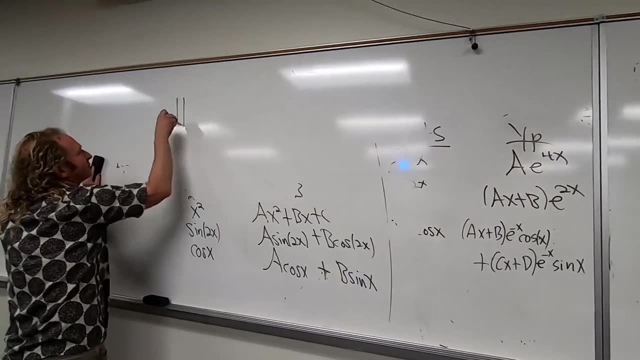 I'm figuring out what I'm going to do. What am I doing? So let's do number one. How much time do we have? Yeah, number one. Yeah, step three was the repetition, right? Yeah, those steps. Yes, that was step three. 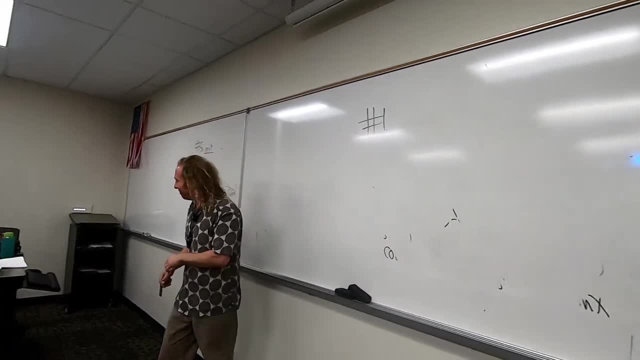 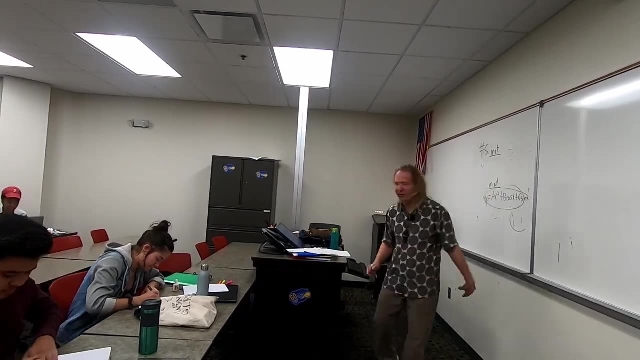 Yeah, that was I was thinking of, like the questions on the test. Oh, no, no, no, no, no, no, It's just the steps. Got it Okay, Okay, Yeah, Okay, All right, let's just do number one. 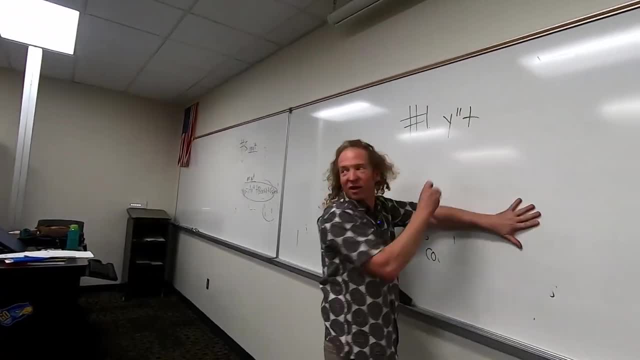 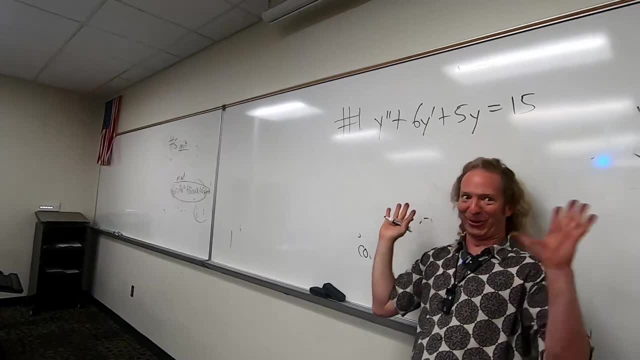 Equal to 15.. Equal to: Oh, it's a number. Oh, it's like it's not zero, Like, oh, it's game over, right? Do you have to leave? I gave up Really, Oh no. 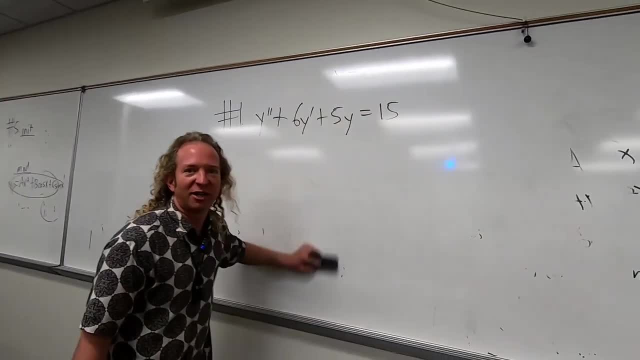 Okay, Okay, okay, There's a video of this already in the playlist too. Okay, all right, All right, so I'm going to write the steps like they are on the test. I think it's better, Because in the homework it's just a solve. 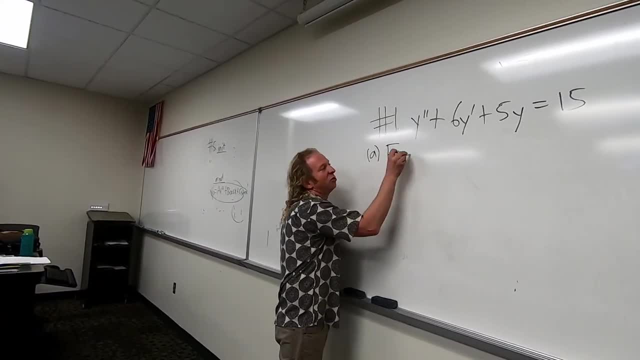 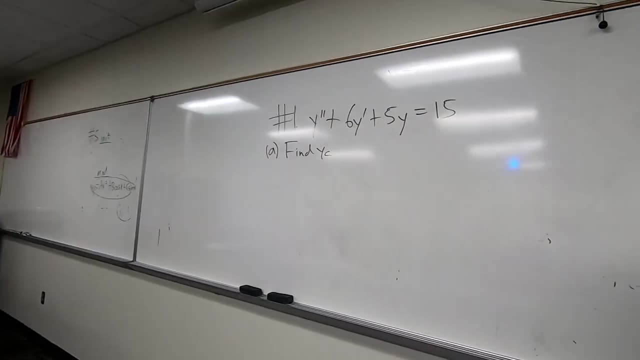 So part A on your test will say: find yc. Usually they're between five and eight points each. It just depends on the test. It depends how many points, How many points I lose before a test. No, I'm kidding, 15 points each. 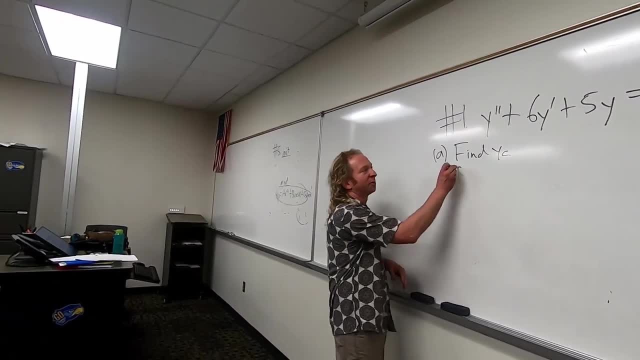 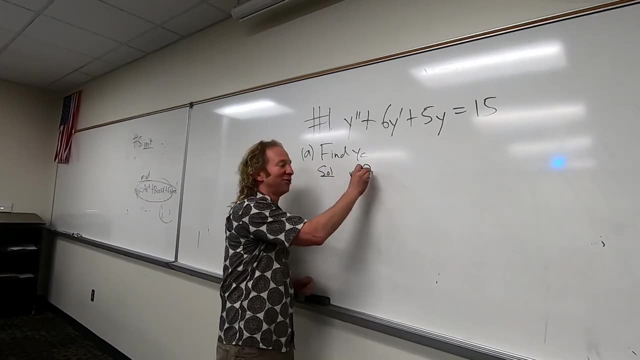 So find yc. That's called the complementary function or solution. All right, so solution. So you define the auxiliary equation. Remember that So m m squared, Or complementary m squared, Complementary, It's like plus 6m. 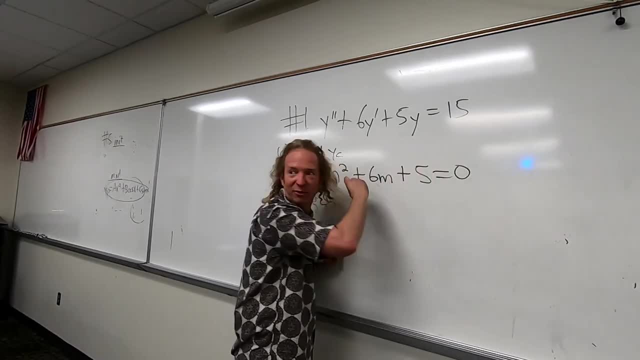 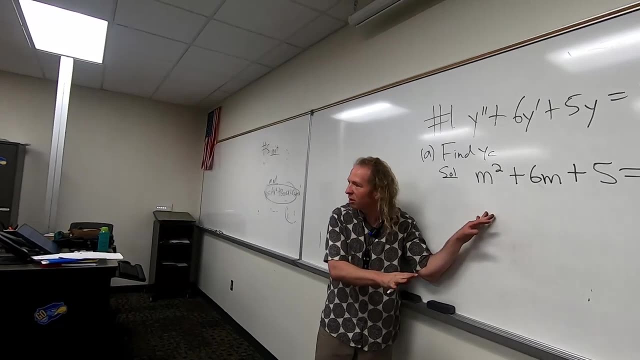 Plus 5.. Plus 5. Equals zero. So that's step one. We've got to solve this. These are all really easy in this section too. They're never hard. You're never going to have to use Rational roots theorem. 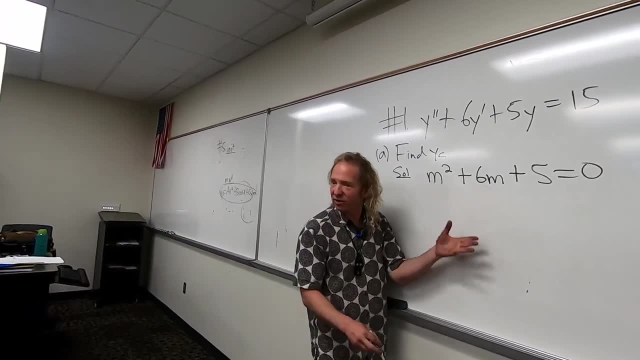 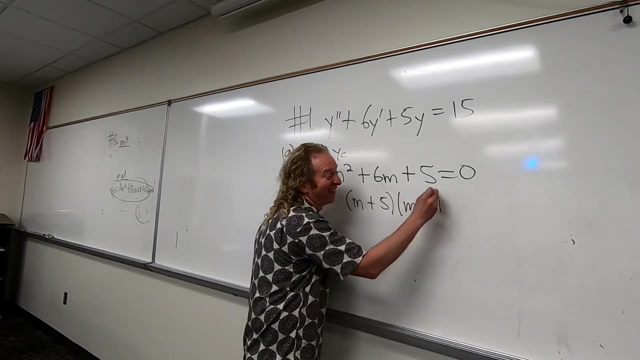 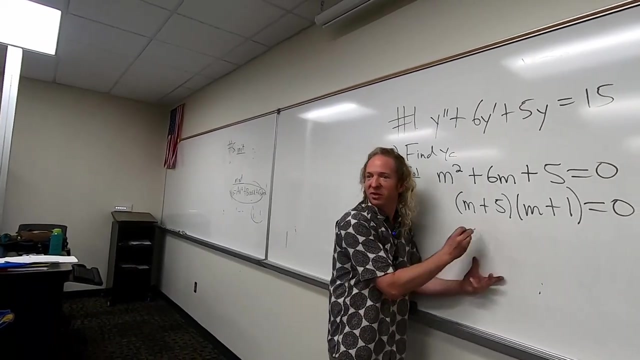 It's never going to be like. It's always really easy. So this should factor Most of the time it does in this section. That's happened to me before on tests and other people. So we're here, So we get negative 5 and negative 1.. 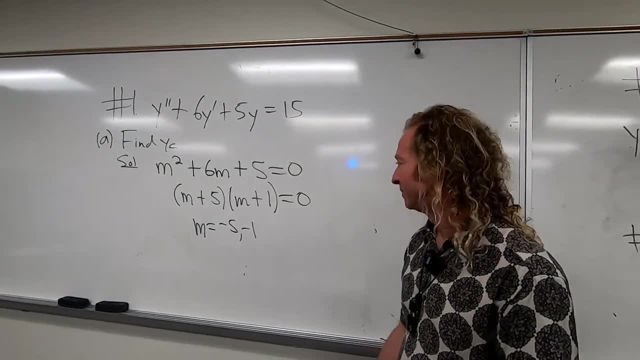 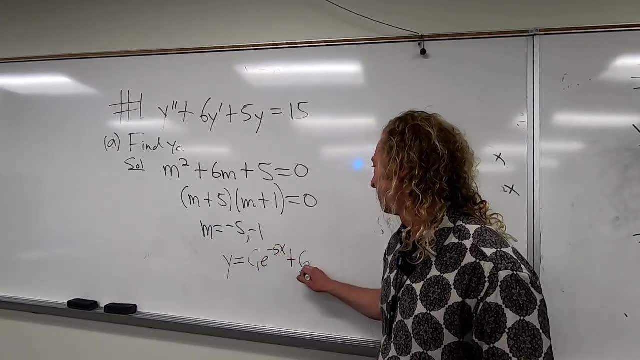 You're right, It doesn't. 2 and 3 doesn't work. It doesn't work. I just missed something, Me too. So c1. That's it. That's it. That's part A, That's yc. 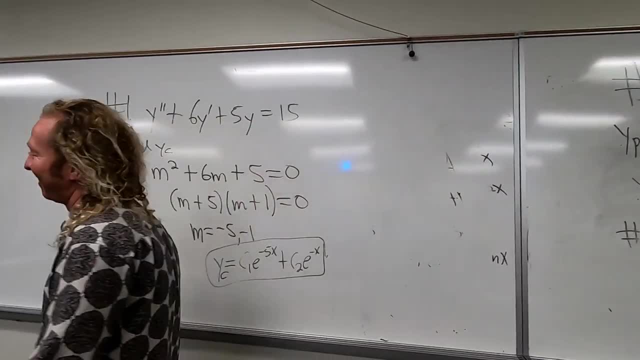 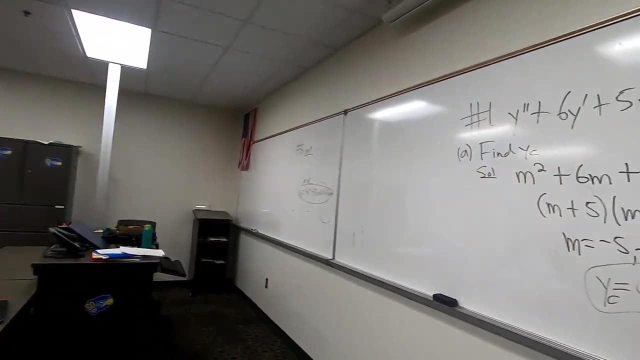 Yeah, that's yc, I'll just do every one. It's fine. That's fine. Yeah, Sharing is caring, right? Yeah, it's all right. It's all right. It's all right, Might need it, All right. 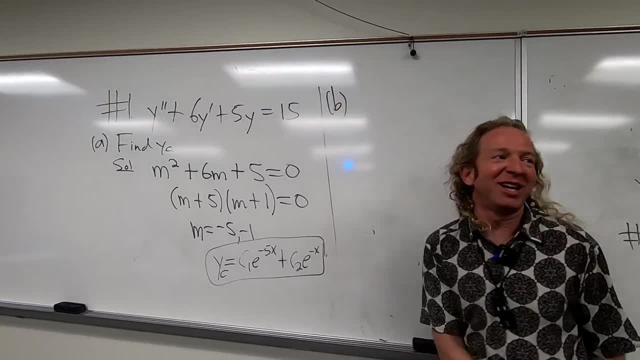 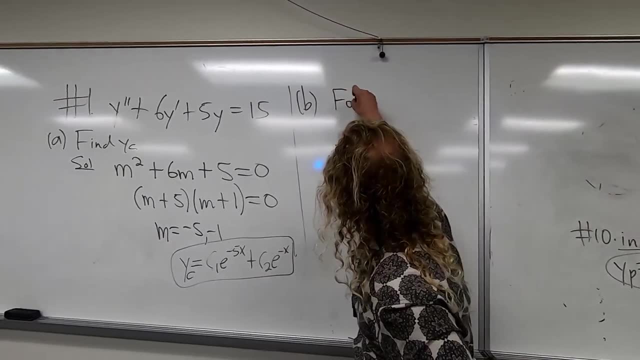 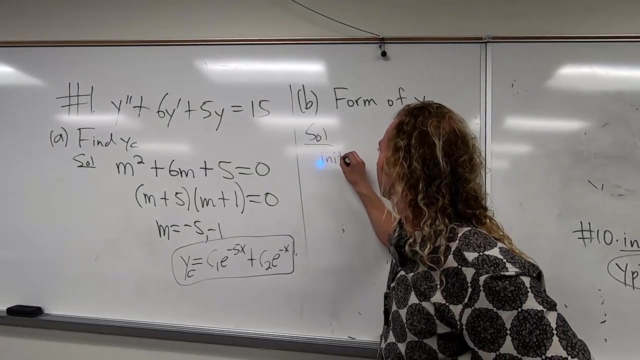 That's part A, Part B, Part B, Part B: Find the form of yp. This is what we just did. This is what we just did, So form, So find the form of yp. It's really easy, It's just A. 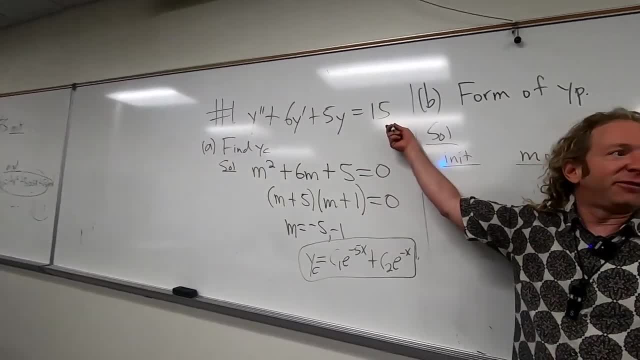 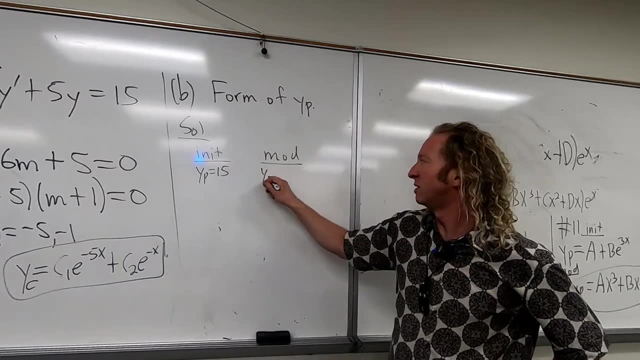 It's just A. Yeah, because you look at the 15, right And it's just A And it doesn't repeat. So I'm going to write it again, just to be silly. Sometimes it's good to be silly. Part C is also A. 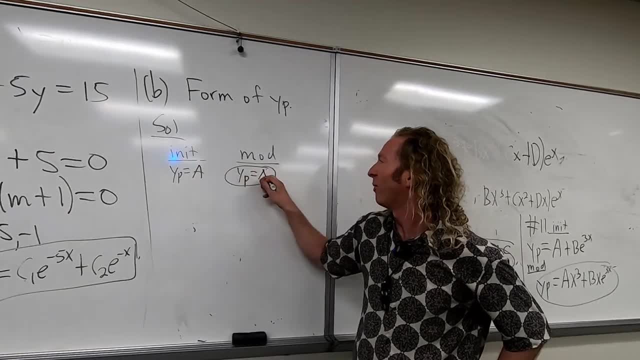 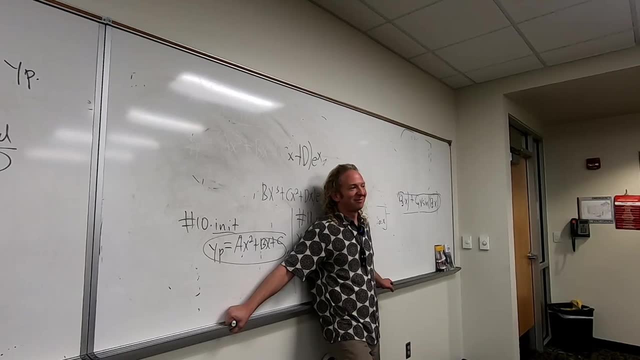 Oh, not 15.. It's A Wow, Wow, Wow, Wow, Wow, Wow, A A A. The camera got me. It's like Australians say A Or no good, A Good A mate. 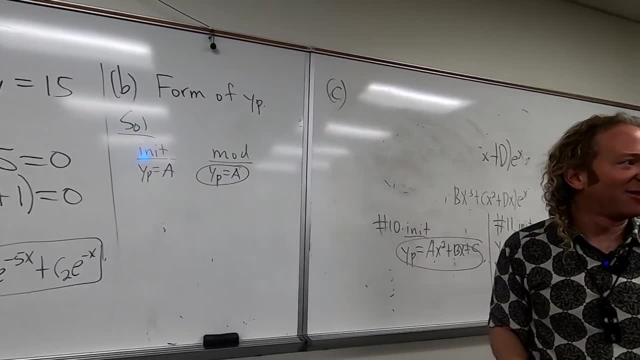 C, Good eye mate C, And so because that doesn't put no, There's no, Right, There's no. You look at that, You write this down. Then you look There's no constants here. Right, If there was like a C3 here. 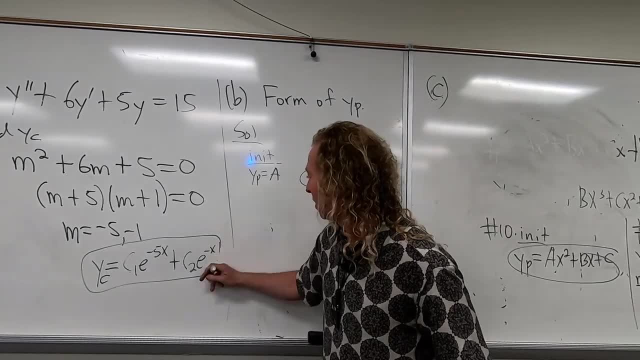 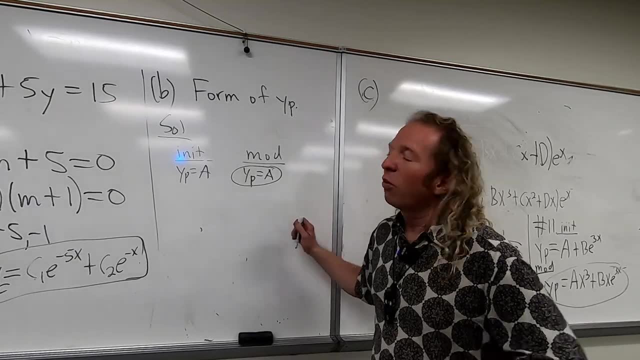 then you got to put an A Next year. Wasn't that C already? Huh, Modification, It's the same. I just wrote it twice. just to write it twice. No, I just mean step C, That's step three in the steps I gave you. 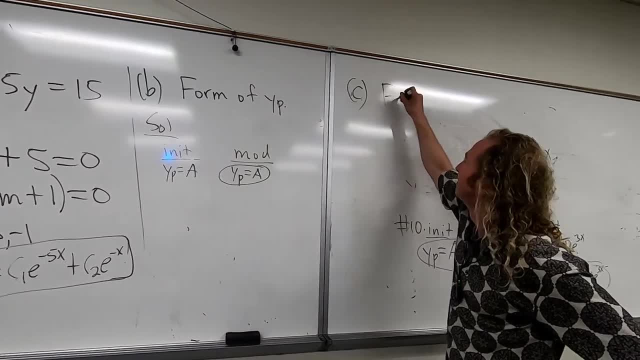 But that's. This is part C. now, Yeah, don't worry, This is. I thought you were dividing it in the same amount of steps that you did in the No, no, no, no, no, no, no. 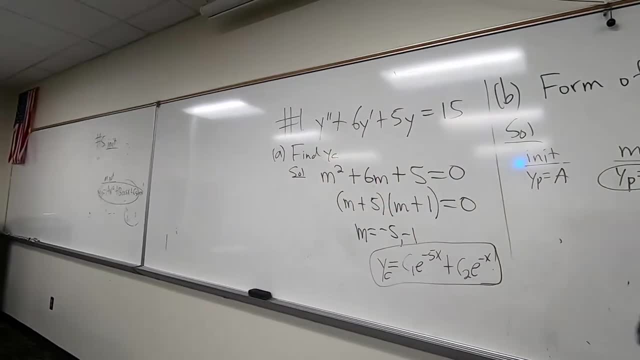 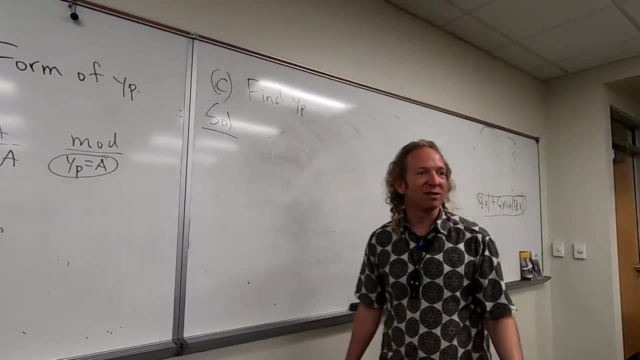 Oh, okay, We haven't done this yet. This is the new thing, So this is where it gets messy. However, this is the easiest problem in the history of the world, So this one will not be messy. So, Because we only have five minutes, 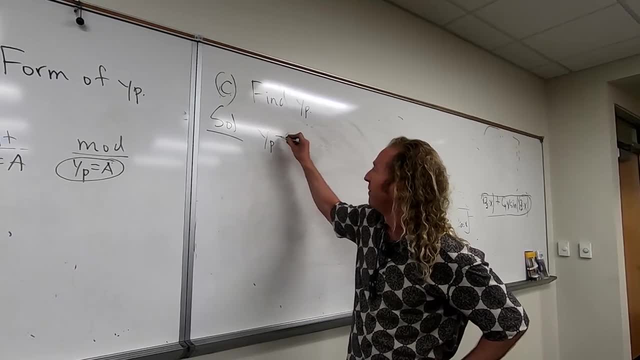 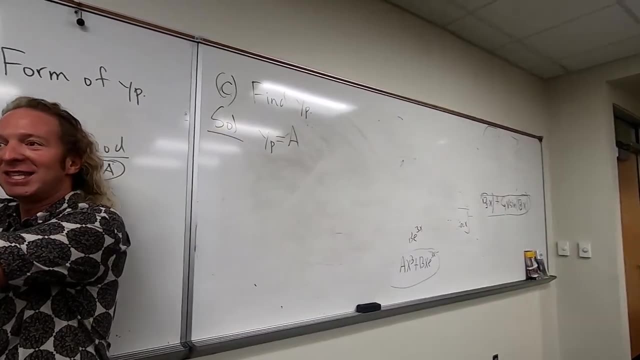 So basically, you have to write down your YP, So YP equals A, And now you have to differentiate this monster and plug it into this DE. So there's two derivatives. So let's take the derivative twice. So what is the derivative of YP? 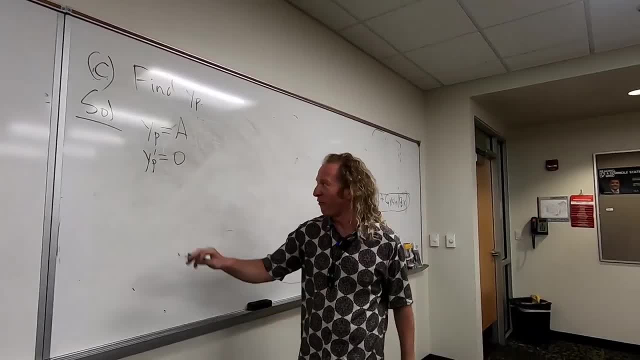 Zero, Then we have to do it again. I'm going to show every step, because this is our only example today. Next time we'll do a harder one, We'll jump in like: do the hardest one in the homework. This is zero. 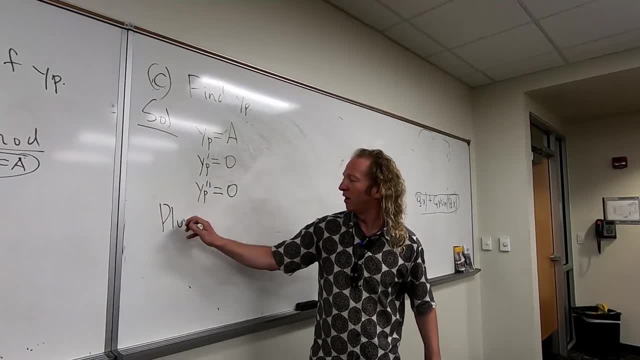 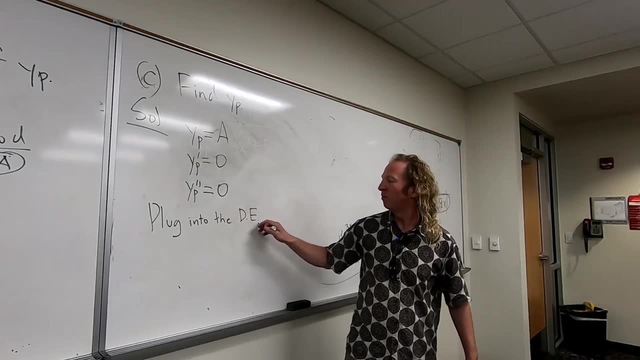 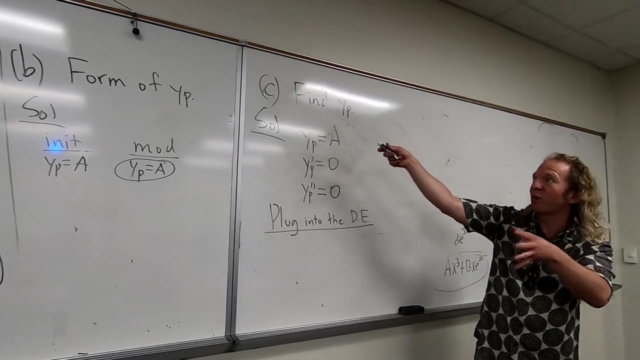 So now we plug into the DE, Plug into the DE, So always This is the same step. It's part C. Part C of the question is to find YP, So we have to find A. So basically you take the derivatives. 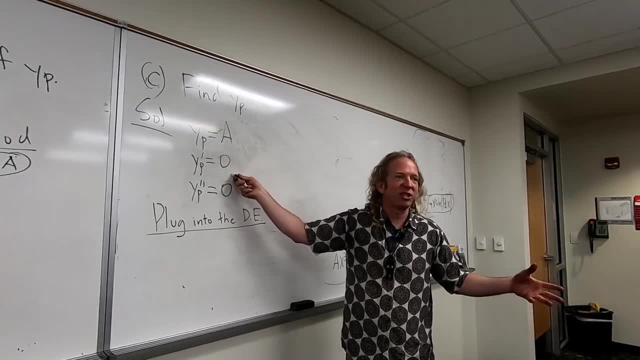 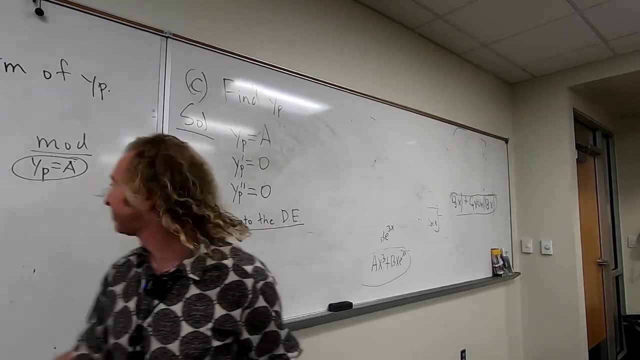 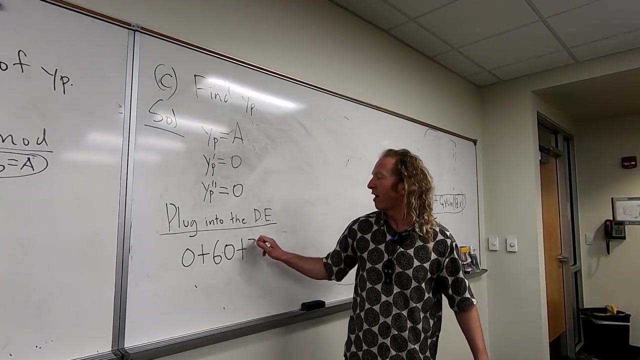 This is where it gets messy, because you know what happens when you differentiate right Product rule like six times. It's ridiculous So now. so it'll be zero plus six times zero plus five times A. Everyone see why it's A. 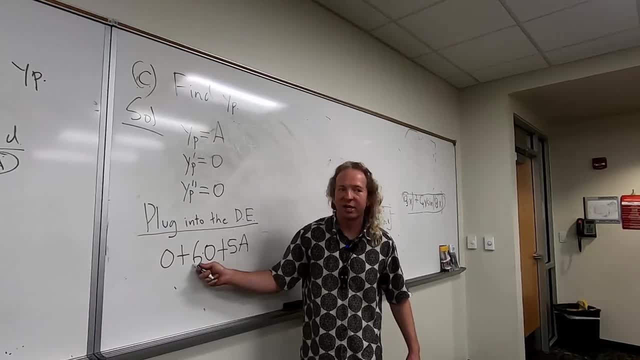 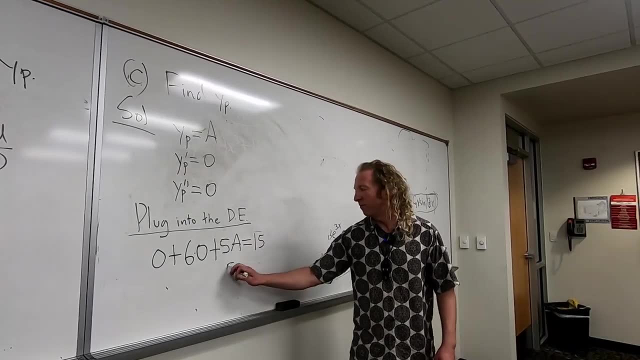 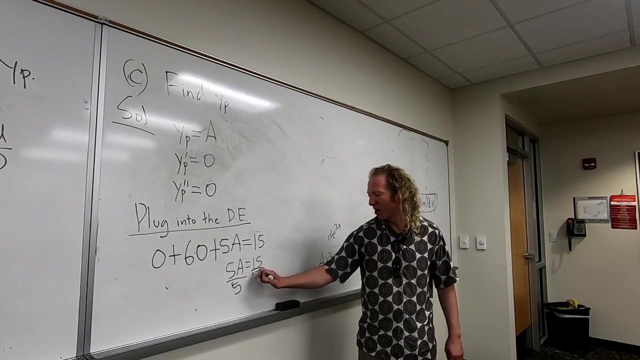 Because it's Y. So it's zero plus six times zero plus five times A, And all of that is equal to Fifteen. Fifteen, So divide by five. I'll show every step because we have four minutes, So let's like make it count. 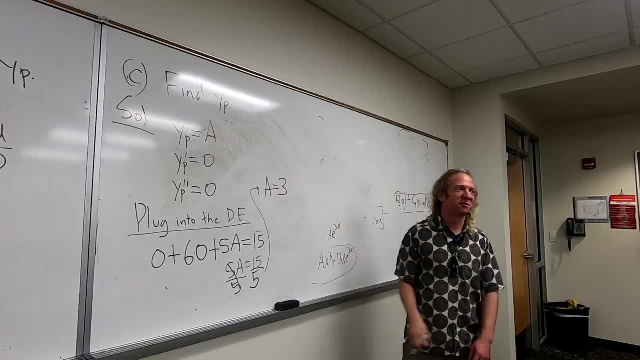 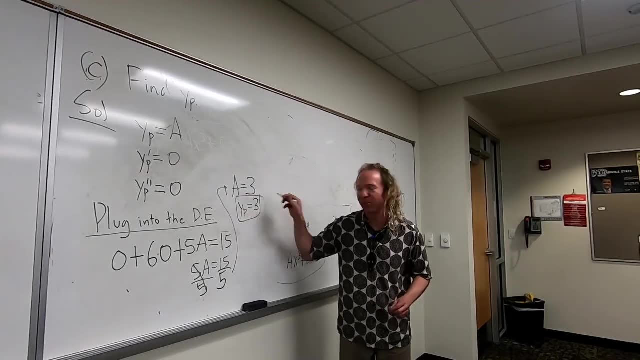 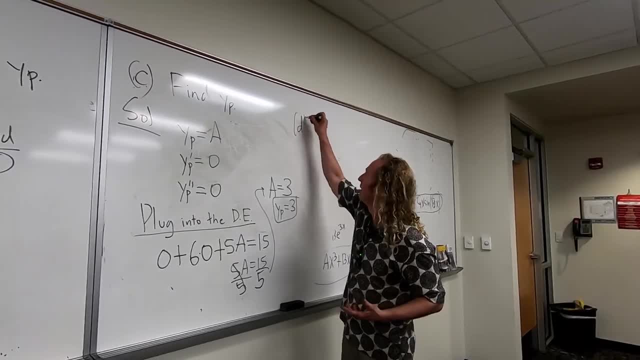 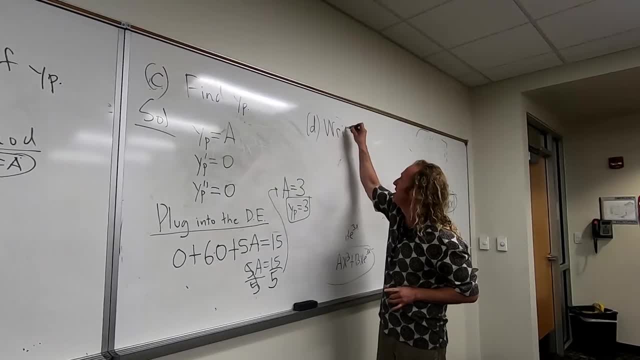 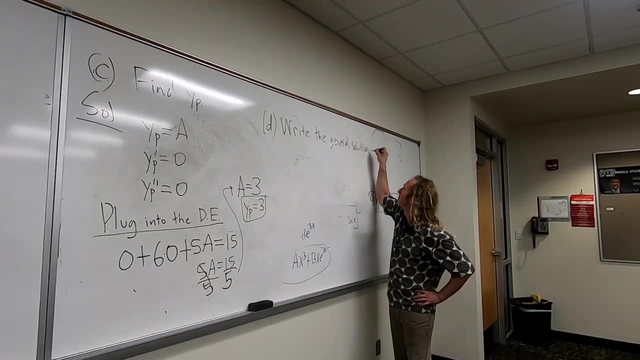 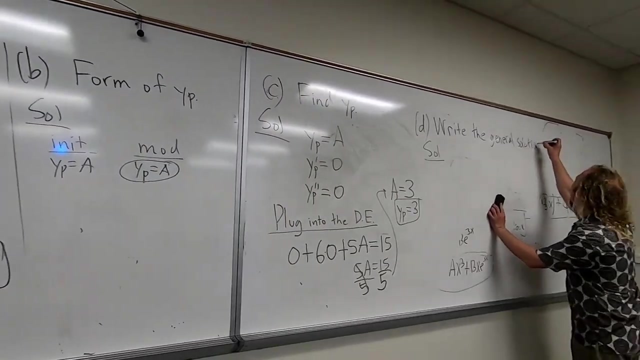 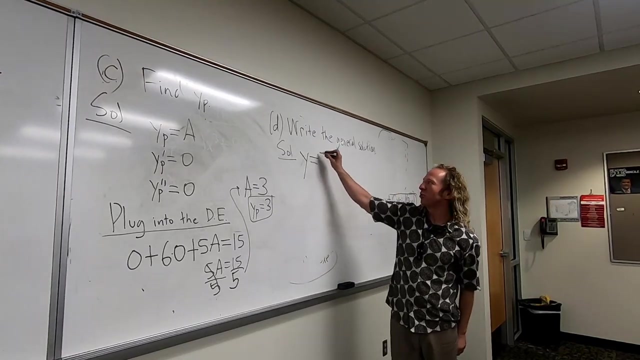 you need a break sometimes, Right, This is the easiest part if you have the answers already. The general solution Solution Solution. Sean. Write the general solution Solution. So the general solution is Y equals YC. Do you remember? 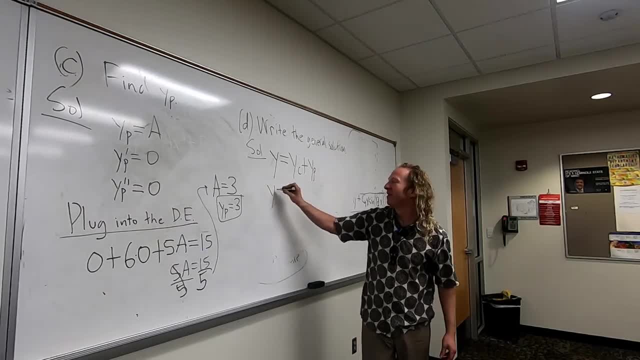 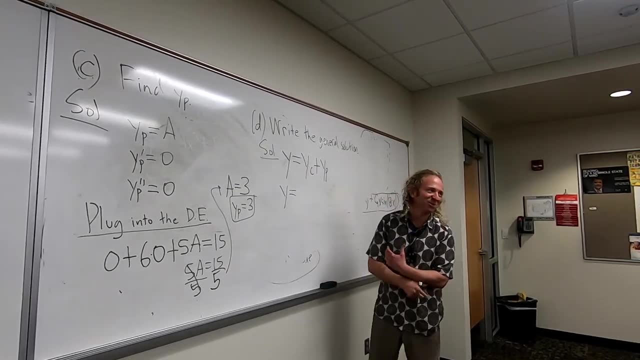 Plus YP. Sometimes people will like mess up and they just write this on the test. What happens if you do that? I don't know. I don't know. I don't want to make that decision now. It's really, it's really. 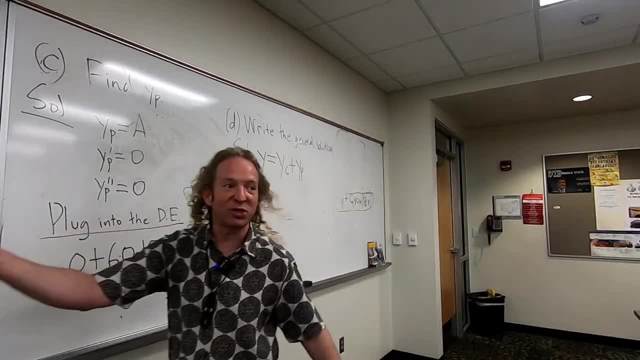 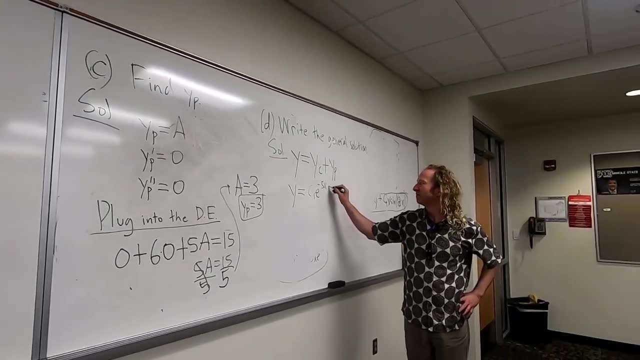 Don't do that. Please just get it right. Just get 100.. Please get 100.. So it's this one C1.. Mm-hmm, Mm-hmm, That's where I get three Plus Three. 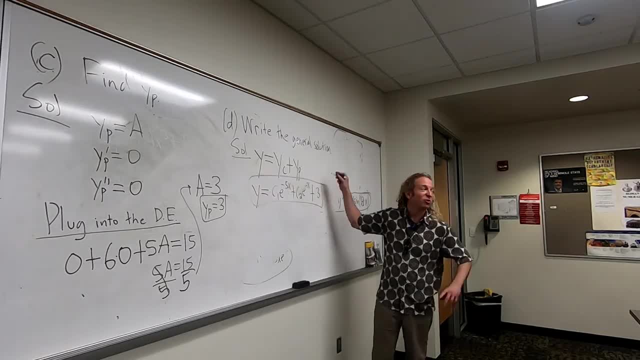 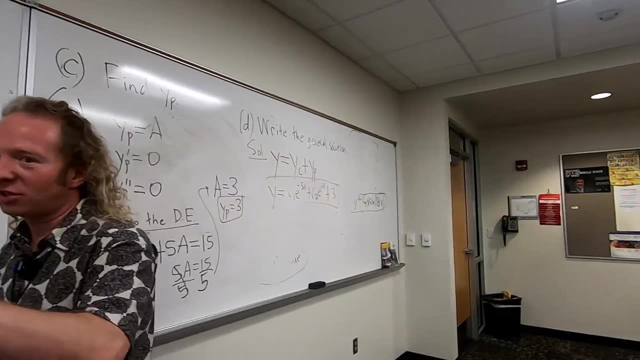 Three, And that would be the answer to the question. So this is what the homework wants. The homework will just say: solve, And you have to do all of this on your own. Do you have it in parts or just the final answer?